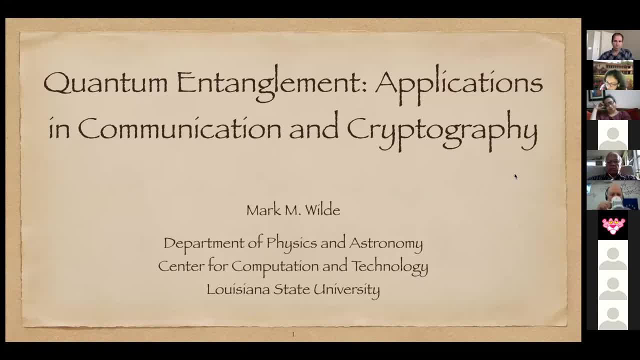 and the new journal of physics. His current research interests are in quantum Shannon theory, quantum optical communication, quantum computational complexity theory And quantum error correction, among many other things. So, without much further ado, I the floor is yours, Mark. Quantum entanglement: applications in communication and cryptography. All right, 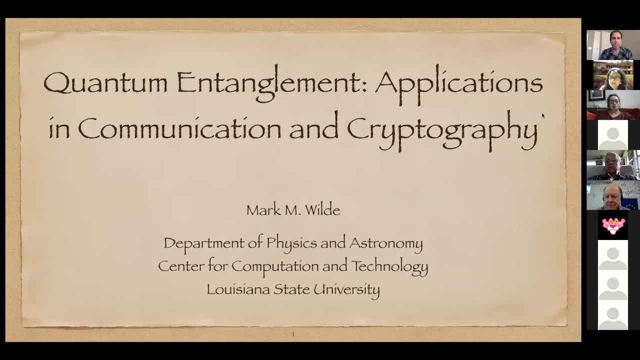 thanks a lot for the introduction. It's very nice of you and thanks for having me here. It's a pleasure to deliver this talk to such an esteemed group. Is there any chance that I could not? I could be a parasite instead of a co-host, Because what keeps happening is that I hide the floating media. 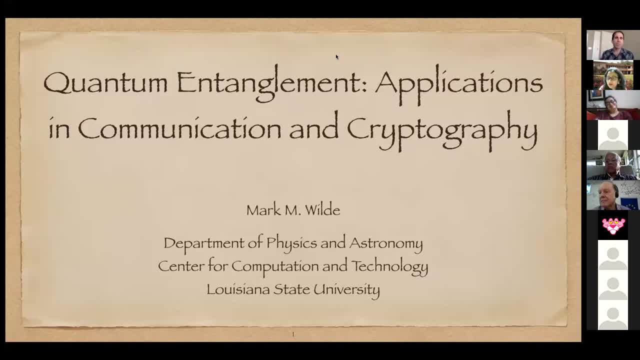 controls and then people keep coming to the waiting room. I can unco-host you if I. I don't think you'll ever become parasite, but I will withdraw the co-host permission. Okay, so then you're a normal participant. Okay, fair enough, All right, thanks a lot. Yeah, so it's a pleasure. 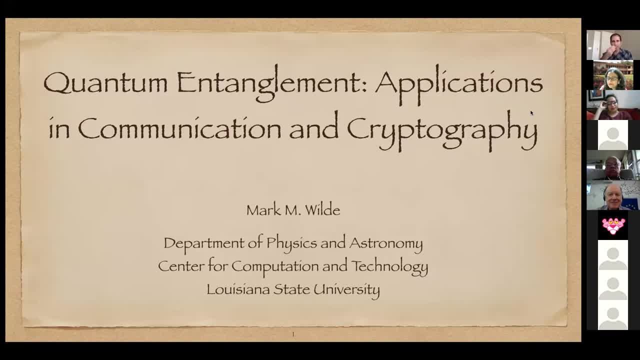 to be here and seeing so many people log in, I guess I got a little nervous, So I'll try to do my best. So there's a number of topics included. Some of them are basic and some of them are more advanced, And I'll try to find some balance between them. 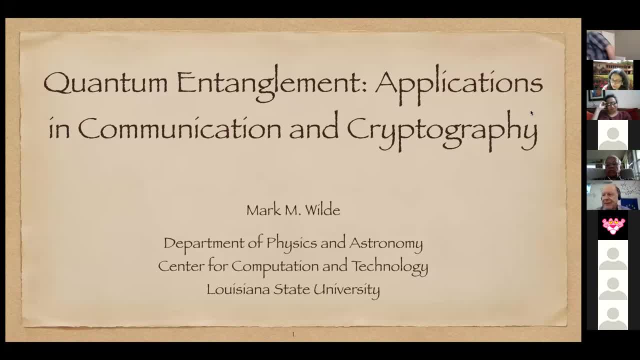 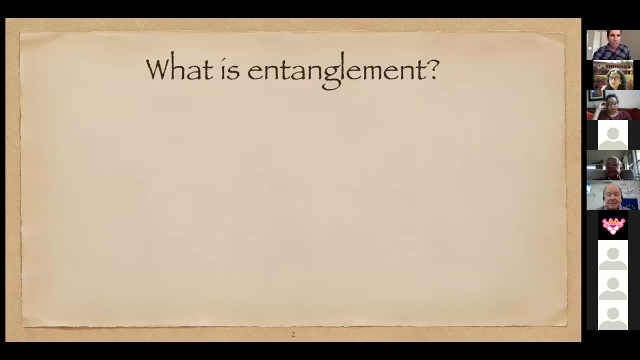 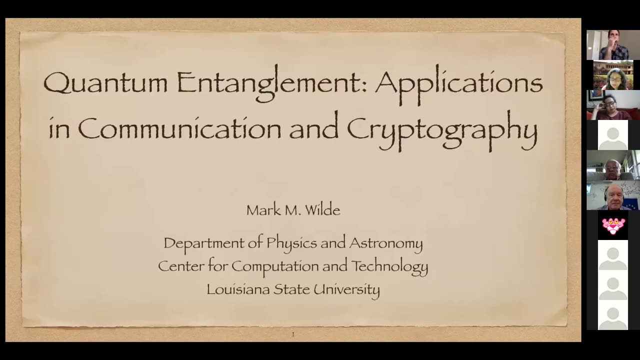 Please keep me on time. Maybe I'll grab my cell phone real quick to watch the time, if you don't mind. Okay, so yeah, this is meant to be some overview of applications of entanglement in quantum shannon theory, or maybe something i'll mention briefly. 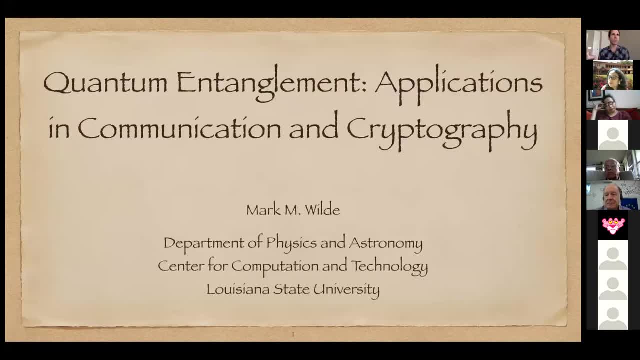 you talked about the ahp burkhauser prize. it turns out that this morning my co-author, david suiter's delivering the talk about that work at the international congress on math for mathematical physics and um. he sent me the slides one hour before the talk, so i hope it went well, okay, um. 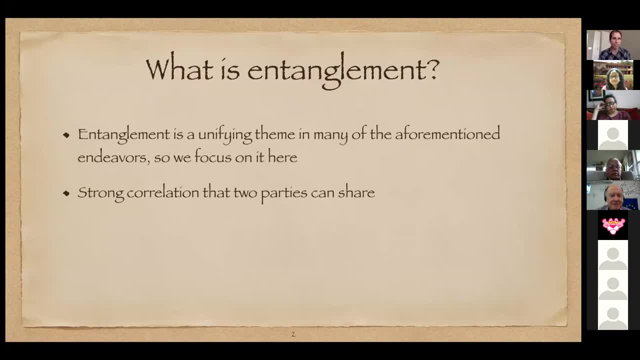 so entanglement, as we know is, is a unifying theme um in in quantum information and quantum communication, and it's a strong correlation that two parties can share, and it's it's really, you know, in quantum information, what we look for are distinctions or separations between the. 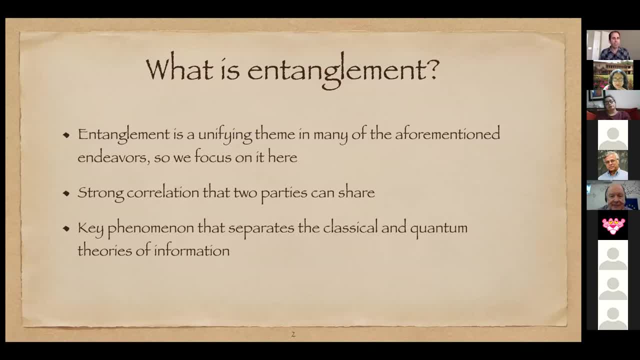 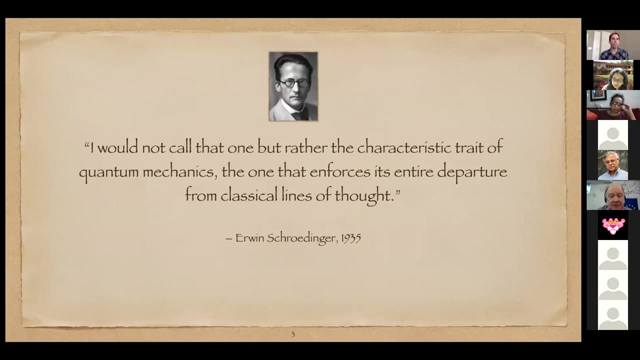 classical and quantum theories of information and it's typically the case that you find that in entanglement, you know, they're just things that are possible with entanglement, um, that are not possible in classical information theory. okay, and then you know, i guess this is for the younger people, um, this is a very famous quote of 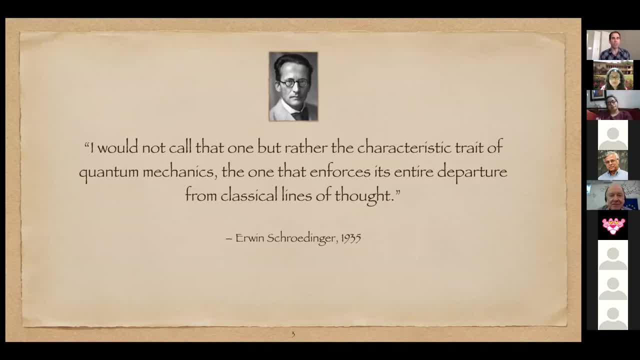 schrodinger. uh, i would not call that one, but rather the characteristic trait of quantum mechanics, the one that enforces its entire departure from classical lines of thought. so it's consistent with what we're talking about. you know, this entanglement is a key separation between: 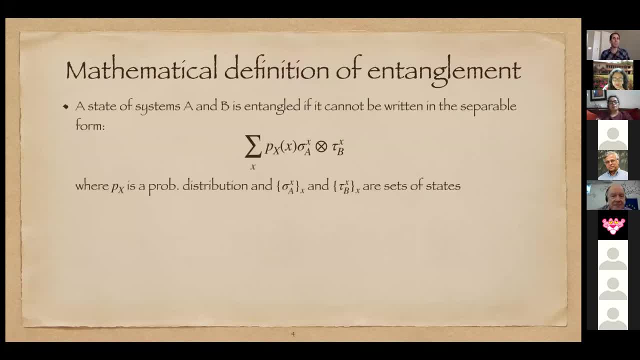 classical and quantum. so what is entanglement? um it, you know it can deal with, uh, states of two parties. uh, typically we call them alice and bob. it can also be for multiple parties, but throughout the talk we'll focus, uh, for the most part, on two parties. so we define entanglement mathematically in terms of: 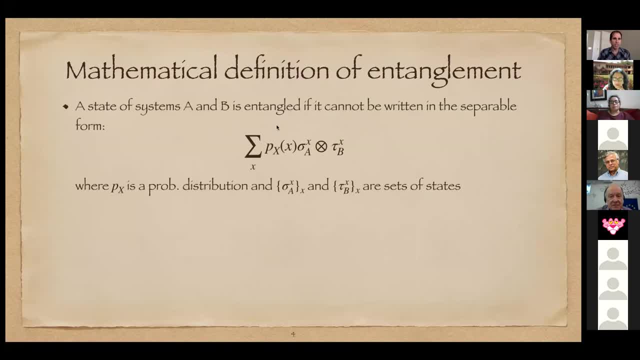 what it is not. and um, a separable state is one that can be written in this form, so it's a probabilistic mixture of two parties, and a separable state is one that can be written in this form. that can be written in this form, so we can do that by using certain types of curves of ah, of product states. 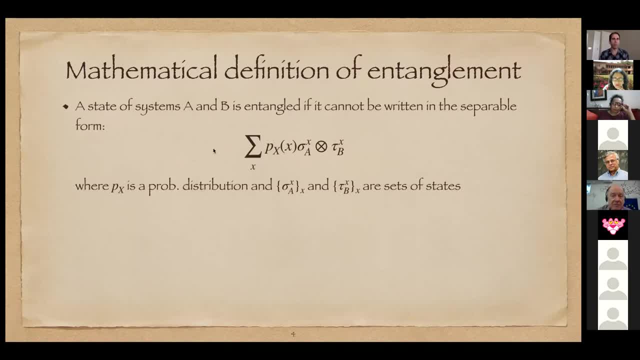 so we imagine that there's a hidden party in the backgrounds who generates this hidden classical variable x according to a probability distribution p of x, and then sends the the classical information to both alice and bob and um, you know, because that i not information is classical. it can be copied and sent to alice i Er DR bless you. robust and to be give us that�� okay, and so then they receive it. and then alice prepares a- moments, as we see it, toachteca and error at the producer, and then it's the first step to exactly get a transfer here, the food culture up. the the first step improves the original E. 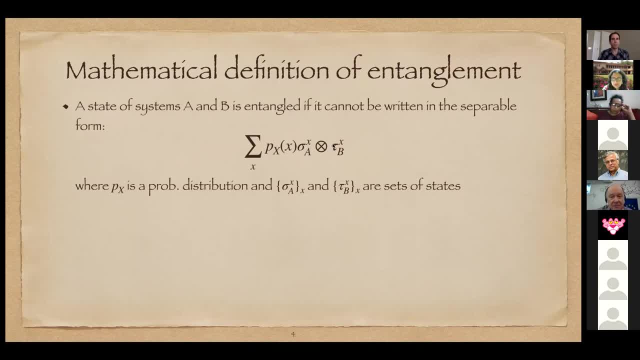 United S e sigma x, based on the value that she receives, and Bob prepares a state, tau x, and so this state is prepared by local operations and classical communication, and so it's unentangled. and then any state that cannot be written in this form is said to be entangled. maybe a few remarks. 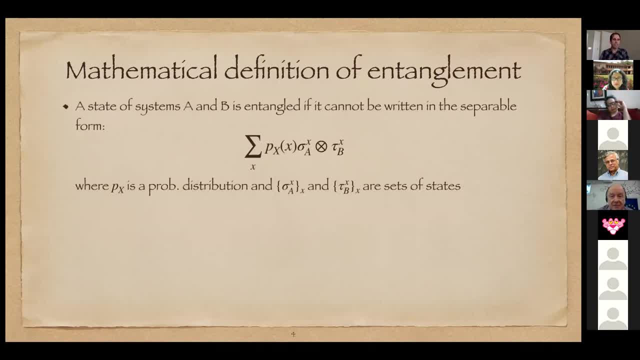 it is. it is a computationally difficult problem to decide if a state is entangled, and there's various ways that you can formulate this problem. one is in terms of the density matrix. so you're given the list of entries of a density matrix and if you're asked to decide if the state is, 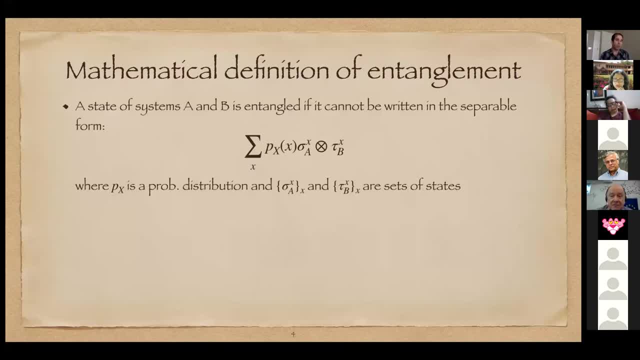 entangled. it's known that that is an NP hard problem, which means, according to widely held beliefs, that there's not going to be an efficient classical algorithm to decide that there. there are generalizations of that result where, if a quantum state is prepared by a circuit and then you want to try to decide using a quantum computer whether a state is, 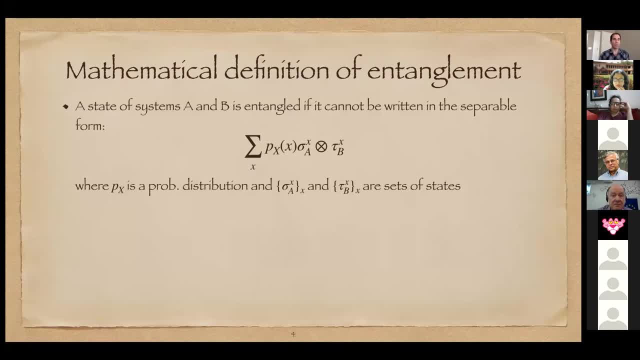 entangled. it's also believed that that problem is is hard for quantum computers to decide that problem. that's something that I've worked on, okay. so yes, as we're saying, separable states can be prepared by local operations and classical communication and, furthermore, like a basic 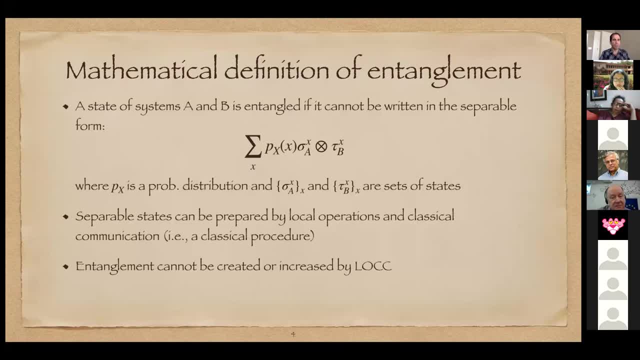 postulate that that you know, we we hold for entanglement is that if you have some state and you quantify its entanglement in terms of an entanglement measure, an entanglement cannot be increased by just doing local operations and classical communication. this, this resource theory of entanglement, was invented by Charlie Bennett. 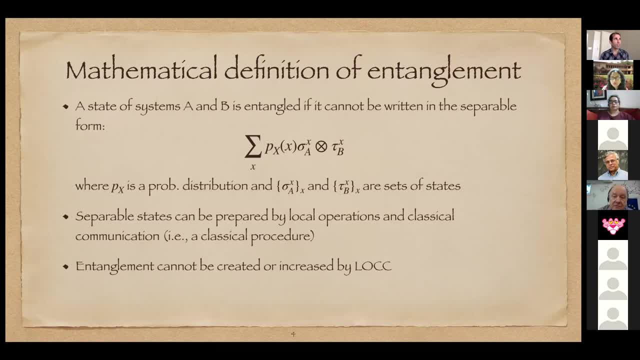 who's on the call? and John Smolin and DiVincenzo and Wooters, in a 1996 paper that has been widely influential, um and um, you know, even all these, all this theoretical work that we see on resource theories, um, that was influenced by this resource theory of entanglement as well. so, people in quantum, 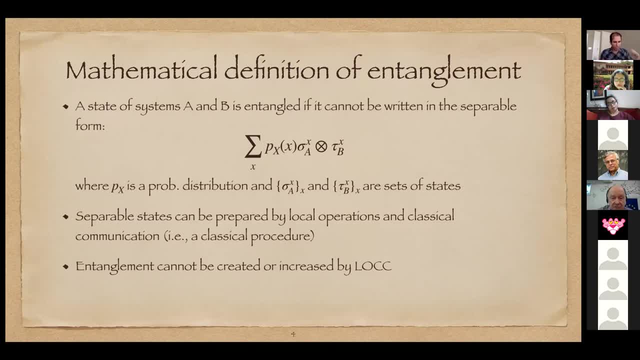 information. more broadly, they're now thinking about resource theories of almost everything. so there's resource theories of thermodynamics, there's uh resource theories of coherence- this, this, is a topic that has been debated quite a bit. there's resource theories of magic States for quantum computing. there's 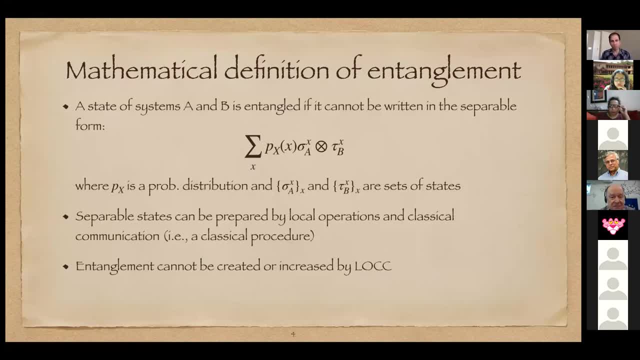 resource States of non-gaussianity, because in quantum optics experiments these non-gaussian States are typically a useful resource for quantum computing and uh communication. so, um yeah, those are just some comments I thought to make about uh general research topics that the younger people might be interested in pursuing. 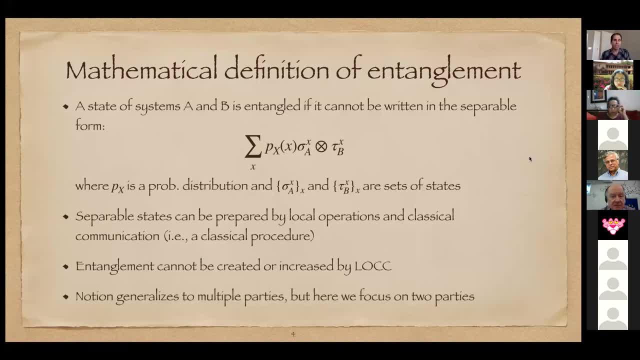 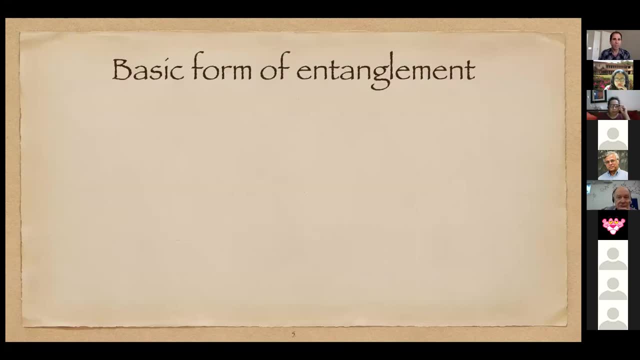 okay, um, and as I said, this notion of entanglement, it generalizes to multiple parties, but here we're going to focus on two. okay, so what is a basic form of entanglement is the ebit. this is like the standard fiducial form of entanglement and, as a density operator, it's written in this form. 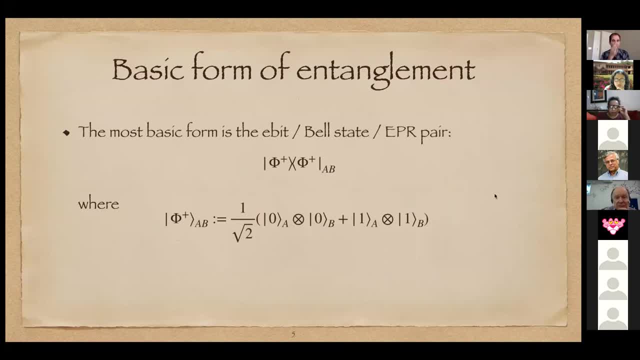 and this is the cat corresponding to the, the ebit state, and it's a uniform superposition of two possibilities. both Alice and Bob have zero zero, or they have one, one and um. it appears in many basic protocols such as teleportation or superhands coding, and so often we're trying to distill states. 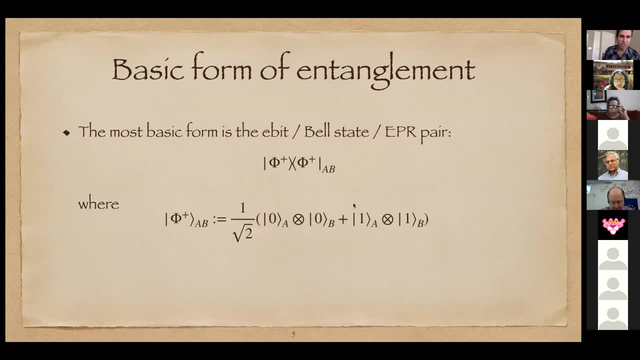 uh, to, to to this standard ebit state, or as many ebits as possible, okay. if you want to try to think of a classical analog of entanglement, I would say it would be a shared secret key. okay, so why? why do I say that? um, a shared secret key is private to Alice and Bob. it's uniformly random and perfectly correlated. 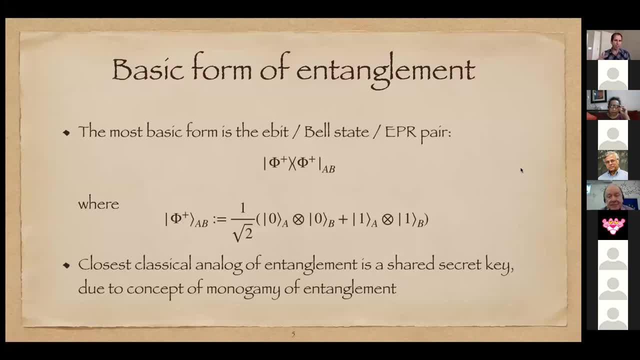 and a key aspect of it is it's intensive product or it's it's independent of any other uh uh system in the universe that some eavesdropper could possess. okay, and these kinds of properties are very similar to to those that entanglement has. 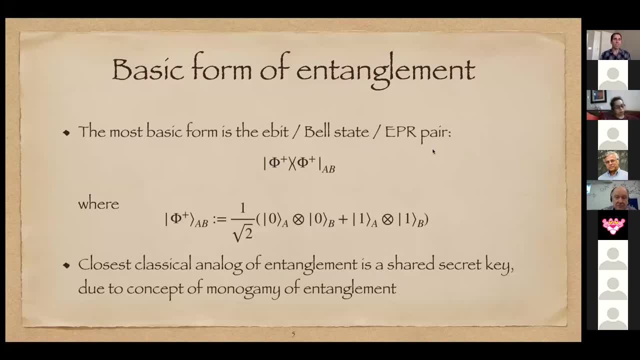 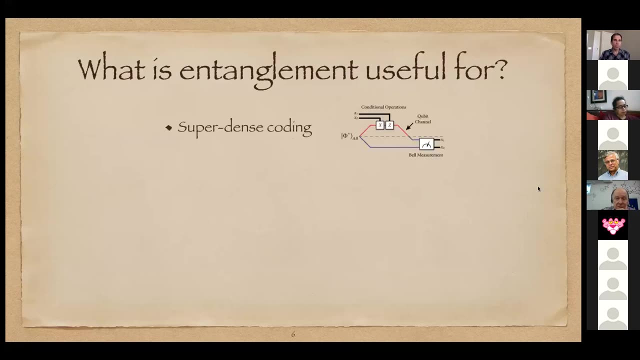 and in fact if you have a pure entangled state, then you can do local measurements on it to get a shared secret key. but you can't necessarily go the other way. if you have a shared secret key, you can't generate from that entanglement. okay, so, um, what is entanglement useful for? I'm 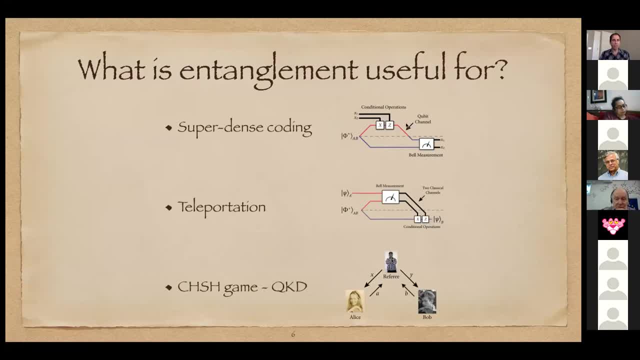 going to review these basic protocols. they're quite famous. and then what we do in quantum Shannon theory is we think of generalizations of these protocols. Like you can ask, oh, let's take the noiseless qubit channel and make it noisy. Then what happens? 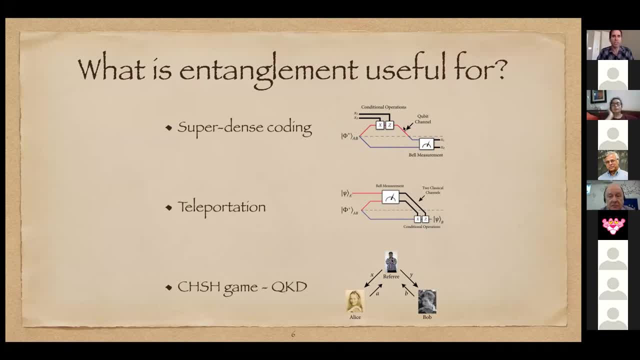 Let's take the ebit state, Let's make it a noisy ebit state. Then what can we do? right, And in teleportation you can make the shared entangled state noisy and then ask about what kind of transformations are possible and at what rate can you do transformations? 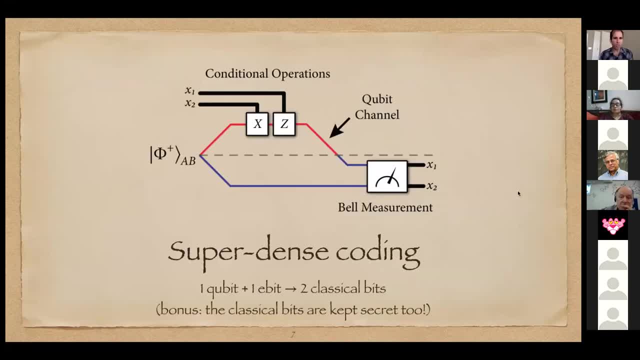 Okay, So superdense coding, very famous protocol introduced by Bennett and Wiesner in 1992.. The way that it works is: Alice and Bob share this ebit state before communication begins. The diagram indicates that the two qubits have been distributed to Alice and Bob. 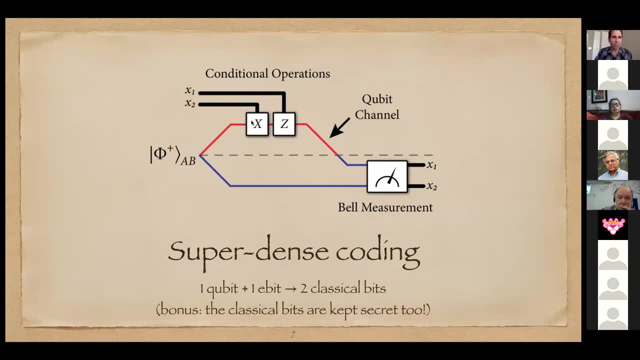 And then what's very interesting is that the two qubits have been distributed to Alice and Bob. And then what's very interesting is that the two qubits have been distributed to Alice and Bob And by performing local operations, Alice can rotate the global state to one of four different possibilities. 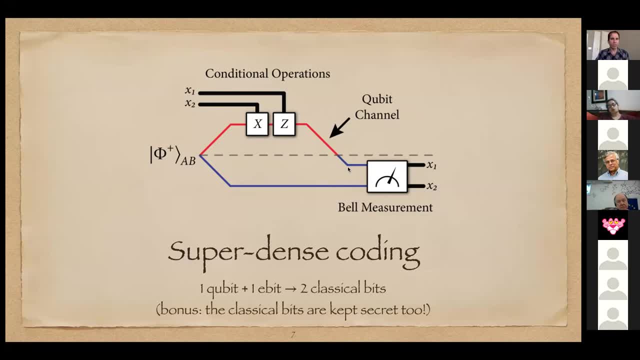 She'll then send her qubit over this noiseless qubit channel And then Bob can distinguish which one of the four possibilities. Alice rotated the state to Okay, And this is the perfect implementation of the protocol, And you know we can modify it to consider imperfect versions. 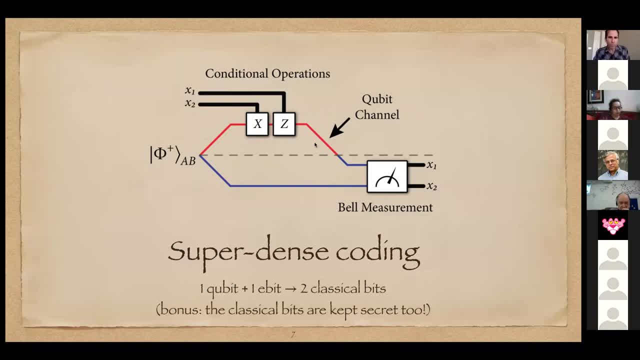 But for now let's focus on the perfect version. What's also an interesting aspect of the superdense protocol- superdense coding protocol- is that it has a security aspect whereby you know if there's an eavesdropper tampering the line. 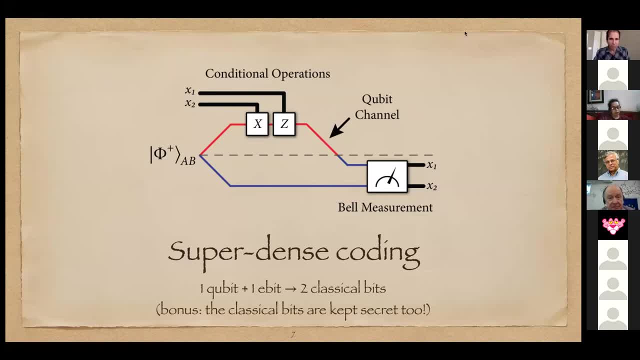 then, excuse me, sorry, if there's an eavesdropper tampering the line, then this eavesdropper only has access to this system And the state of this system is a maximally mixed state, independent of the bits that were encoded here. 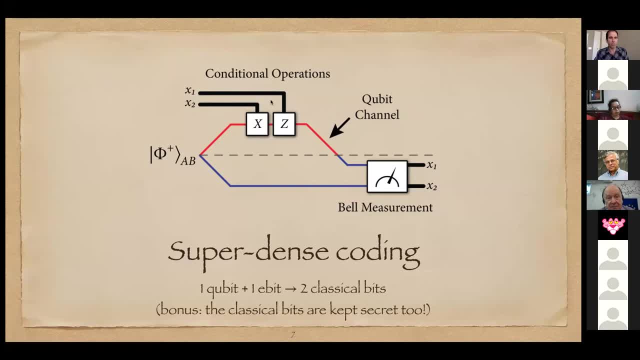 And so an eavesdropper tampering this line cannot figure out which bits were encoded, And that's sometimes considered in the context of secure communication. Okay, And then you know- this is another thing that Charlie Bennett introduced- is thinking of this protocol in terms of resources. 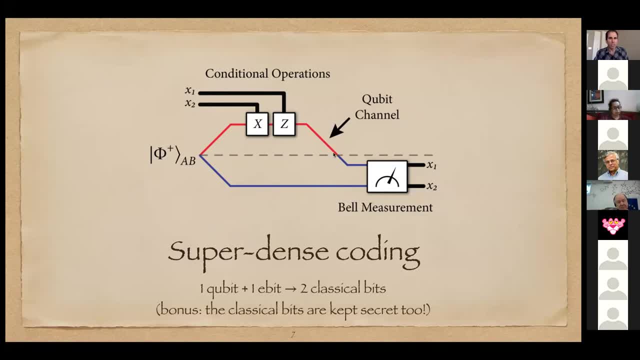 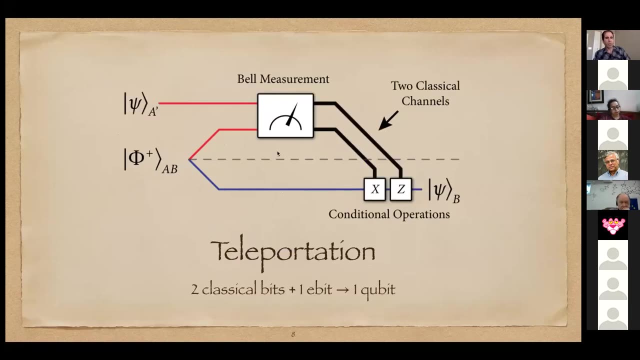 Resource conversion. So the protocol takes a qubit channel and an ebit and then it converts those non-local resources to the non-local resource of two classical bits being communicated. Okay, In teleportation what you do is you flip things around when compared to superdense coding. 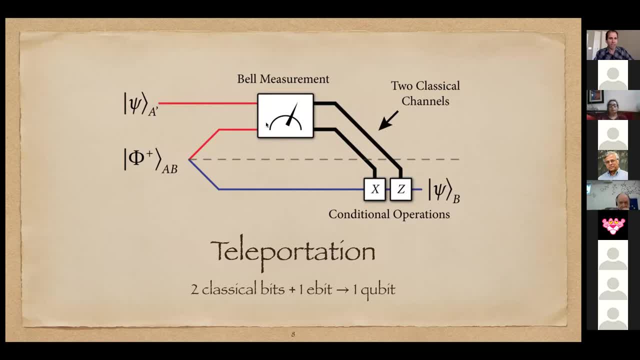 Instead of Bob performing the Bell measurements, Alice performs the Bell measurements And Bob does these conditional Pali operations. And this protocol was discovered one year after superdense coding. I have my hopes up that one day a Nobel Prize will be given for the teleportation protocol. 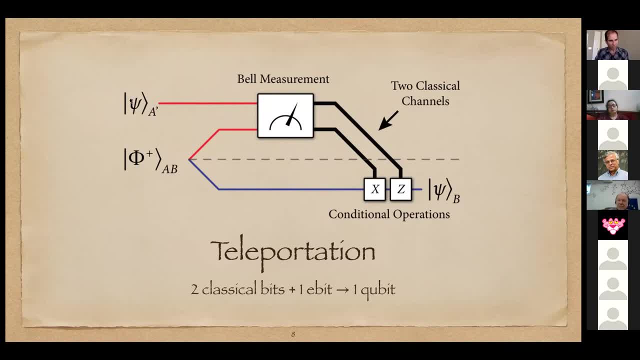 But we'll see. So what it does is it transfers a qubit faithfully from Alice to Bob. Okay, And it's. it's by means of this interaction between the Bell measurement and the entangled state, And you know, these two classical bits are transmitted. 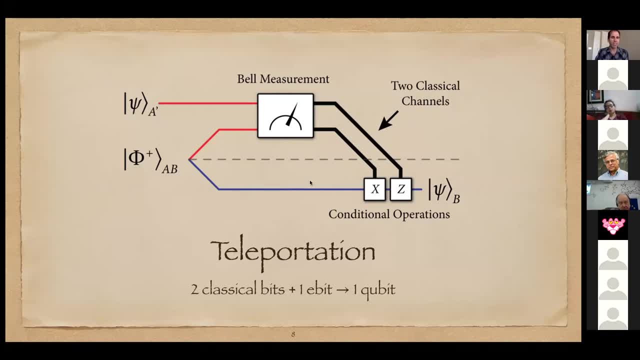 Before the bits are recovered by Bob, the state locally is in a maximum mixed state, And so the state, the local state of Bob, is useless before the classical bits are recovered. But then, after performing these conditional operations, Bob can recover the state that was transmitted. 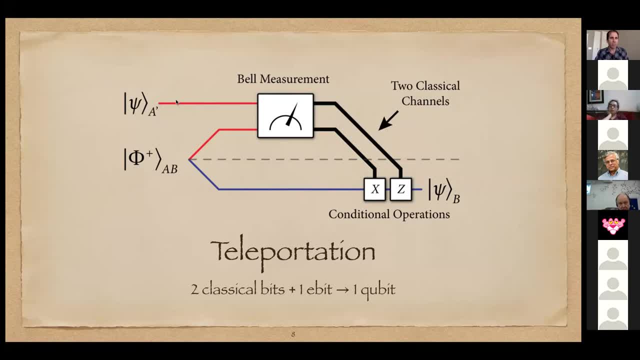 There's also no violation of the no-cloning theorem, because the state here gets- I believe the phrase in the original paper was the disembodied transport of the state from here to here. So the Bell measurement somehow disembodies the state and then it's encoded in these non-local correlations and then appears over here on Bob's end. 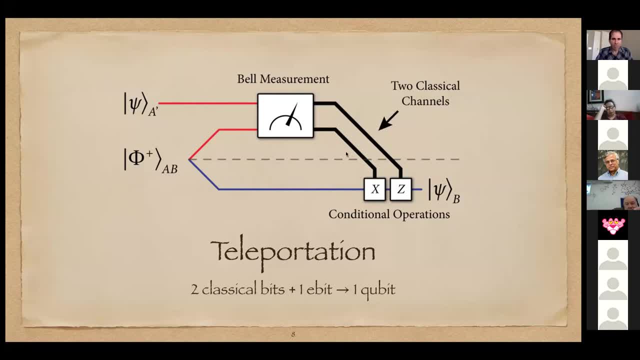 Okay, Again, there's a cryptographic aspect of this protocol. If someone has access only to these classical bits, then they cannot figure out anything about the state that that is is present here and that we want to teleport over here. These two classical bits are uniformly random and independent of the state here. 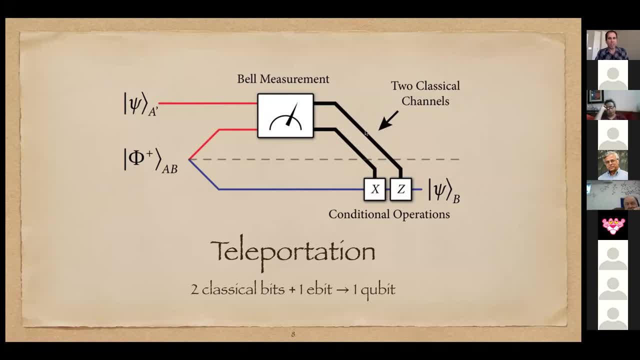 And so you know if an eavesdropper is tampering the line then she cannot figure out anything about the state that's being transmitted. I think that aspect has been utilized a fair amount And you know variations of quantum key distribution protocols such as like measurement device, independent QKD. 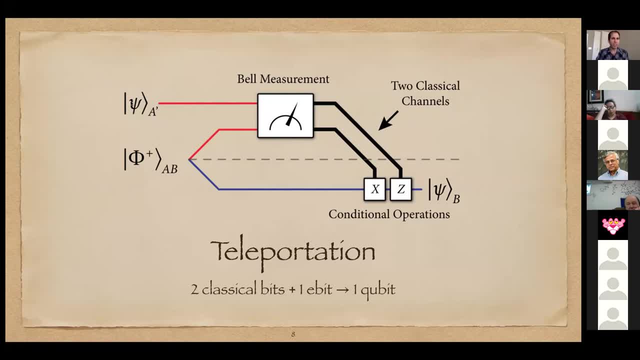 Okay, And then the transfer of the state works for any possible state. You know it's like a universal teleporter. So the protocol again, we can think of it in terms of resource conversion, where we take these two classical bits, one e-bit, and convert them to one qubit. 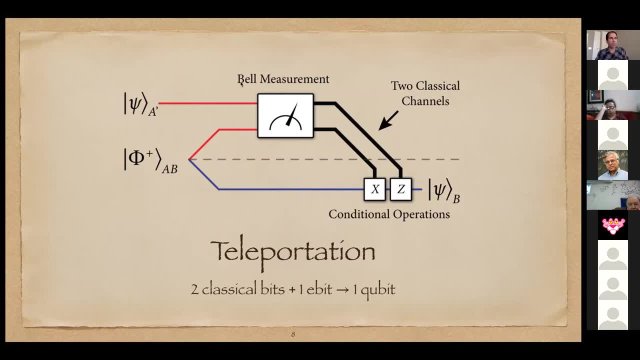 And it's interesting if you read some of the early papers on teleportation. Richard Josa had some exposition of teleportation and he said that you can think of teleportation kind of like the qubit goes back in time, like the qubit is here and then it somehow gets transferred and like ricocheted through this bell measurement and then ricocheted off of this bell state and appears over here. 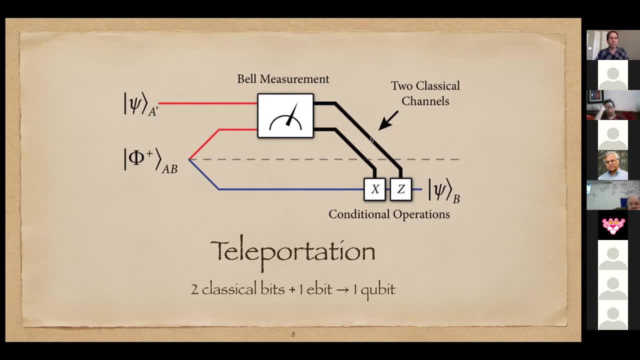 And so that's a very interesting way to think about it conceptually that in fact Charlie Bennett invented a model of time travel that has been considered seriously by people working on quantum gravity et cetera. that's called post-selected teleportation. 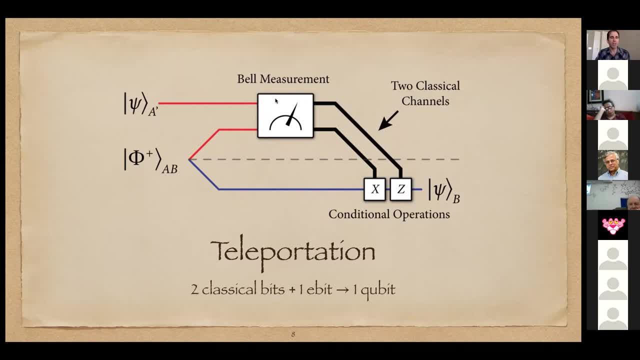 So the idea there is that one-fourth of the time you get lucky and there's no classical information that needs to be transmitted, And so it's kind of like the qubit Back in time. Okay, But I won't talk about that further today. 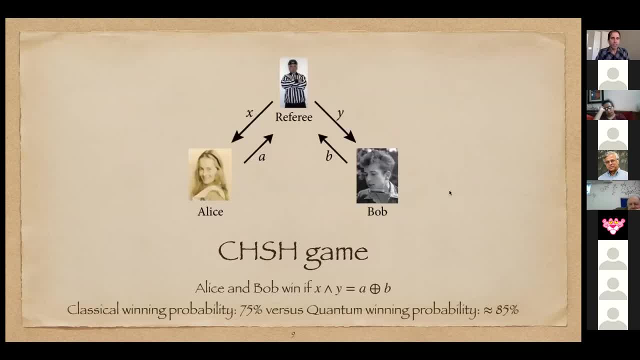 I just thought it was an interesting point to mention. Okay, Another way that entanglement manifests itself in quantum information is through the use of this CHSH game, which is another way to describe a Bell inequality experiment. Okay, And you know, we're now at the point where Bell inequality experiments, or CHSH games, have been demonstrated very convincingly. 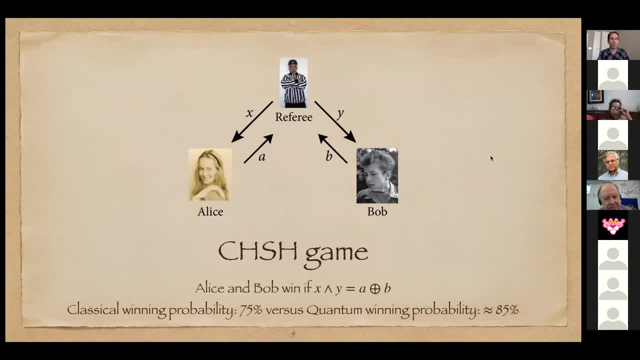 Experimentally, this happens. you know, there were early experiments in 1982 and later, but then it was about 2015,, 2016,, where various experimental groups closed loopholes that were associated with Bell inequalities. Okay, But what is the basic game? 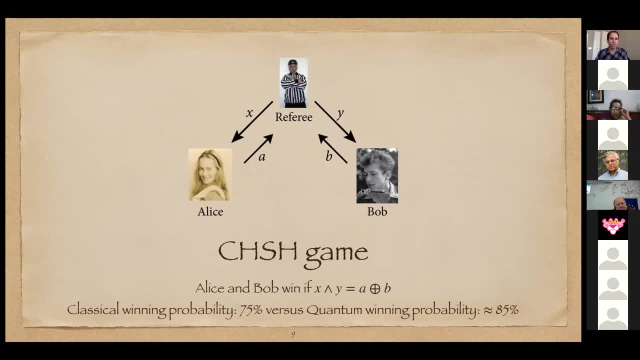 We imagine there's a referee in the background and then there are two players, Alice and Bob. The referee communicates a bit to Alice and another bit Y to Bob, And then Alice and Bob, they report back classical bits A and B. Okay, 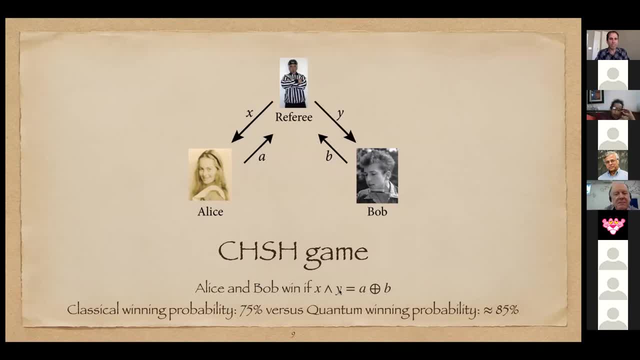 And then the referee declares that they win the game. if the logical AND of the inputs is equal to the exclusive OR of the outputs, Okay. And if they employ a classical strategy, in which you know they're not allowed to share entanglement, if they just have separable states or classical shared randomness? 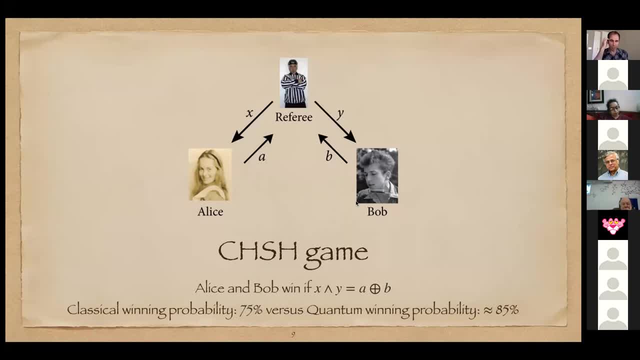 they can only win 75% of the time, Okay. But if they share this EBIT state and they're allowed to do non-commuting measurements locally, then they can win 85% of the time, Okay, Which I believe is equal to cosine squared pi over eight. 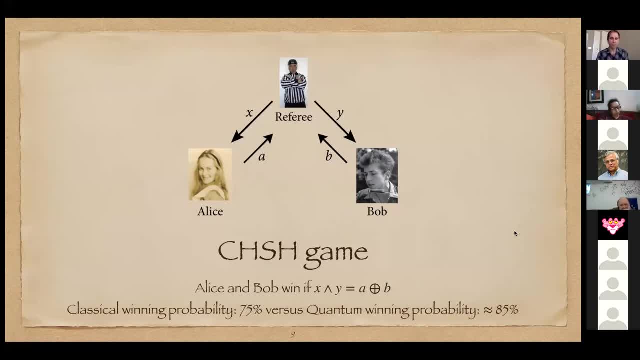 It's this famous number in quantum information. Okay, And the CHSH game is the basis for cryptographic protocols. Okay, With device-independent QKD, which has been investigated quite a bit over the past decade and more. So the idea there is that, you know, on some rounds of a QKD protocol you do tests with the CHSH game to test, to have some confidence that Alice and Bob threw by means of sharing quantum states and local operations and classical communication. 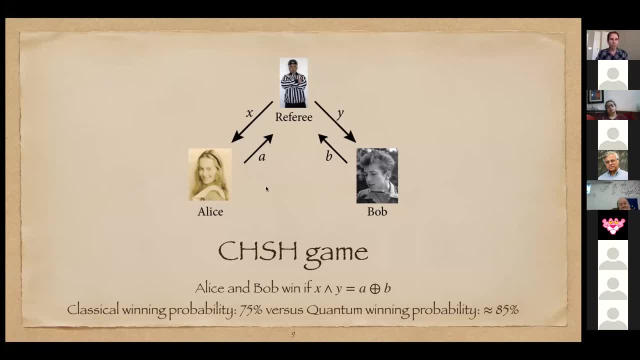 Okay, They can share some EBITs, And so on the test rounds, if they share EBITs they can win 85% of the time. And then the idea is that on the other active rounds, if they have EBITs, then they can generate secret key right by the argument they were making earlier that an entangled state is in tensor products with any eavesdropper. 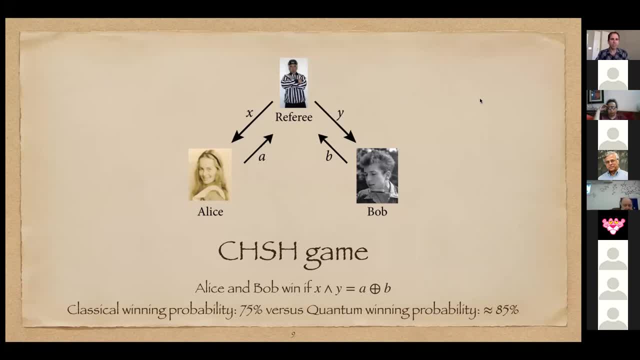 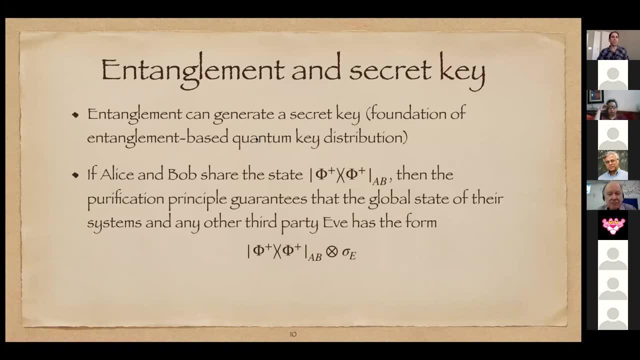 And then they can use these entangled states to generate secret key. Okay, So Indeed, let me talk a bit further about that and how entanglement can generate a secret key. If Alice and Bob shared this EBIT state, then there's a purification principle of quantum mechanics. 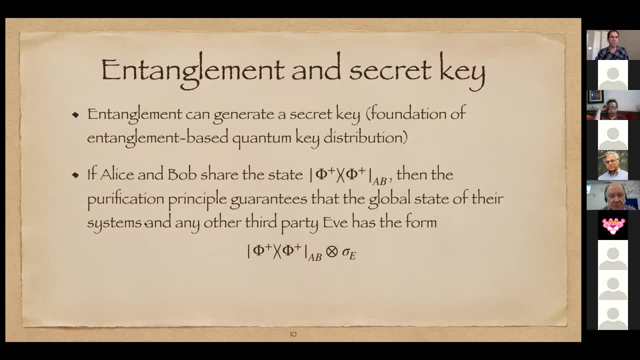 It guarantees that the only possible global state of their systems and any other third party has to be in this tensor product form right. So if they share this ideal state, then that is their state And the eavesdropper has no correlations whatsoever with this entangled state. 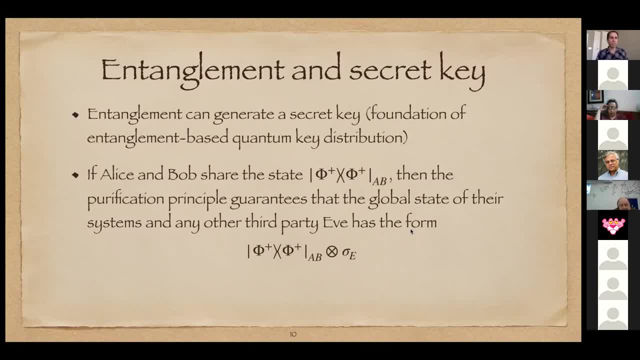 And so that's also called monogamy of entanglement, because it's only Alice and Bob that can be entangled, and not a third party, if they share this EBIT state, And so by doing these local measurements, they can distill a secret key. 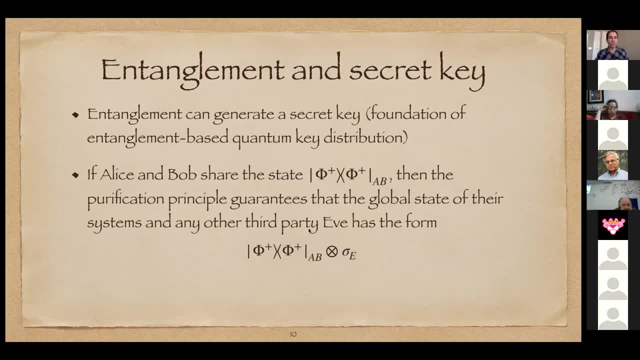 And then, whatever the eavesdropper measures, she'll not be able to figure out the outcome of the The measurements of Alice and Bob. She would just have to try to guess randomly what the outcome would be. And if they share many, many EBITs and they're doing this experiment over and over again, then the probability for the eavesdropper to guess the exact value of the secret key drops exponentially with the number of EBITs. 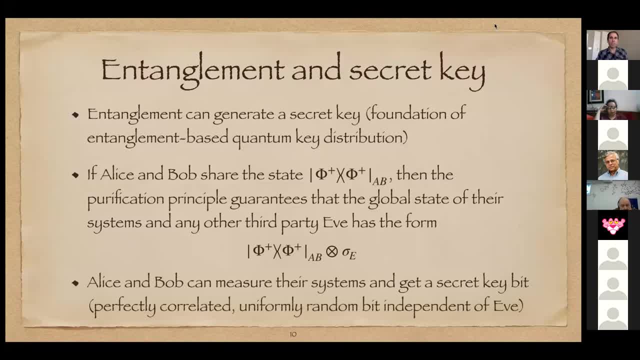 Okay, Can I ask a question? Please go ahead. Yes, On the CHSS game. you mentioned that people, Alice and Bob, they make non-local measurements. Did I hear you correctly? No, they do local measurements. Oh, they can make local. 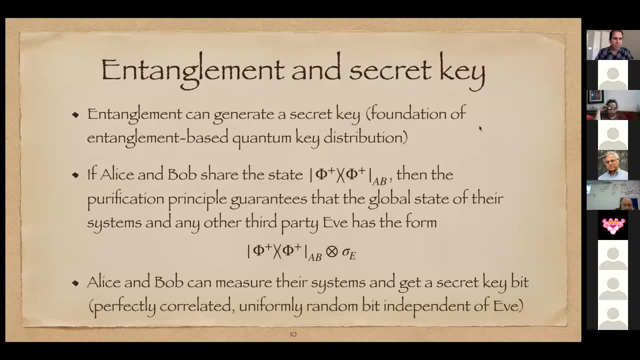 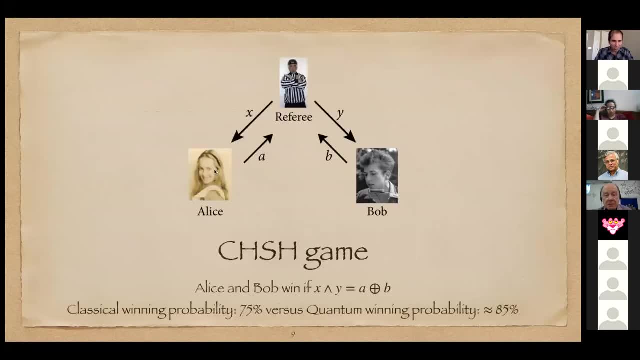 Okay, Yeah, They're doing. Sorry, Oh, now it's working. Okay, So we imagine that they share an EBIT before the game begins and then Alice is allowed to do. I think I said non-commuting measurements. Hopefully that's what I said. 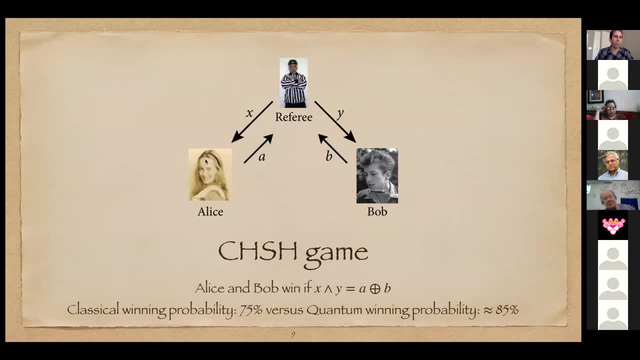 Okay, But the measurements are local. So I believe the winning strategy: Alice measures Sigma X or Sigma Z at random, And then Bob measures Sigma X plus Sigma Z at random, or Sigma X minus Sigma Z. You have to normalize that root too. 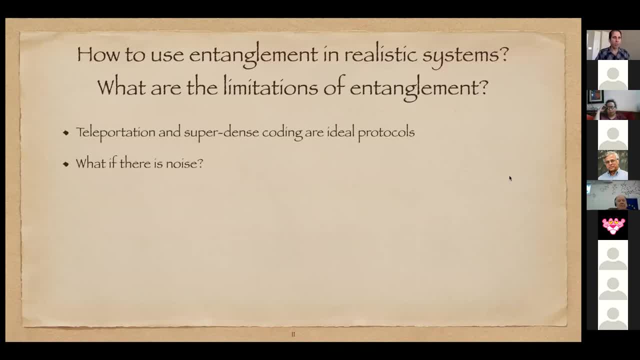 Okay, So okay, Now we're getting to. let me check the time. So we're okay, Good. The question then becomes: we've talked about these ideal protocols. The question then becomes: what if there's noise? what kind of things can we do? 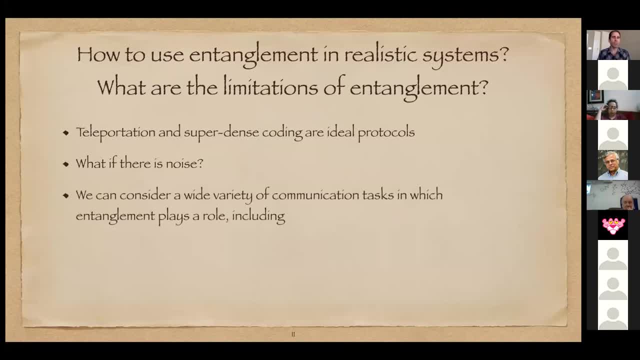 And that motivates the whole area of quantum Shannon theory, right? So that's, that's the topic on which I wrote. now two textbooks: one I did on my own, The second textbook we've put in the archive. I'll mention it later. 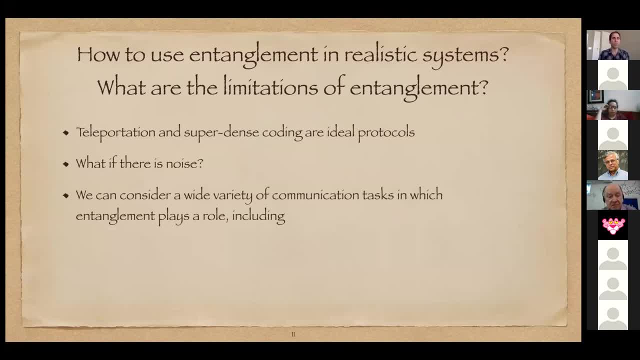 This was done in collaboration with the student at LSU, Samit Khachru, who's now going to be doing a postdoc in Germany. Okay So, but we can. you know, there's this question in these basic protocols: What if there's noise? 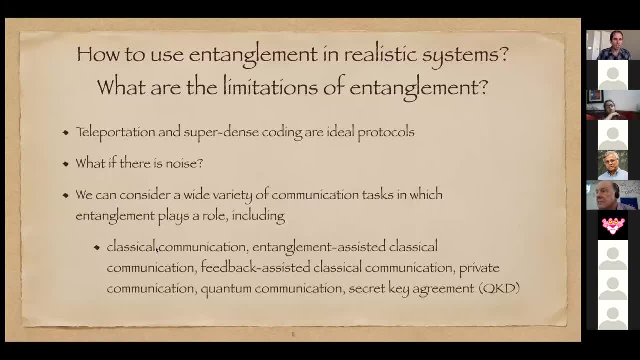 And then we can consider a whole variety of communication tasks: classical communication over quantum channels, entanglement, assisted classical communication. what if there's feedback? What kind of rates can we achieve? Private communication, secret key agreement- Those two are related and they're related to QKD. 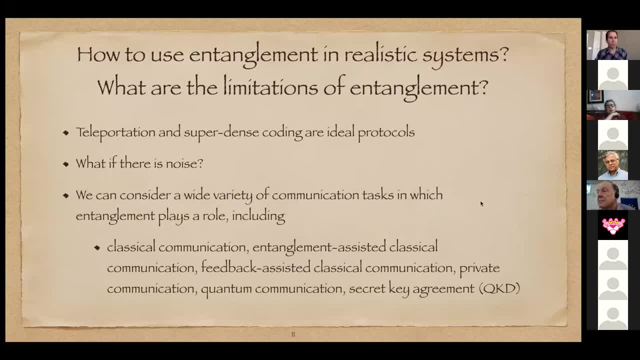 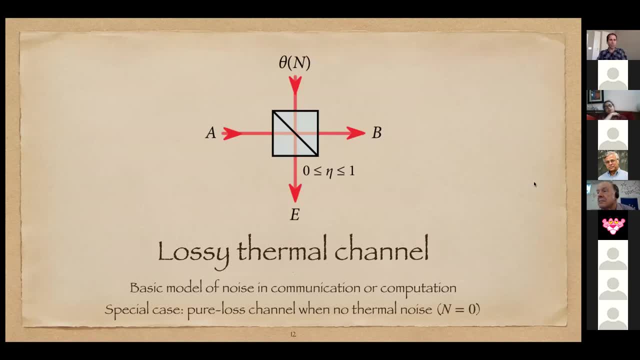 And finally, quantum communication, which is useful for distributed quantum computing. Just in the chat, Okay, All right. Um, so, if you want to think about a basic noisy channel that we would expect to encounter in practice and experiments, uh, it's this lossy thermal channel. 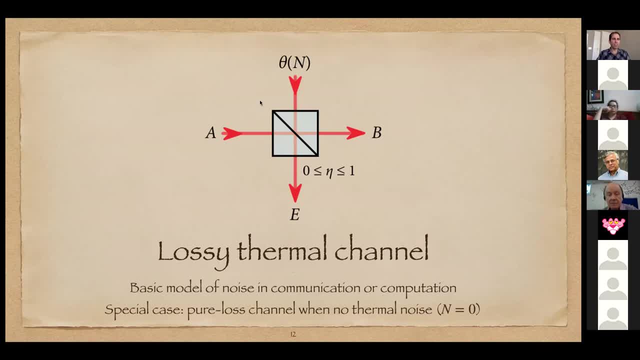 Okay, So what is the mathematical or what is a basic optical model This channel is? Alice has a mode of light that she's using to transmit a quantum state, and this quantum state. there are all kinds of choices that can be made. The popular ones include, like coherent states, uh, squeeze states that can 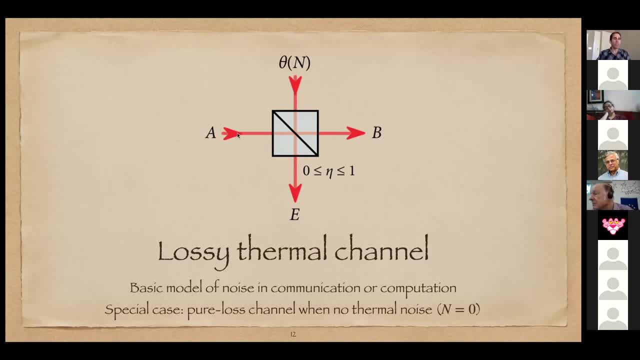 be one share of an entangled state, Anyway. So this input mode to be prepared in some state of light and then the inaccessible environment prepared, Okay, So this is a state that's thermal with respect to the, the photon number operators, the Hamiltonian. 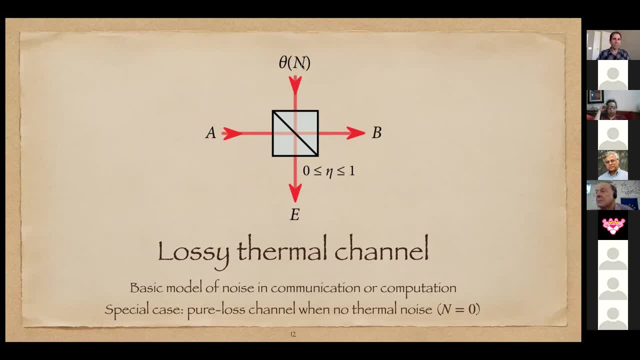 And uh N indicates the number of noisy photons, the mean number of noise and photons in this thermal state. And then the beam splitter represents loss And it, you know, ADA is the fraction of photons that make it through from Alice to Bob. 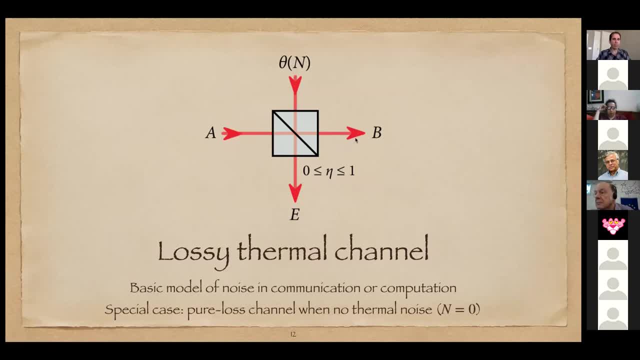 It's like the, the remnant of the input that makes it through from Alice to Bob, And it's also called transmissivity. Okay, And so Bob gets one output port of the beam splitter and then the environment gets the other output port, and you know it's, it's lost, right. 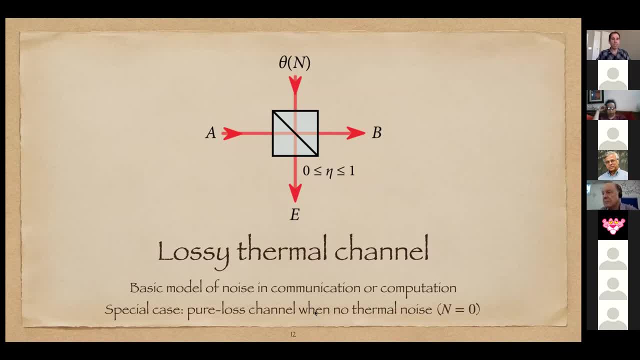 The environment is inaccessible. Okay, And then a special case of this is of wide interest in experimental practice also, when there's no thermal noise. In that case we call it pure loss channel, because the only uh noise that's due to. 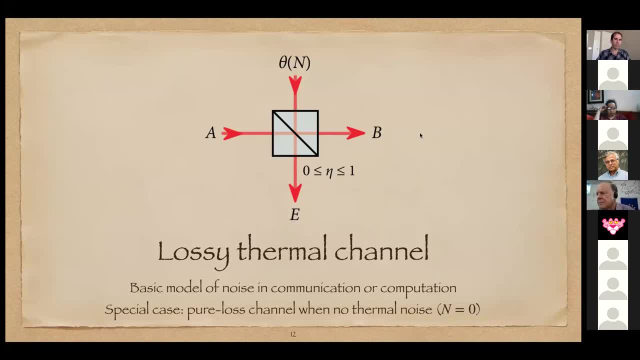 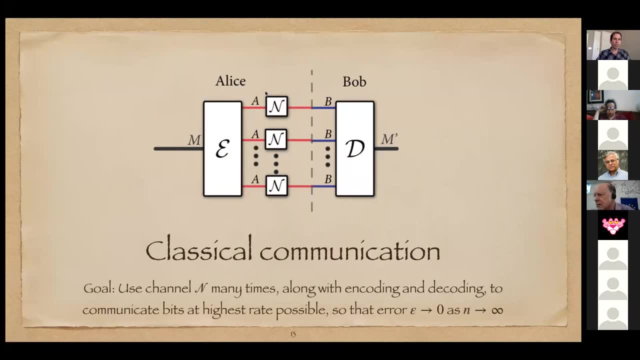 the, the, the channel is loss, Okay, Okay. So, um, here is a model. Here's how we can depict classical communication over QAM channel. So Alice wants to transmit some message, some classical message over many independent uses of the noise. 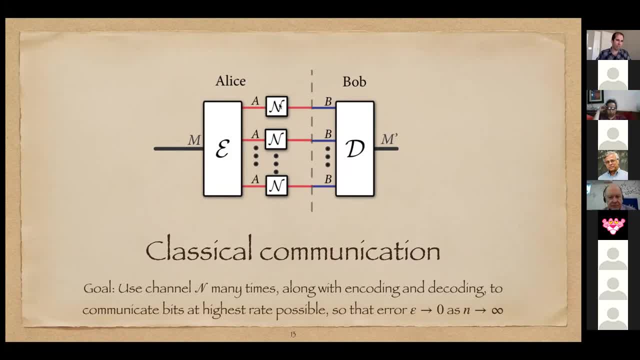 So, um, we say, is a is a quasi-noisy channel, ok, And so an example of that noisy channel could be the thermal channel. And she's allowed to do some encoding before communication begins? OK, And the encoding can be anything that's allowed by QAM mechanics. 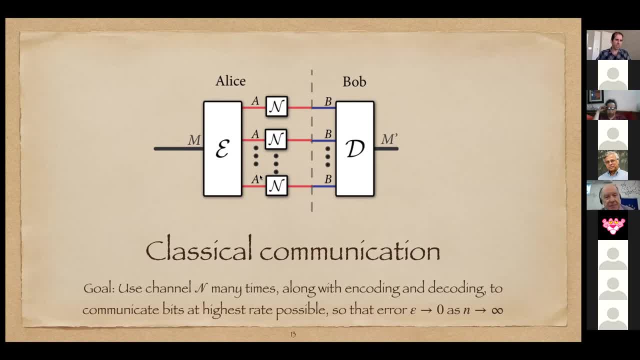 So we can prepare a sensor product of coherent states. that would be an example of a good choice for a thermal channel. But in general we can allow for entangled states, Okay. Okay, And it's known for some channels. coming back to entanglement, it's known that there 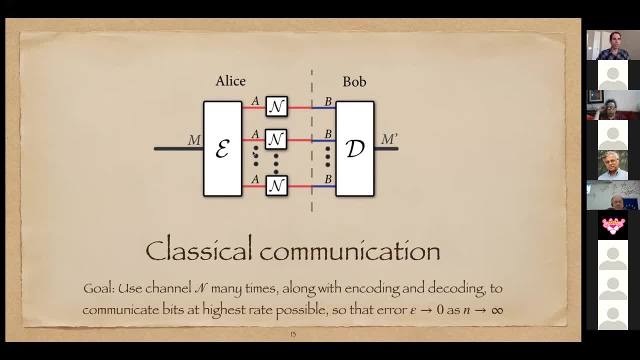 exist channels for which entangled code words can enhance the capacity, Okay, To enhance the ultimate communication rate. So then the other side of this is that Bob receives all these channel outputs and then he's allowed to do, again, anything allowed by quantum mechanics. 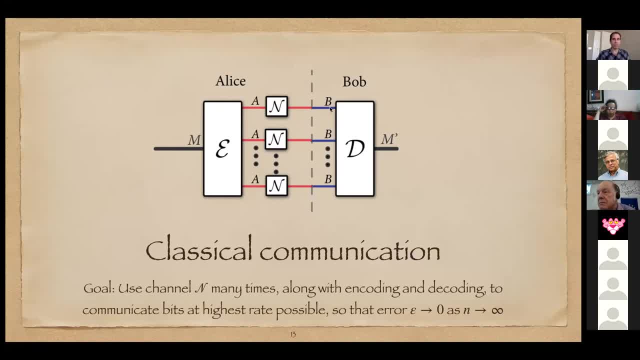 So it could be a collective measurement in which he's measuring all of the output modes And then the output of the measurement is some classical choice, It's some classical estimate for the message that was transmitted. And so, in quantum Shannon theory, what we want, 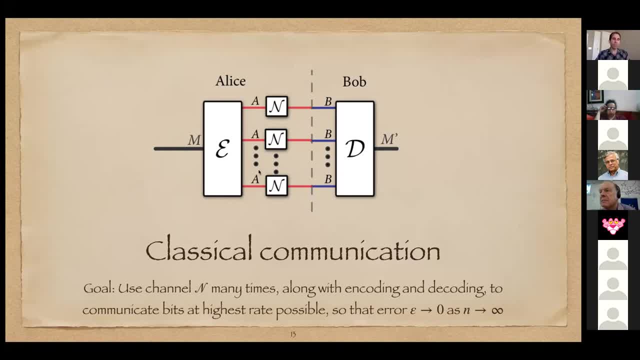 is that you're allowed to use the channel many times, along with any possible encoding and decoding. You want to communicate at the highest rate possible, such that the error in decoding the message is not a problem. So you want to communicate at the highest rate possible. 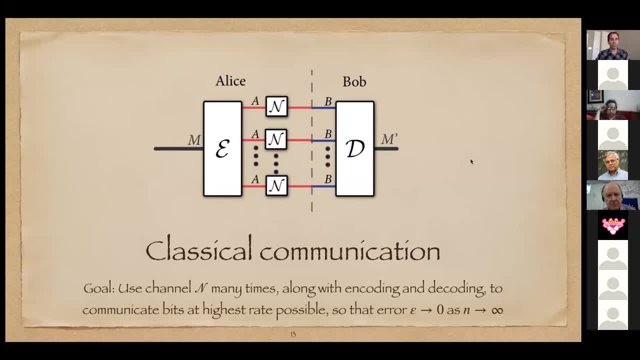 which decays to zero as the number of channel uses goes to infinity. So the highest rate possible is called capacity, And this is a notion that goes back to Shannon in 1948.. Okay, So what is done in a classical communication scheme is that you're just. 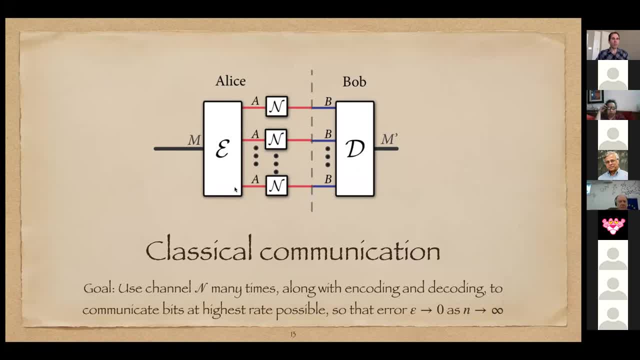 using what's called a product encoding. Okay, So the code words that are fed into the channel are tensor products of states And an example would be a coherent state: Okay, And then you know that goes through the channel, which could be a loss channel, And so some remnants of the coherence state. 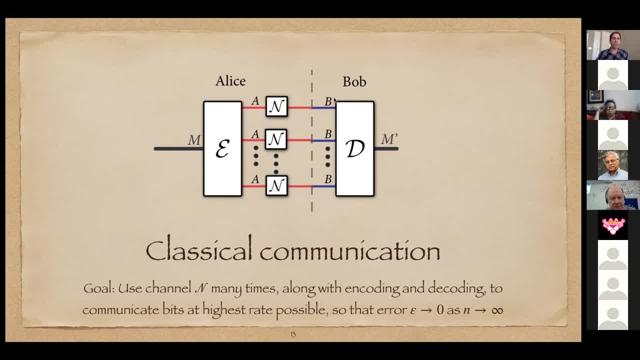 appears over here at the output, And then a classical strategy would have Bob perform individual measurements of each mode. Okay, And examples that are used in actual communication scheme are: schemes are heterodyne or homodyne detection, to use language and quantum mechanics. 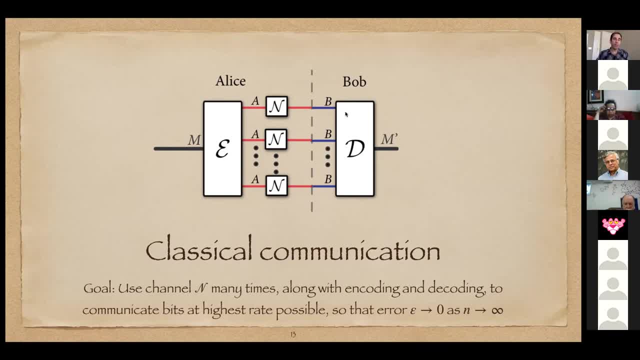 Okay And that'll get you a certain rate of communication. But it's known that if you allow for a collective measurement, you can achieve rates at the Halevo information rates. So that's related to work that Alexander Halevo did, as well as Schumacher and Westmoreland. 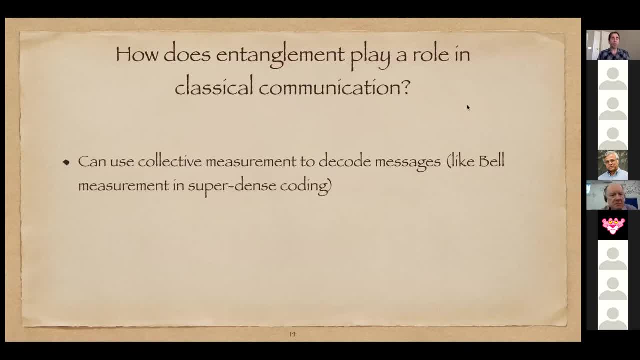 Okay, So how does entanglement play a role? Well, we already talked about some of that here. One of the ideas that you can use a collective measurement to decode the measurement, to decode the messages- And you know we talked about the example of super dense coding, the Bell. 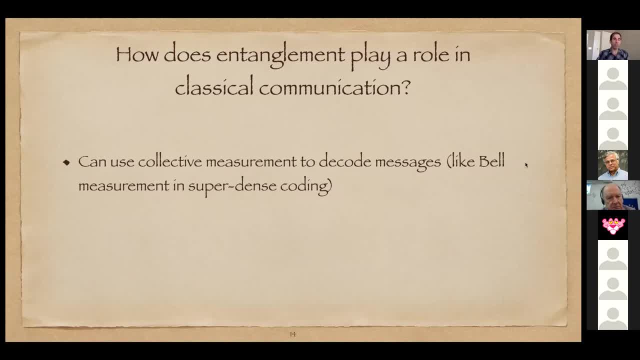 measurement. that's done. there is an example of a collective measurement. Okay, The other thing that can be done is to use entangled code words that can possibly enhance rates And, as we mentioned, there are examples of channels for which enhancements are possible. 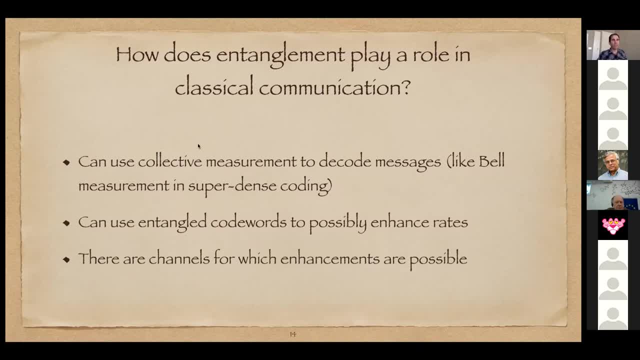 So explicit examples are known Where Collective measurements can enhance capacity. But if you combine collective measurements and entangled code words, explicit examples of channels for which capacity is enhanced, that's not known, There's only you know it's. it's known that there exists channels. 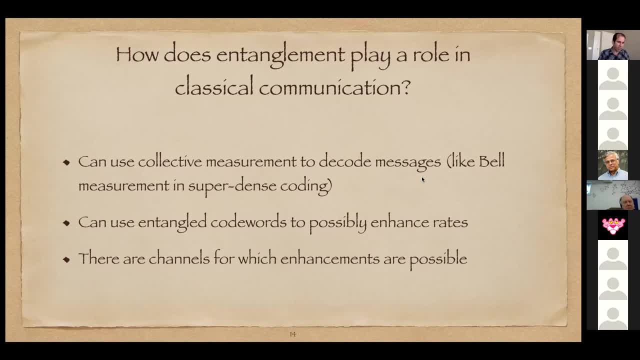 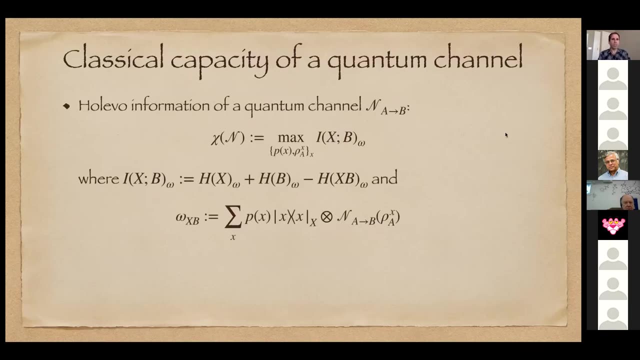 It's kind of. there was, channels were constructed randomly And then it was shown that among ensembles of channels, there exists channels. That's due to Matt Hastings 2008.. Okay, So what are? what is one of the main results for classical communication? It's this notion. 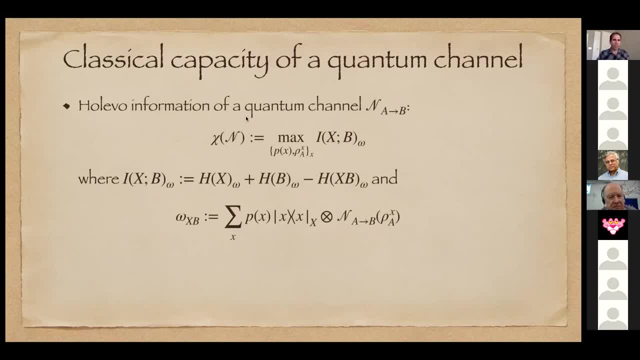 of classical capacity. So we can measure the classical correlations that can be generated by a channel, by using this quantity that generalizes Shannon's mutual information- It's called Halevo information- And what you do is you. you pick a probability distribution over classical. 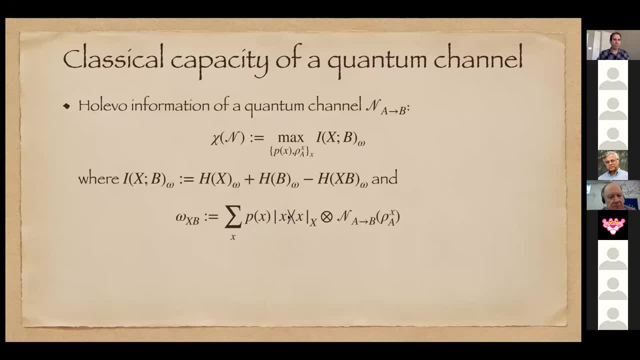 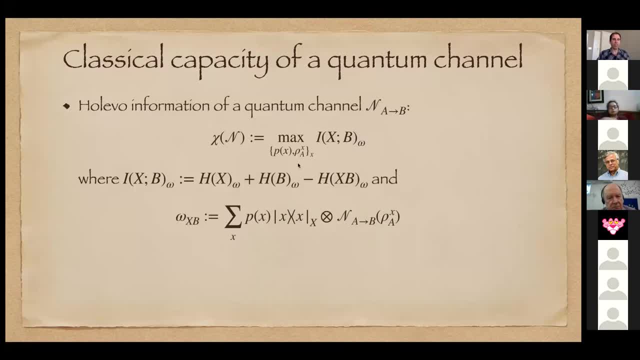 Rick, I uh kind of look through real soon. All right results of Halevo, Schumacher and Westmoreland is that this is an achievable rate for communication over a QAM channel. So in principle there exists error correction codes that can achieve this rate. 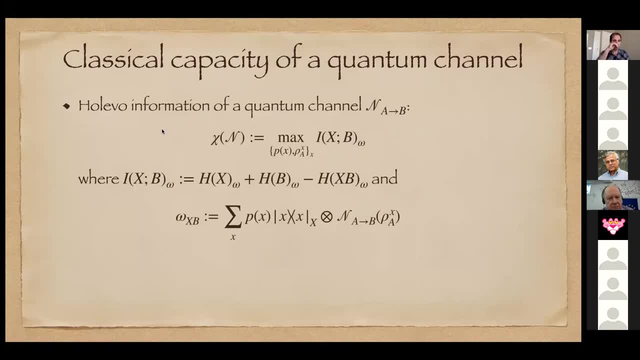 There's a choice of encoding and collective measurements. that can be done at the decoder And this mutual information is a linear combination of entropies: The two marginal entropies of this bipartite state minus the joint entropy, and that's a correlation measure. 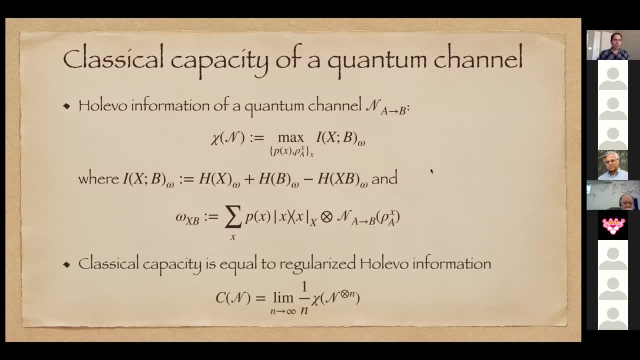 Okay, And you know, depending on your viewpoint, this is either very interesting or unfortunate. The classical capacity is equal to this regularized Halevo information, So you have to take this quantity that we defined here and evaluate it for a tensor product. 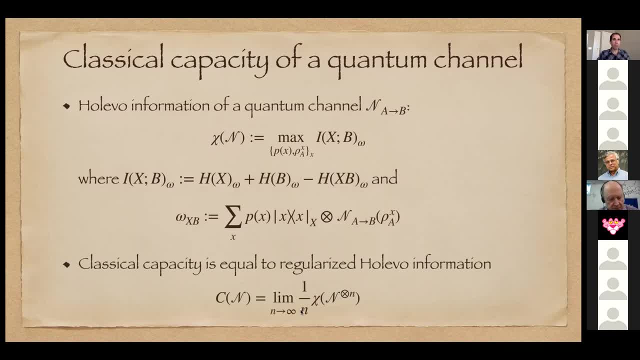 so many uses of the channel, divide by the number of times you used it and take this limit. Okay, And for some channels, like the thermal channel that I mentioned previously, it's known that you don't need to do this limiting procedure. It's known that the Halevo. 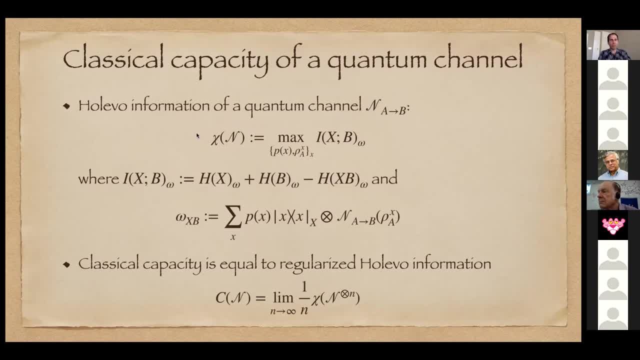 information is actually equal to the capacity And for the thermal channel, we know explicit formulas for the capacity in terms of the transmissivity of the thermal channel And the thermal environment noise. That was a landmark result due to Halevo, Giovannetti, Garcia-Petron and Cerf back in 2013.. However, in general, it's believed that this limit 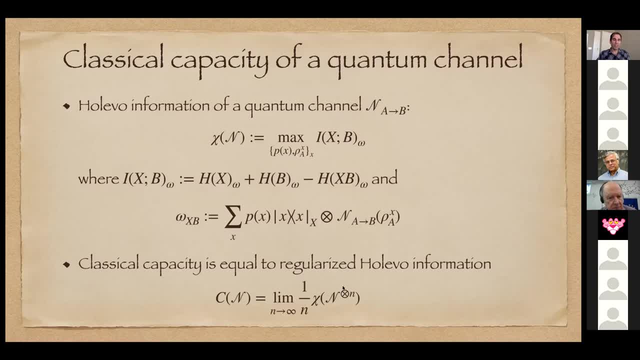 is necessary. Okay, And so then research questions have revolved around. well, it's going to be hard to compute this quantity, or at least we believe so- And there's actually a big open question here whether this quantity is even computable in the sense of Alan Turing. 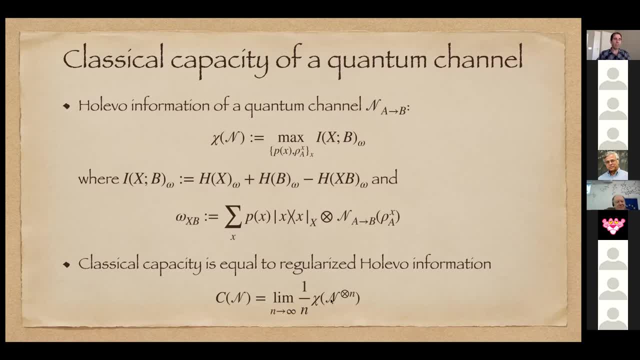 But you know, given the belief that this quantity is hard to compute, you can then try to bound it from below and from above, And so you know, that's research that I've been involved in, others have been involved in, And we try to come up with clever ways to bound this quantity. 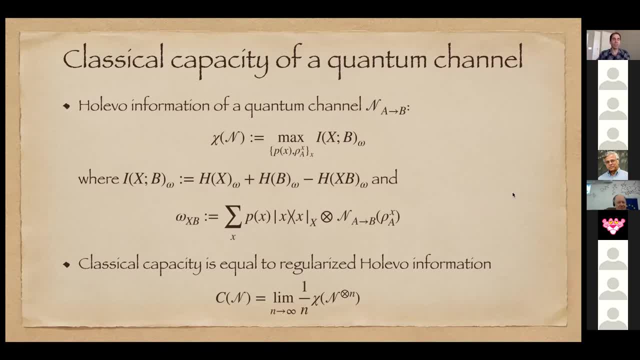 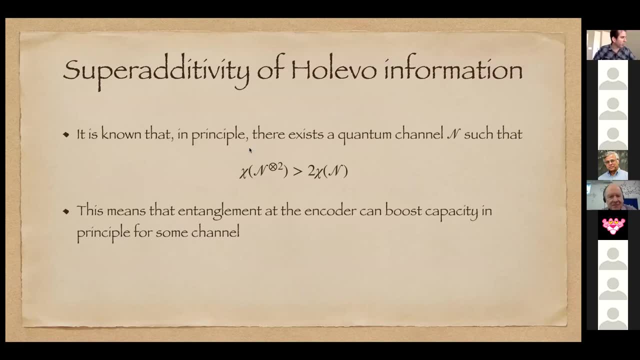 to try to narrow down the capacity, maybe identify it for key channels of interest. Okay, Related, so this is more detail about the Hastings result I was mentioning earlier. Hastings proved that there exists a quant channel such that if you evaluate the Halevo information, 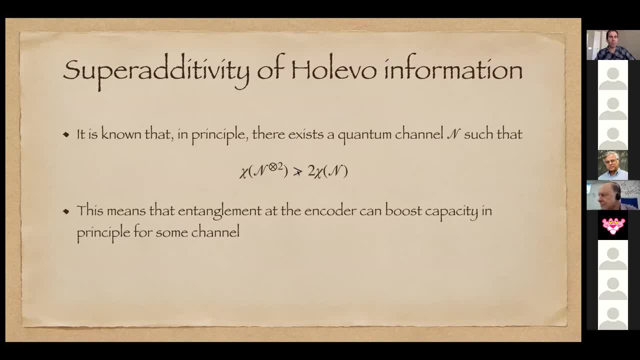 for two channel uses, that value is strictly larger than twice the Halevo information of the individual channel, And so we can interpret this as saying that if we use bipartite and states of the encoder, that can boost the capacity. in principle Okay, But indeed a major challenge for quantum information is to provide such an example. 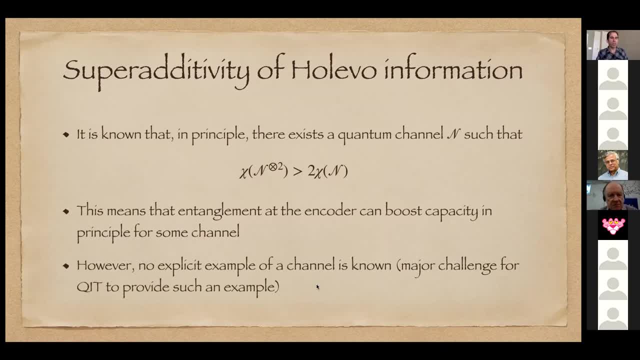 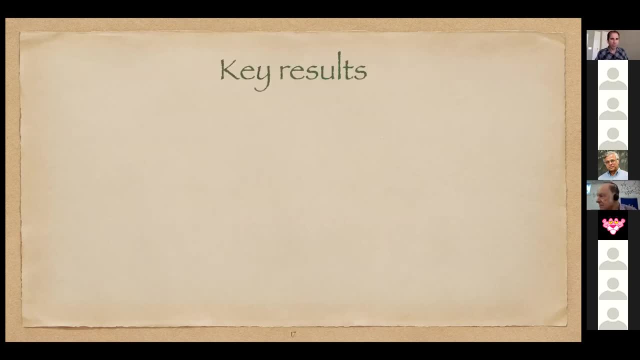 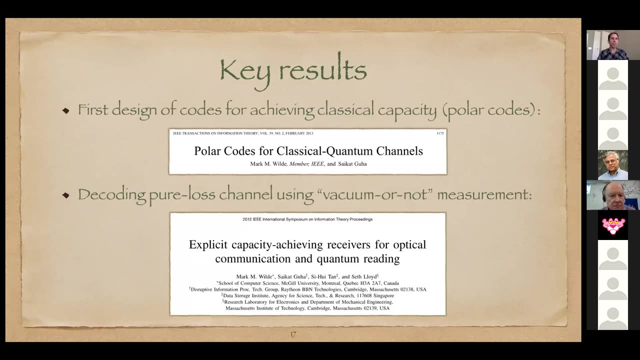 If you're interested in recent progress in this question, you can read papers of Pranab Sen. He's at TIFR in Mumbai, Okay, And then I'll tell you some work that I've done on this topic if you're interested in learning more. 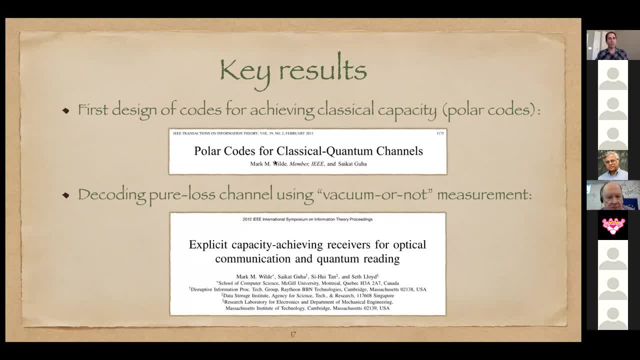 So we were the Saikat Guha, who's my colleague at University of Arizona. We wrote a paper about designing error correction codes for achieving the classical capacity. We were inspired by work of Arikhan, who won the Shannon Award some years ago. 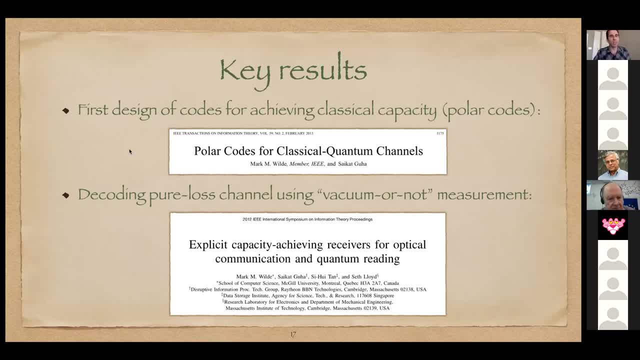 by inventing this, And so we took his ideas and we generalized them to the quantum case, And so if you're interested in designing codes for achieving capacity or achieving the Halevo information of channels, you can look at this paper And then this paper that I wrote with Saikat and Sihui Tan and Seth Lloyd. 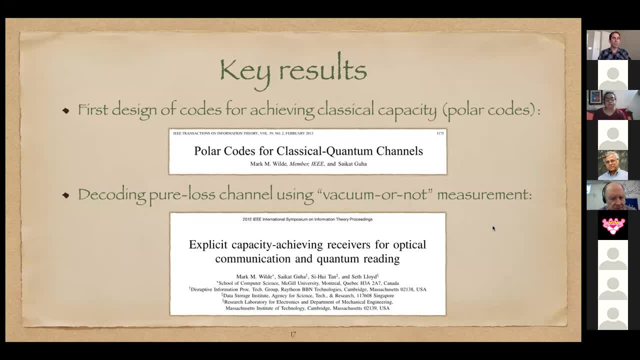 we designed a measurement that can achieve- if you can build it in the lab, then you can achieve- the capacity of the pure loss channel, And this is a measurement that I believe would be very difficult and challenging to implement in practice. We call it the vacuum or not measurement. 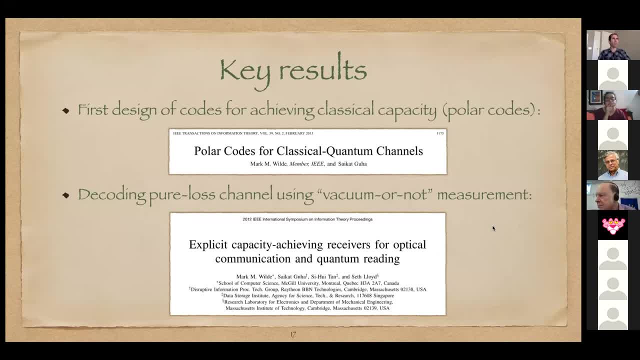 What it has to do is it has to coherently project onto one of two possibilities: Either the all vacuum state of n modes or the identity minus that Okay. And what's critical is that if you get the outcome not vacuum, which is identity minus the vacuum, 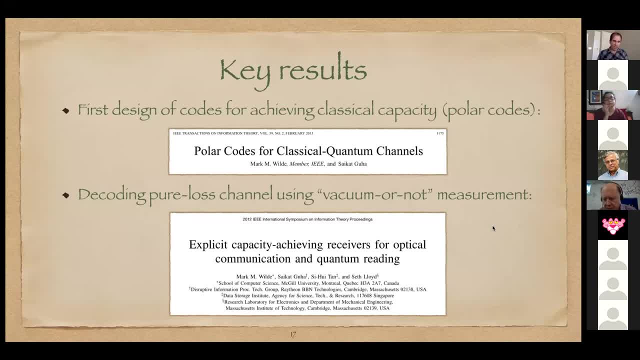 then the state, the resulting state after the measurement should be the state with the vacuum subtracted out. Okay, And so that's the part. the not vacuum is the part that's hard to realize in practice. to do that coherently, There was a paper with a very 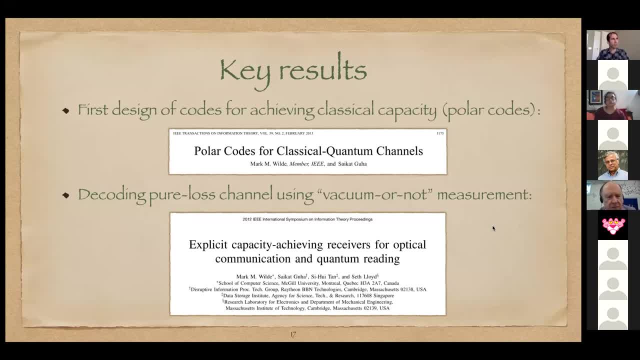 I don't know how popular the TV show Seinfeld is in India, But there's a paper by Daniel Oi called Measuring Nothing And it was about trying to, you know, realize this vacuum or not measurement, And at least a theoretical proposal for doing so. 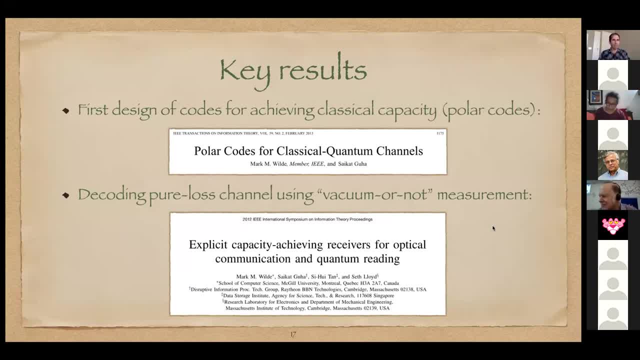 Ultimately, the editors of Physical Review Letters made him change the title to something much more boring, But on the archive it's called Measuring Nothing. Okay, Is there a question in the chat? Oh, can I please say what are polar codes? 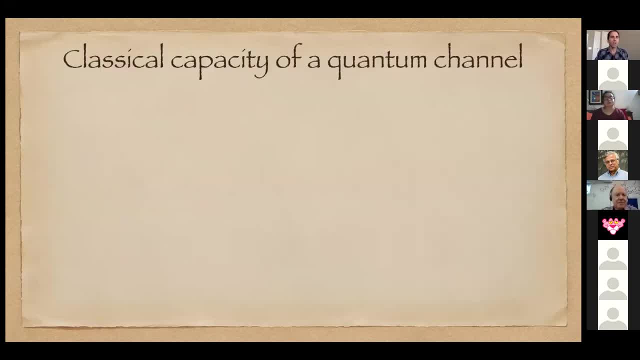 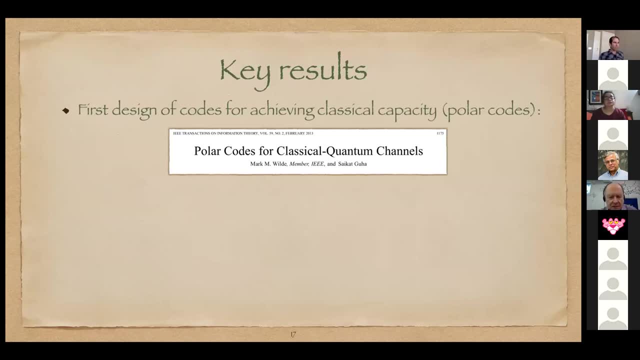 Yes, Let's see. So polar codes. briefly, what they do is you take end uses of the channel And then, by encoding of the channel, you realize what are called virtual channels, from one bit of the input of the encoder to all of the outputs. 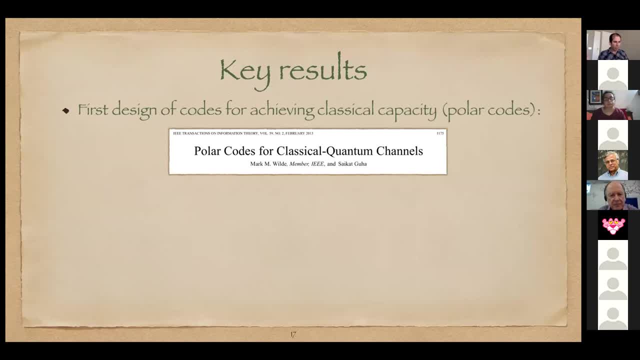 So that realizes you know, like a binary input channel, And then you can consider these virtual channels for every possible input bit. Okay, And then what Archon proves is that these virtual channels polarize, Meaning that either they are near perfect or near useless. 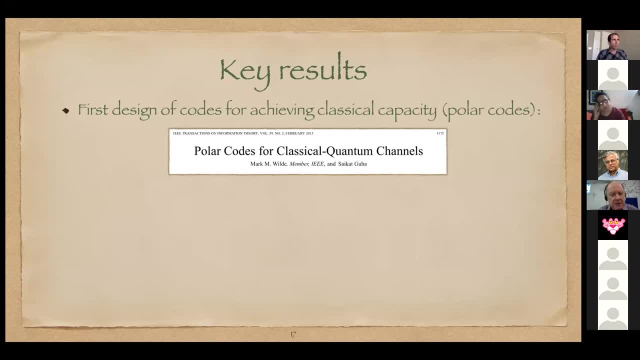 Okay, And so the idea of the encoding scheme is that, well, if you know that some are near perfect or some and some are near useless, you encode the bits you want to transmit into the near perfect channels And you put ancillary bits that you just set to zero. 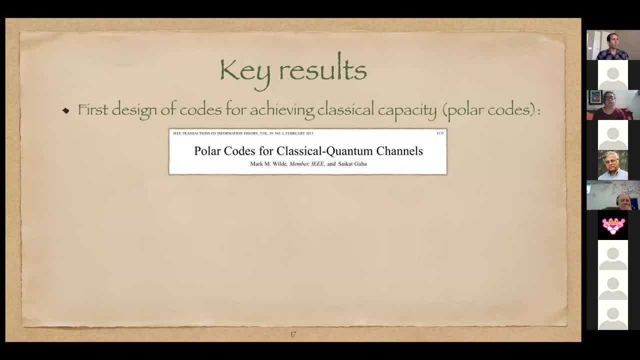 Archon called them frozen bits. Then the useless channels, And what he proved is that the fraction of the overall channels that are near perfect, they're equal to the capacity, And so that's that's the idea behind them. It's a really beautiful paper. 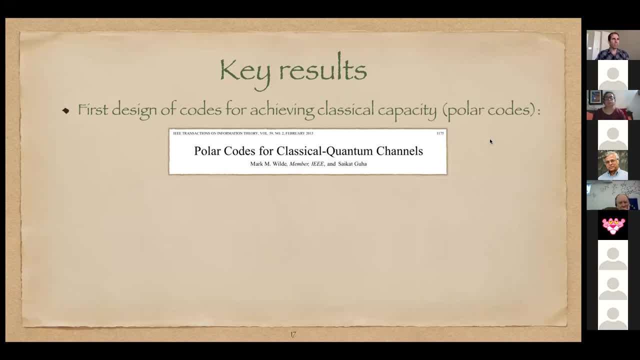 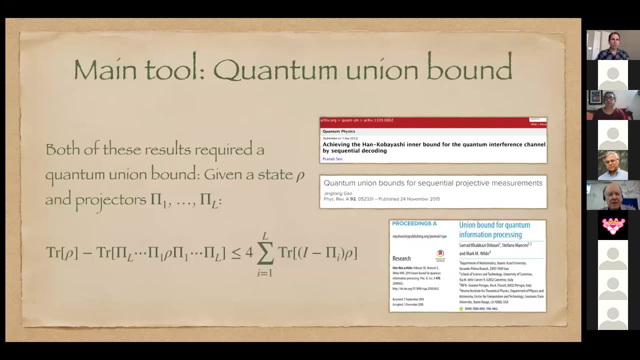 Like that was. that was quite an uplifting experience actually, personally to read Archon's paper, So if you're into that kind of thing, I highly recommend it. Thank you, Charlie, for your answer also. Okay, So I want to mention something interesting. 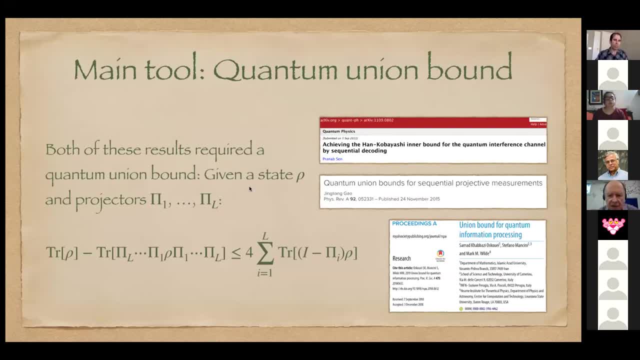 a technical tool that was used to prove these results. It started with work of Pranab Sen and was subsequently improved by a Chinese researcher, Gao Jingliang Gao, and subsequently improved by Samad Stefano and myself. 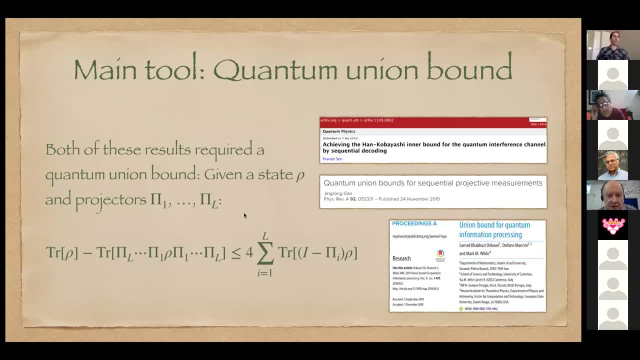 It's what we call a quantum union bound, right? So the union bound is so ubiquitous in classical probability theory, And you know it's, it's used everywhere, It's like a basic tool. So this is a quantum version of it. 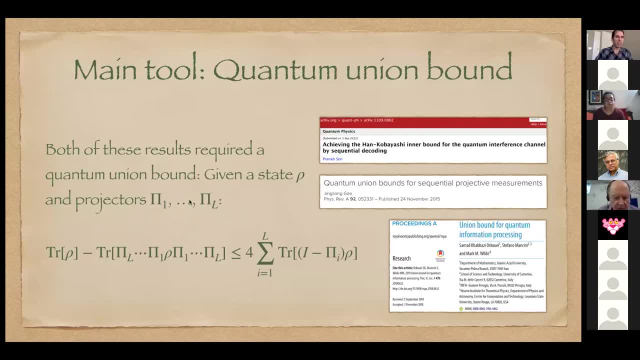 Okay, So the idea is that if you have a state and a sequence of projectors and you can think of each projector as being as one element of a two outcome measurement, right, So pi one could be pi one and identity minus one is a two outcome measurement. 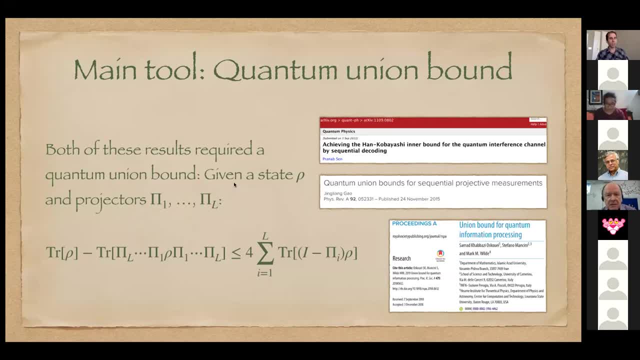 And so you think of each of these as a two outcome measurement. And so the application, or why it's useful in quantum information, is when you're decoding, you could decode successively. You could ask like: is it the first message? Was the first message transmitted? 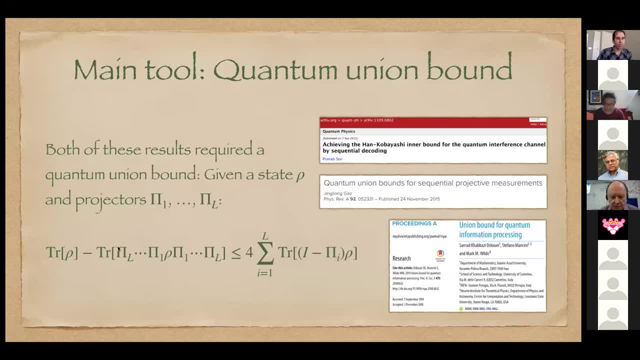 Was the second trend message transmitted, Was the Nth message transmitted, And so you'd want, like a certain sequence, a certain sequence of outcomes to occur. Okay, And so you can think of this right. here is the probability that a correct sequence of events occurs. 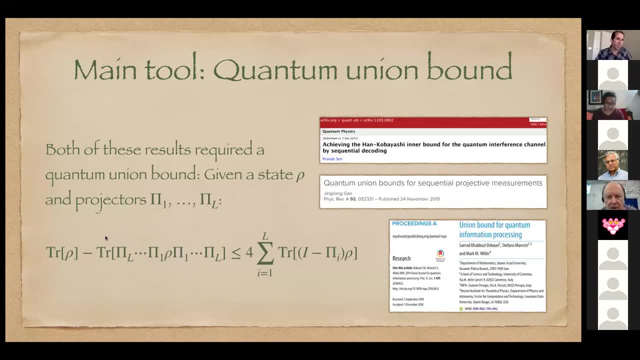 And in classical probability theory you would think of this as an intersection of events. Okay And so trace of rho minus that if rho is a state, this is one. So one minus. that is the complement. So in classical probability theory, 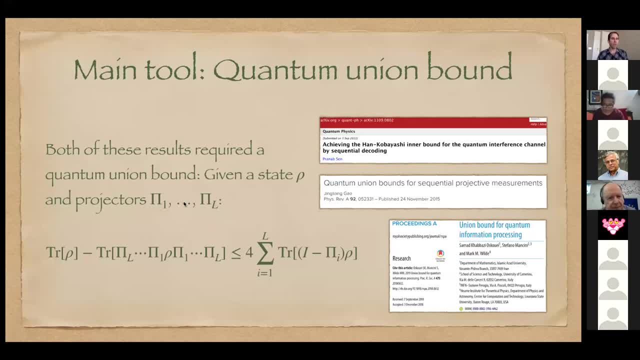 it would be a union of the complements, The complements of the individual events, by applying the Morgan's law. So what the union bound says is that this probability of an incorrect sequence of events is bounded from above by the probability that the sum of the incorrect probabilities 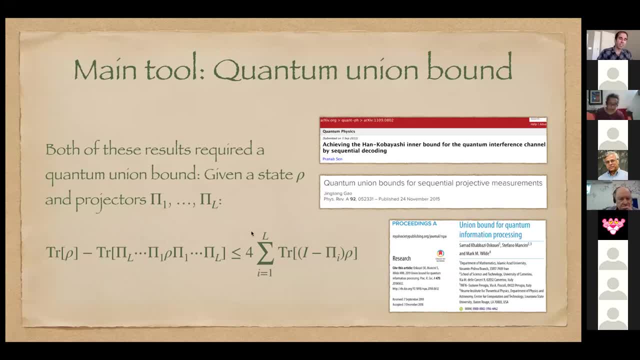 the sum of the individual errors. Okay, And in probability theory you don't have this factor of four, but due to this, due to us being in quantum and these projectors don't have to commute, the factor of four appears. 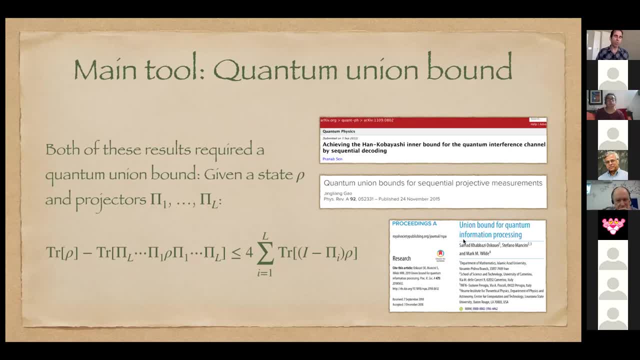 I forgot to list the recent paper of Ryan O'Donnell and his student. Ryan O'Donnell is a computer scientist at Carnegie Mellon who's more recently done a lot of wonderful work in quantum information. He has a recent paper called Quantum Union Bounds Made Easy. 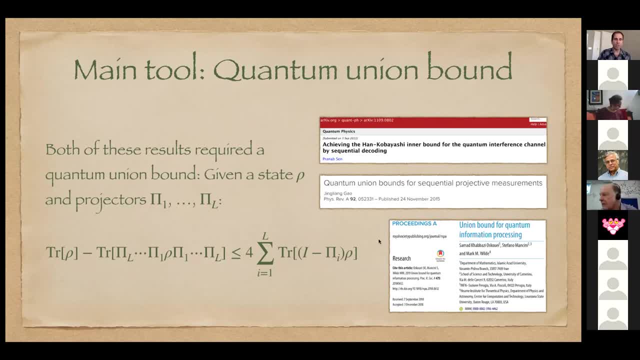 I think he was frustrated looking at all of these papers and the proofs and finding them complicated, And so, you know, tried to make it simpler, And it's an interesting paper. I'd recommend having a look. They also prove that this factor of four is 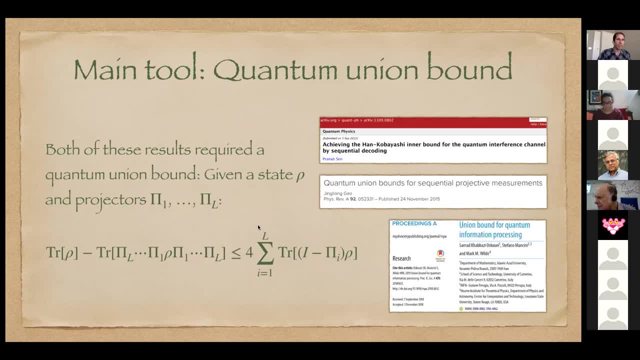 there's a sense in which this factor of four is optimal, that you cannot make it any lower in the general case. Okay, So there's more things in the chat. Why are polar codes Okay? Good, So I think I have about 15 minutes left. 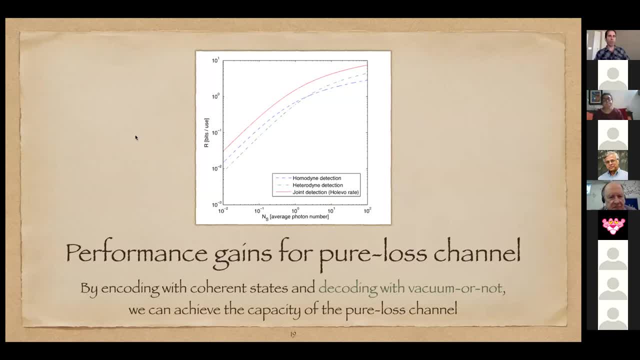 Yeah, Sure, Let me try to keep progressing. I will not be able to get through all the slides that I have, but I'm just going to try to give you a sense of some other things. So we were talking about differences between classical and quantum information. 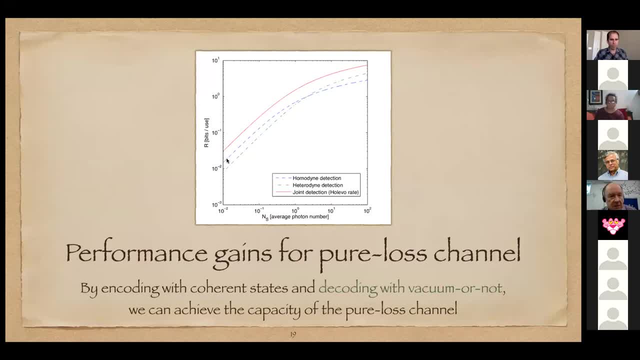 So this shows a nice gap that one can achieve for classical communication over optical channels like the pure loss channel. So this is rate in terms of bits per channel use versus photon number that you're allowed to use for the encoded states. 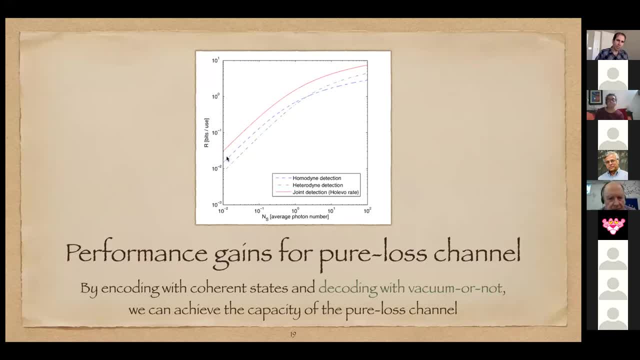 And what you see is that, if you're using homodyne detection or heterodyne detection, there's only a certain rate that you can achieve, as where, if you use joint detection, this collective measurement, you can achieve a much higher rate than principal. 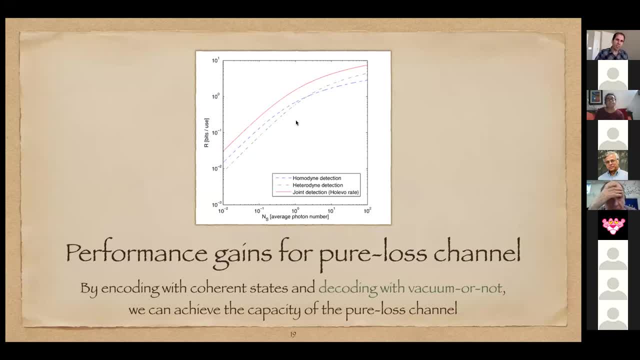 Okay, And it's interesting that for low photon number, homodyne detection does better than heterodyne detection, And that's because these lower photon numbers, homodyne detection, is measuring one, just one quadrature, And so there's less of a noise contribution from the vacuum. 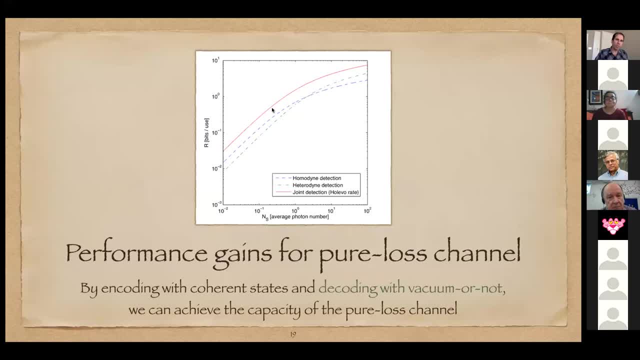 That's where, when the photon number gets larger, that noise contribution from the vacuum doesn't matter as much, And there's a sense in which heterodyne detection realizes two parallel channels. because you're two parallel classical channels, because you're. 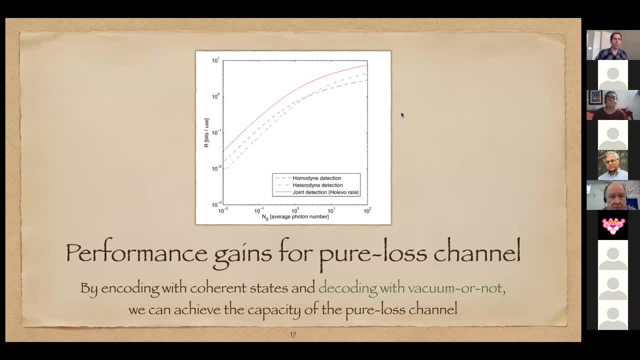 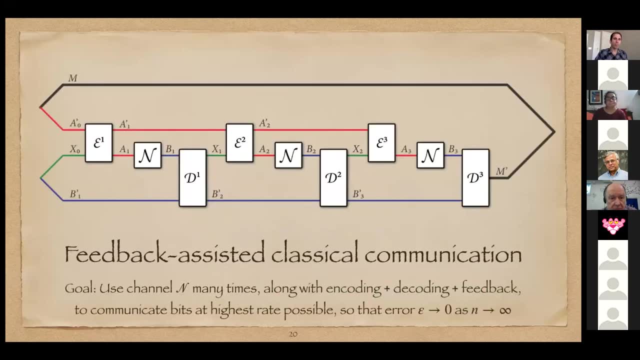 you're measuring. it's kind of like you're simultaneously measuring both quadratures, And so for higher powers or higher energies, you can achieve a higher rate. Okay, Now I want to talk about feedback assisted classical communication. This is a topic that I put. 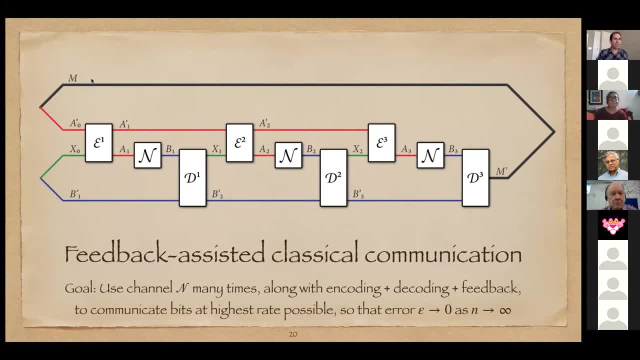 I personally find very interesting, And the diagram becomes quite a bit more complicated. So, but the idea is that Alice has a classical message that she wants to transmit to a Bob, to Bob, and Bob is now allowed to send classical feedback. So anything green now is classical in this diagram. 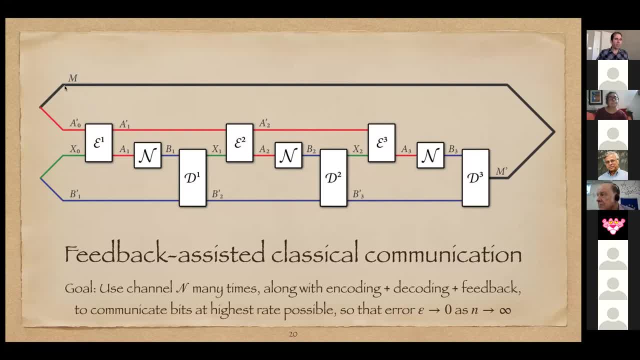 Okay, So you know, based on the value of the classical message, Alice can prepare a quantum state And Bob can send classical feedback. They can do an encode. Alice can do an encoding. keep a scratch register in a local quantum computer. 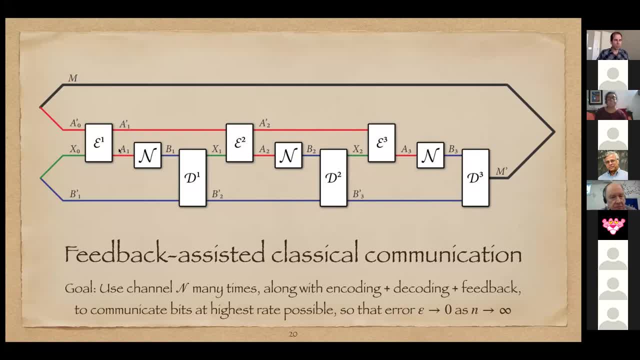 and then send one mode over the, the system over the channel, And then it leads to an output for Bob. He can then take what's there in his local quantum computer and do a decoding. The decoding will have his output, a classical register that he sends back to Alice. 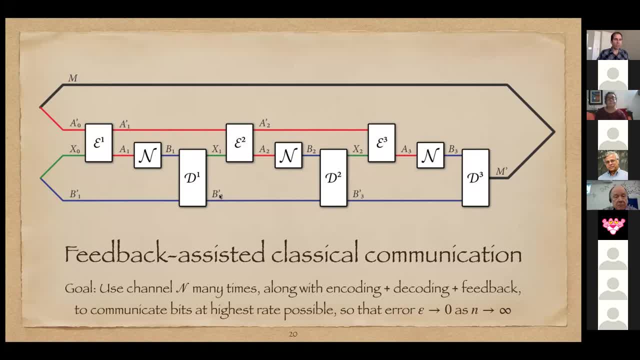 And the local memory registered that he stores in a quantum computer. And then this process iterates And there's questions like: okay, this feedback improved capacity. If not in the asymptotic limit of many challenges, does it help in the non asymptotic regime? 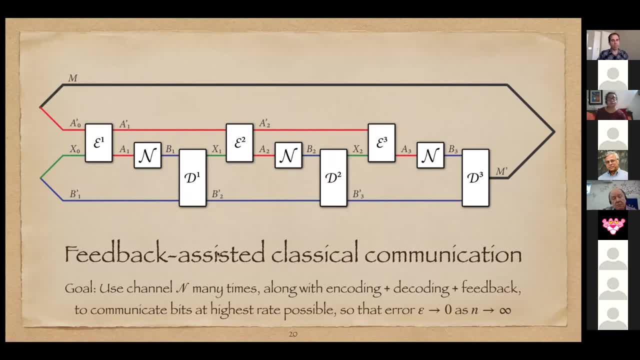 And so there's a notion of feedback, a system capacity. There's a famous result of Shannon That You know, in the case when the channels, when everything's classical, That in the asymptotic regime, feedback does not increase capacity. Okay, 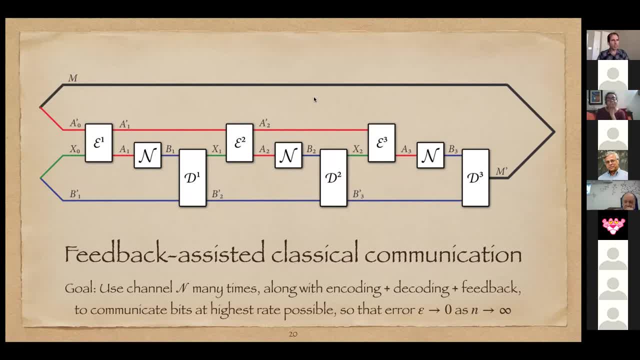 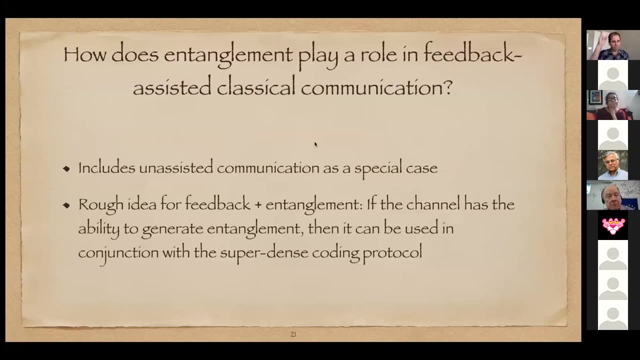 So that's like a landmark result for classical information. I think he showed that in the late 1950s When he introduced the notion of zero error capacity. also, And what's very interesting, is Feedback, This classical feedback in the quantum case. 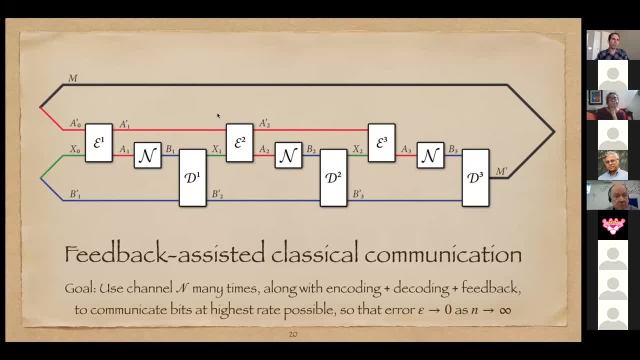 There are examples of channels Known for which feedback can increase the capacity, Even just classical feedback. This was Proven by Graham Smith and John Smolin Back when they were at IBM Around 2009,, I think, And so 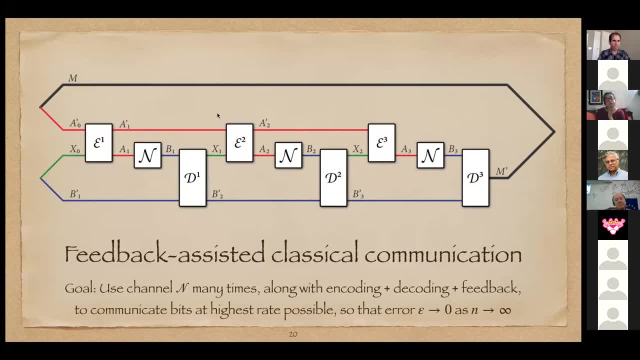 That is a key separation between the classical and quantum theories of information. They showed an example of a channel For which without feedback The capacity Is no larger than two bits per challenge, But then with feedback It can be proportional To the dimension of the input of the channel. 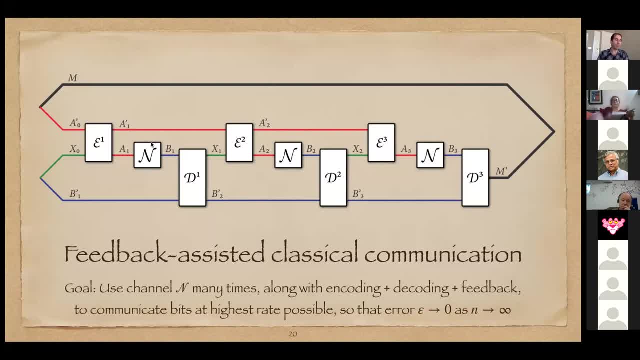 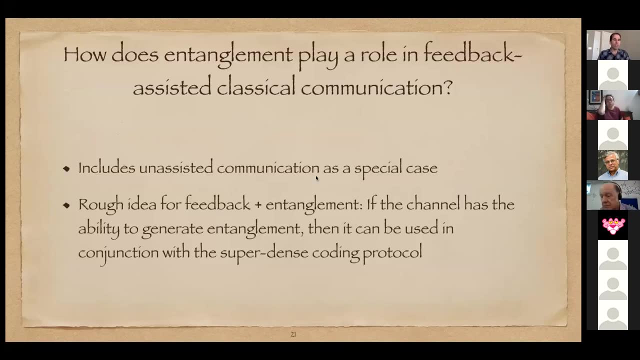 So if the dimension gets larger and larger, The capacity is unbounded. So that's a huge separation between classical and quantum That I think deserves Further study. Okay, So The rough idea that Smith and Smolin used Is that: 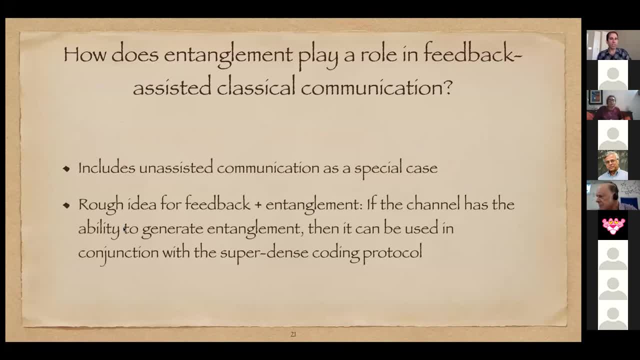 If the channel has the ability to generate entanglement, Then you can use that entanglement in conjunction with the super dense coding protocol. Okay, Like with super dense coding, you can send Two bits per channel use if you have entanglement. 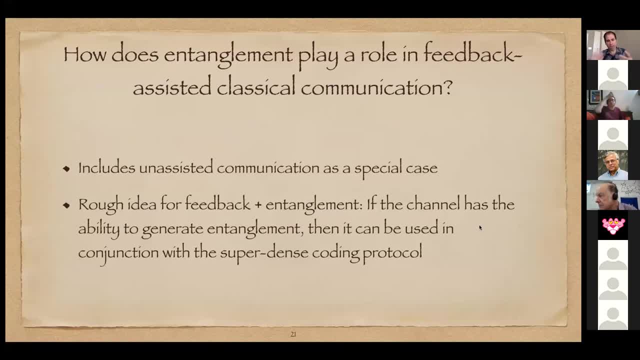 And so Somehow you can, you can use This idea to get a gain in capacity, but it doesn't work for every channel. It only works for Certain channels, And There's there's a question of Whether you would expect to encounter the Smith's small and channel in. 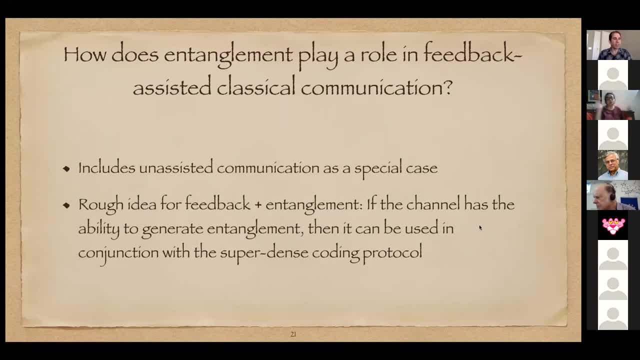 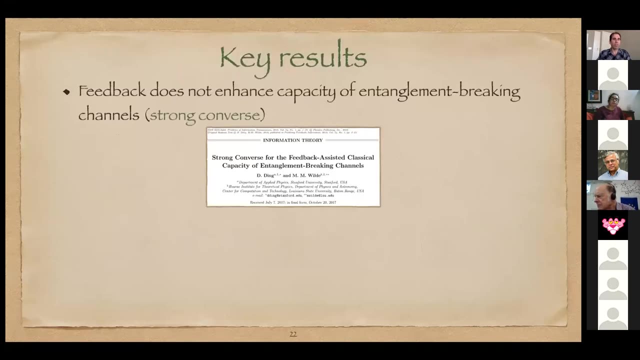 the wild. You know, I think The answer Probably no, And so it would be very interesting, like for the thermal channel, to figure out whether Feedback increases the capacity. That's something that we've Thought about over the years, but we don't have a definitive answer. 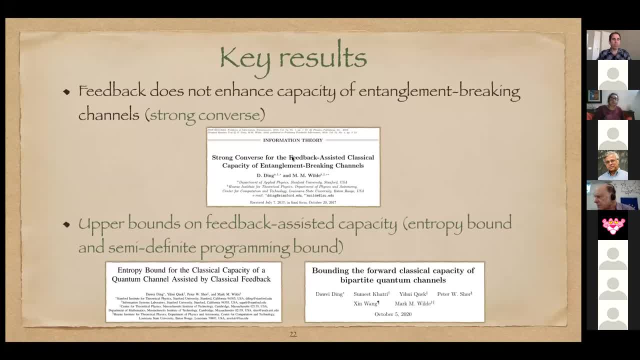 What I've done on this topic Is we showed There was an earlier results of Gary Bowen and his coauthor Where they showed that If the channel is entanglement breaking, like if it has no ability to generate entanglement, 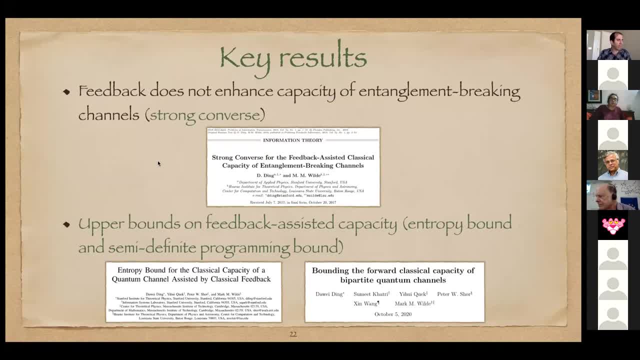 Then feedback does not increase capacity, And then we came in and showed something called the strong Congress, which Which says that If the rate of communication exceeds the capacity, the error probability will actually tend to one, And so That's something that we've done. 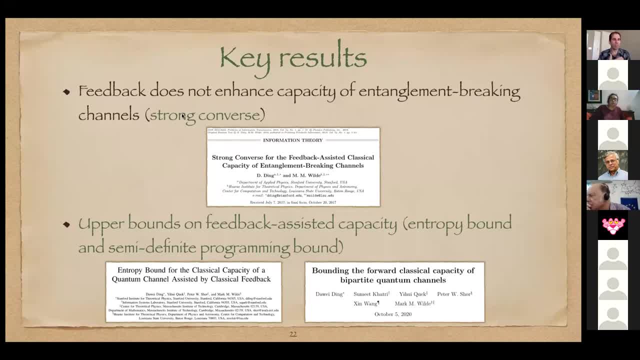 And so You know, We've been trying to figure out what's possible and what's not, And so These strong Congresses Show that the capacity is like a very sharp dividing line between what's possible and impossible. The other thing I've done on this topic, that's in collaboration with 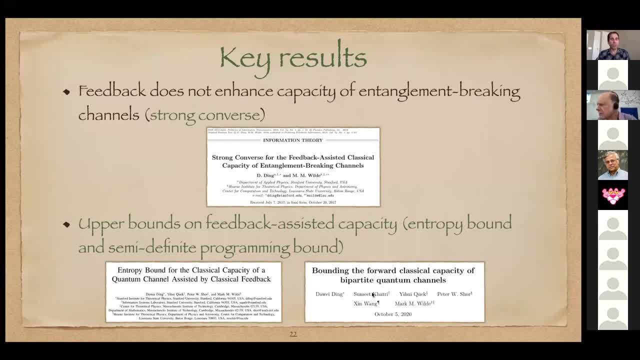 David, You, You quite quick, Peter short, And so meet. you know he's my coauthor for the book, and and Shin Wang. So we've been trying to give upper bounds On this feedback, assist, the capacity, And so in this paper we showed an entropy bounds. 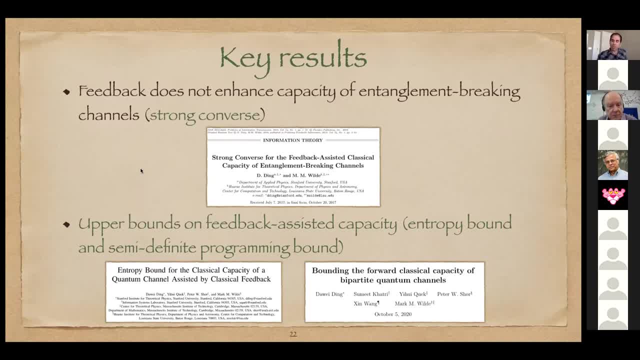 So the maximum output entropy of the channel. There's an upper bound on the feedback assist, the capacity. We use that result to show that For what's called the quantum eraser channel, feedback does not increase capacity, And also for the pure loss channel. 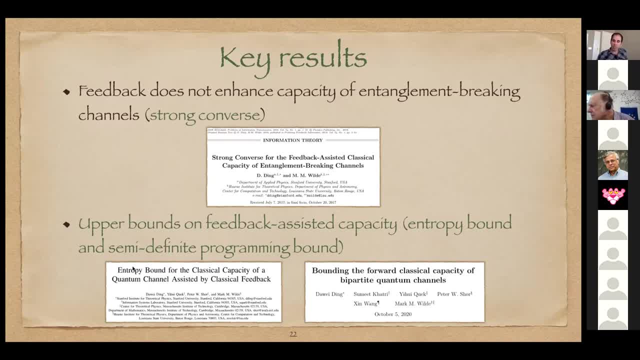 We now know that feedback does not increase capacity, And so There's this lingering question about thermal channel that I mentioned In this more recent paper, And so We've established a another, a different kind of upper bounds On the capacity. 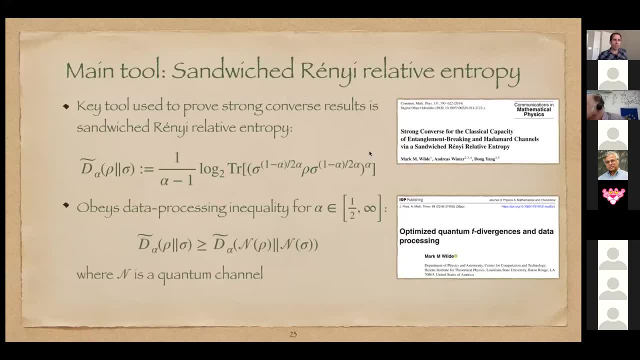 And related to something called Bipartite channels that I won't get into. There's a tool that we use To prove some of these results. It's a. it's a Distinguishability measure. Introduced This paper And independently in the paper by Marco. 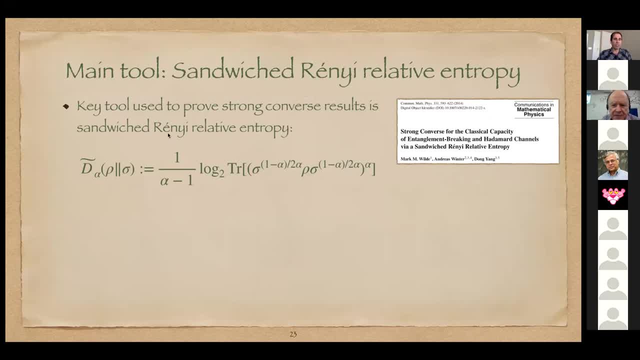 Michelle, Where it's called sandwiched Renny, relative entropy, And it's, It's, It's, It's. It's seen a lot of use, not only in One Capacity kinds of things, But also in thermodynamics and 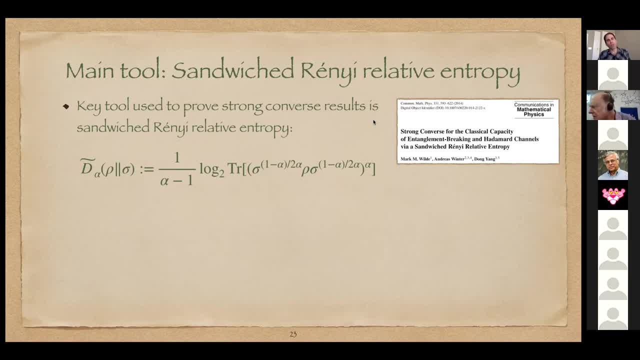 Even by people in high energy physics. So it's, it's an interesting generalization of the notion of Renny relative entropy introduced by renting, And what you do is you Sandwich the density operators in this way And then you get a measure that reduces to the classical. 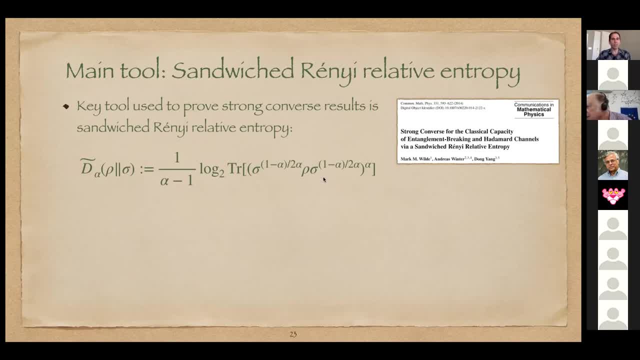 Relative entropy, But then for Non-community in states that can Behave in interesting ways, And what we know is that it obeys the data processing inequality For alpha between one half and infinity. This was shown by. This was originally shown by. 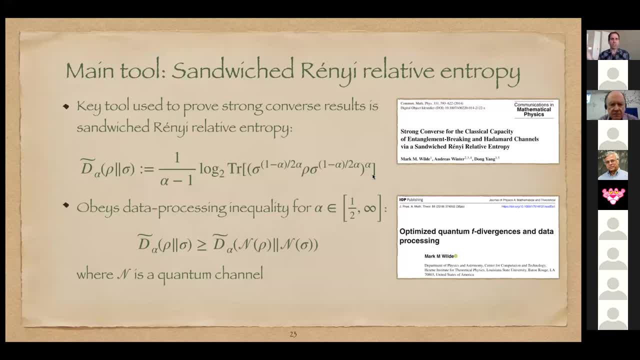 Rupert Frank and Elliot leave And it was shown by others. And then This is a paper that I wrote where I came up with A different proof That's more like Dennis pets is proof from 1986 for a different Quantum generalization of random relative entropy. 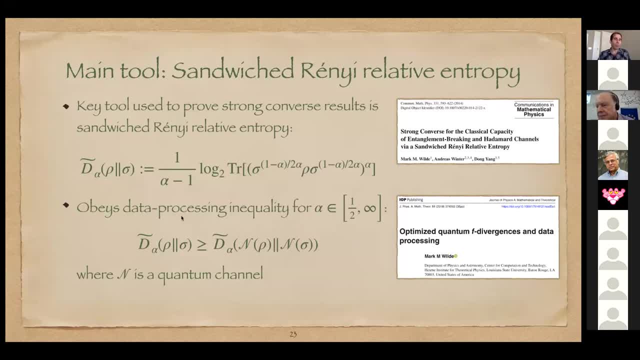 But you know when you're, when you're coming up with a distinguished ability measure, the main thing that you need is data processing, And so that plays a core result in proving these upper bounds Kinds of statements. Let me skip this. 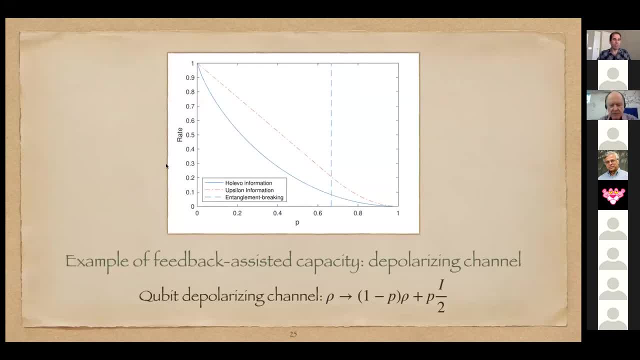 So In this paper, with short at all, We evaluated our upper bounds For the depolarizing change. So The, The, The, The, The polarizing channel for the feedback, assist, the capacity, And this. this is the best known upper bound. 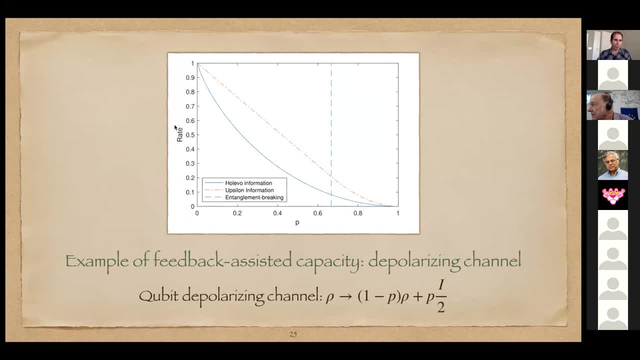 So far Okay, The blue line. So what we're looking at is rate versus the polarizing parameter, The qubit depolarizing channel. Either the qubit gets through with probability one minus P or it gets completely Randomized with probability P. 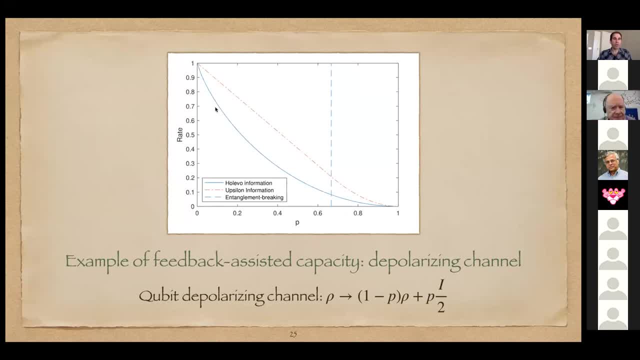 Okay, And this lower bounds, This blue line, is what you can see. This is what we can achieve At the level information rate, And it's actually known for this channel That, if there's not feedback, this is the capacity Okay. 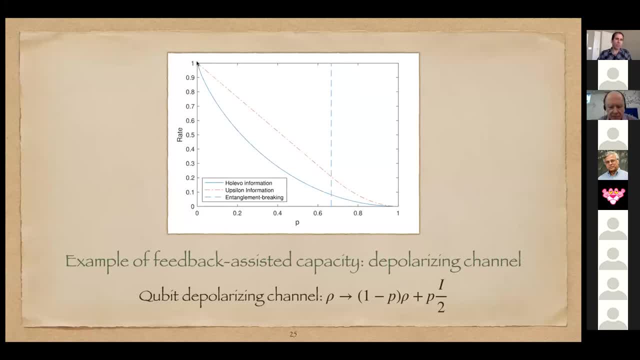 And with our new upper bounds for the feedback, assist, the capacity, This, this is what we find, And so you see there's a significant gap. Still a lot of work to be done to improve this. This line here is where the 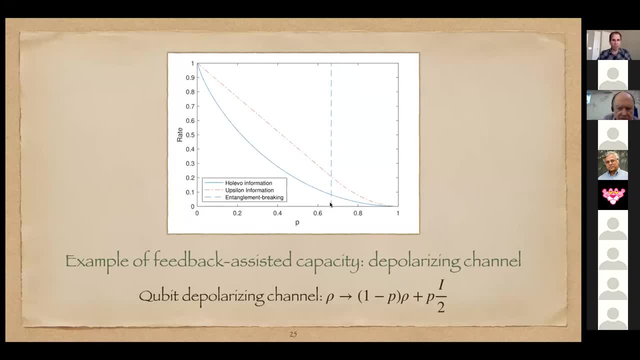 the polarizing channel becomes entanglement breaking, And so we know, beyond this point, the blue line is actually equal to the feedback, assist, the capacity, And we don't expect there to be like a large discontinuity In the capacity. So- or at least you know in a neighborhood around here- 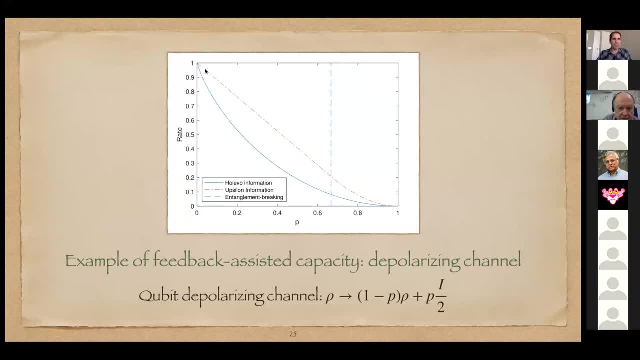 So my, my bed. Well, I don't know. I don't know Since they conjecture, but if I was forced to put down money, I think that we could bring the upper bound all the way down to the lower grounds. 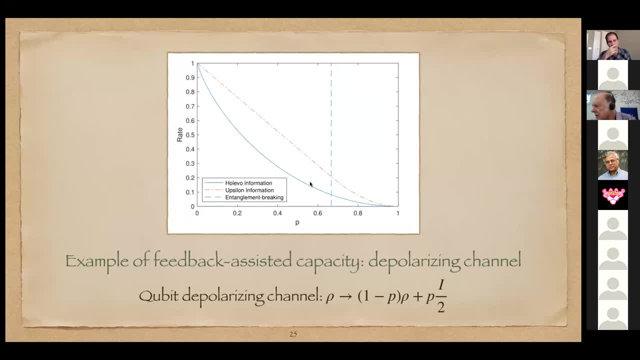 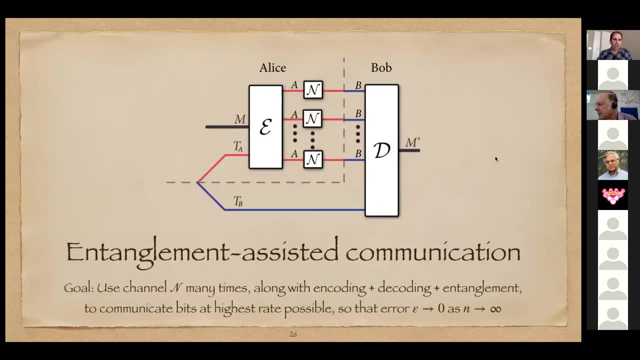 And just more work needs to be done, But It's an interesting challenge for people interested in quantum Shannon. All right, I'm running out. I'm basically out of time. I should leave enough time for questions. Let me just start. 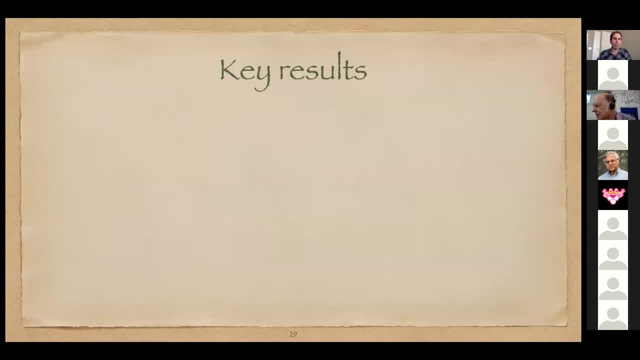 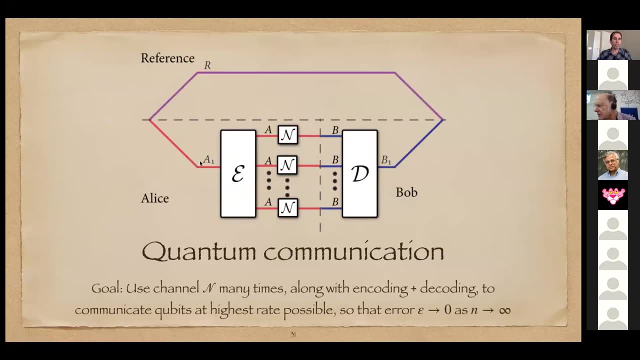 Flipping through and seeing it If I see anything interesting to mention. This is the diagram we think about for quantum communication. If Alice wants to transmit cubits to Bob And we have a notion of quantum capacity, How does entanglement play a role there? 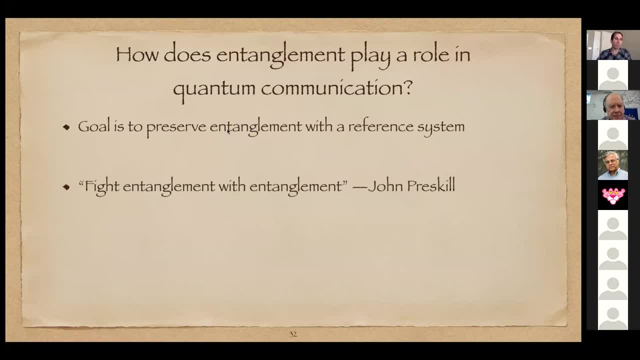 The goal is. you can think of the goal of quantum communication as being to preserve entanglement with a reference system. There's this famous quote of John Presco Where he's saying: we can fight entanglement with entanglement. What does this mean? 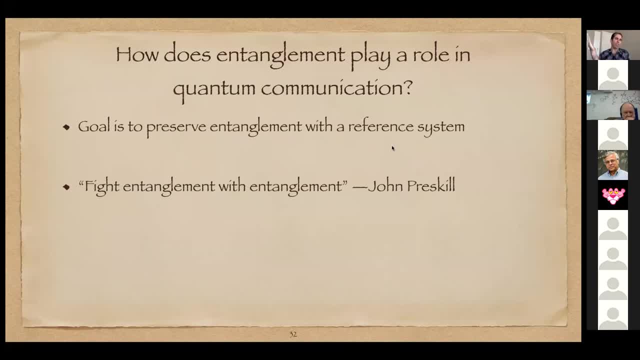 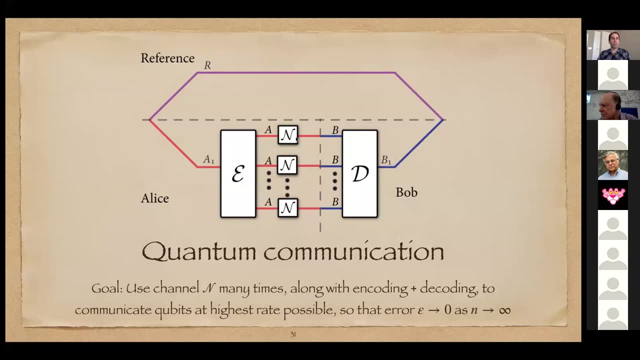 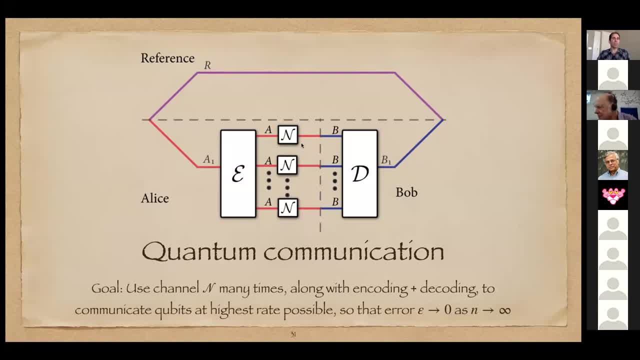 Prevents you from Sending information perfectly. And what we do is We fight that entanglement with the environment By entangling the quantum information Over many cubits, Okay, Or many modes in the apple, In the optical case. 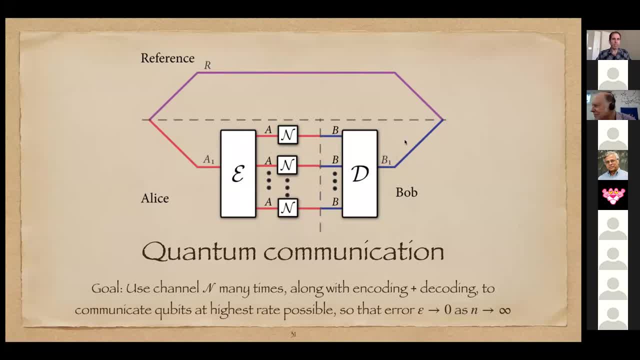 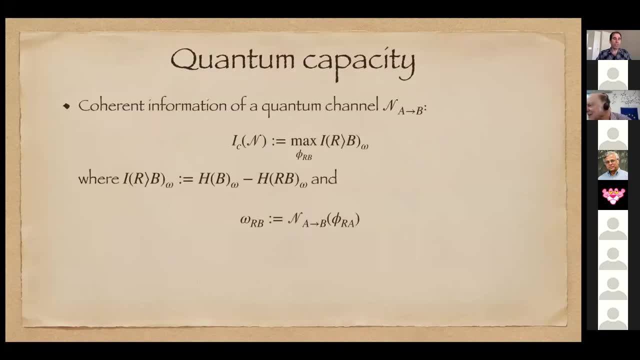 And so you're using this entanglement of the code words to fight the entanglement with the environment. It's an interesting way to think about it. Okay, And Quantum capacity? There's a formula for it In terms of this coherent information of the channel. 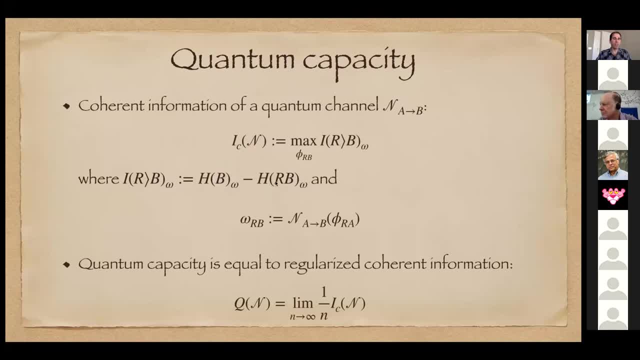 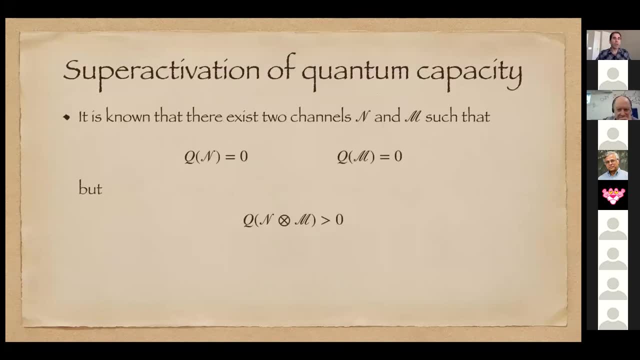 It's defined as this entropy difference, And there's still loads of questions about quantum capacity. Okay, And if you haven't heard of it before, this is a very big deal, Very interesting. This was found by Grantsmith and John yard. 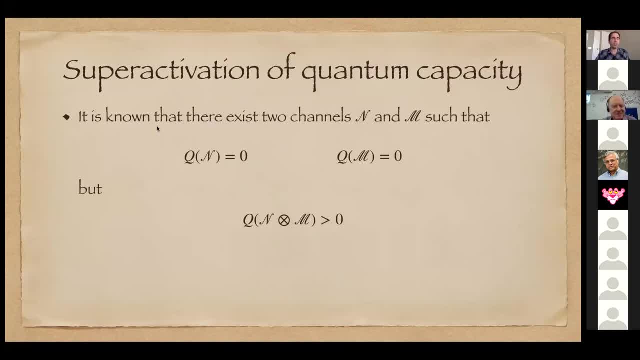 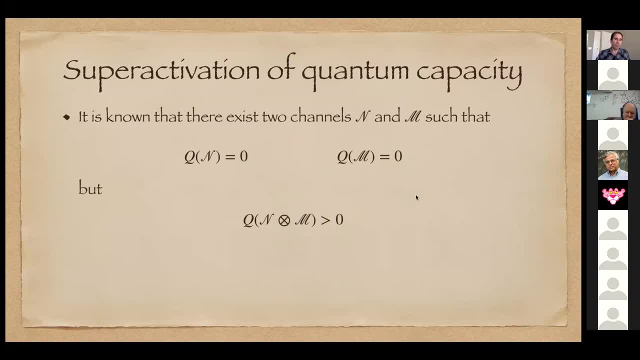 And so the We can see that they're all together And the the quantum capacity is is strictly greater than zero, And Smith and yard actually did work after the original work to show that there exists Examples of Gaussian channels, Quantum optical channels. 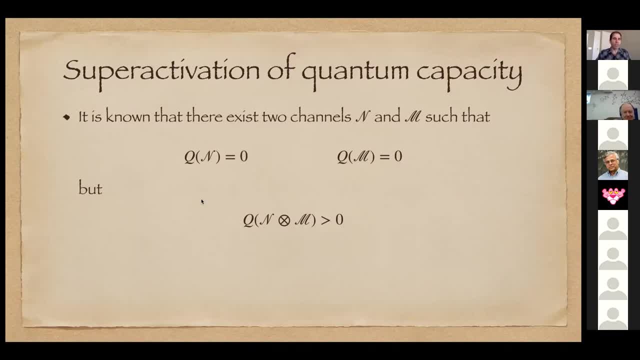 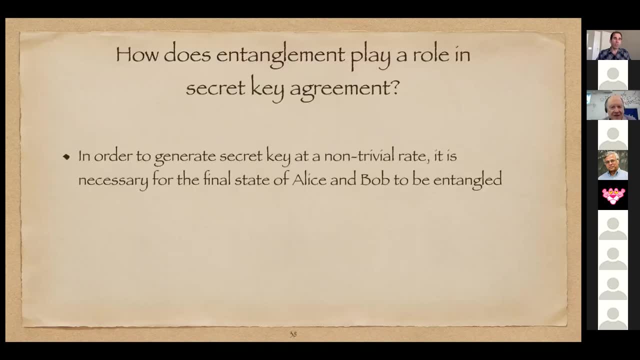 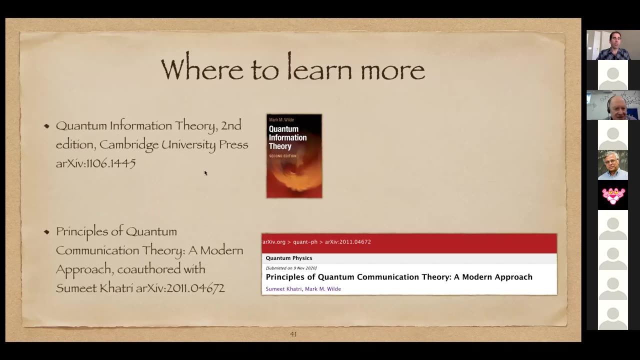 For which this effect holds, And so You know, possibly you could see this effect in the wild. So that's interesting. I'm just going to skip to the end because it's pretty much time. Oh, I should plug these books that I wrote. This is one that's been used a lot. 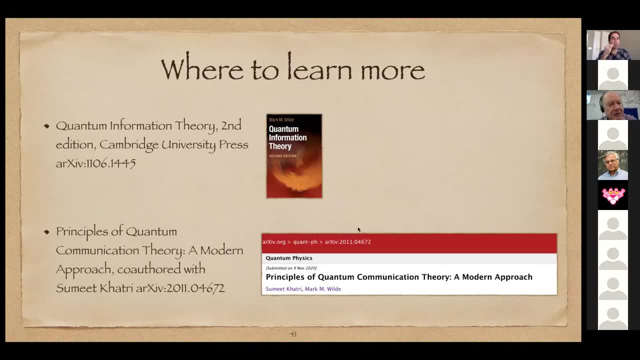 I'm going to be teaching this semester quantum information at LSU, but I'm going to try an experiment and use this new book that I wrote with Sumit. So this book captures everything until around 2011-2012.. And then this book captures many of the activities that were going on in quantum information during the past decade. 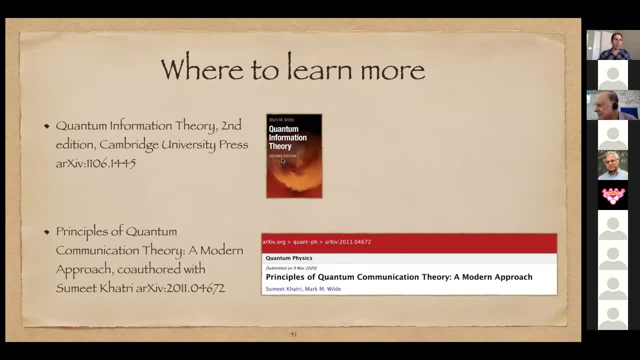 And the approach in this book is to think in terms of von Neumann, entropy and typical subspaces. Those are like very core concepts. The approach in this book is to think in terms of Renyi relativization. So you're taking the relative entropies, formulating all the problems of quantum Shannon theory in terms of a one-shot task. or if you're considering feedback assisted tasks like that would be an n-shot task. 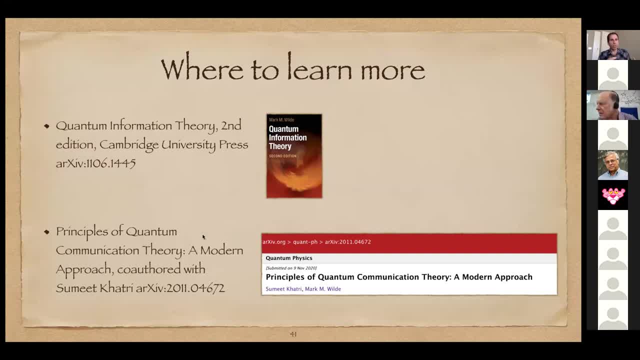 And then you use asymptotics of the one-shot quantities and the interplay of those with Renyi relative entropies to get the capacity results. And so this is- you know, we use this phrase- modern approach. And so this is, you know, we use this phrase- modern approach. 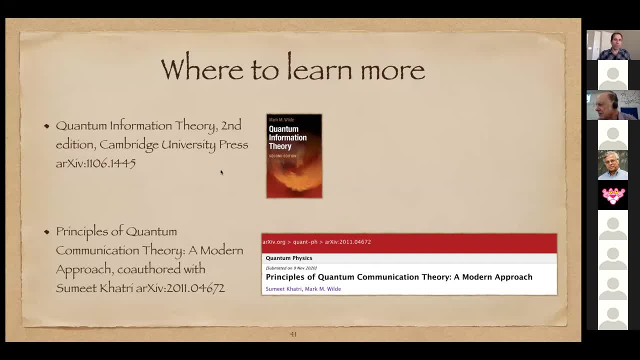 And so this is. you know, we use this phrase modern approach. Eventually that will no longer be modern, but whatever, we chose that title to make some distinction between what we're doing here and what was going on in this book. And then also I gave lectures. 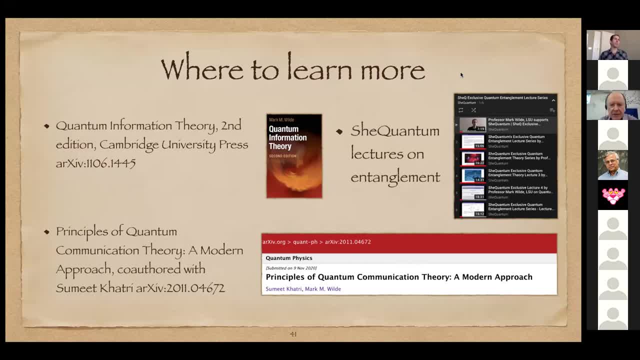 There's an individual, her name is Nithyasri. She's made this organization called SheQuan, to support women pursuing studies in quantum information. And to support that effort, I gave these lectures. And to support that effort, I gave these lectures. 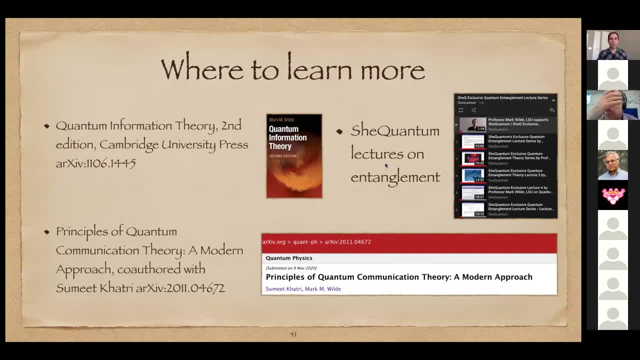 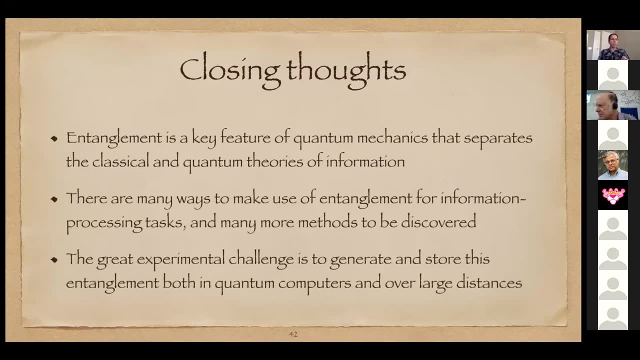 And to support that effort, I gave these lectures on entanglement that can be found on YouTube, And so you can find more there. All right, final thoughts. Entanglement is extremely important. It really shows a separation between classical and quantum. 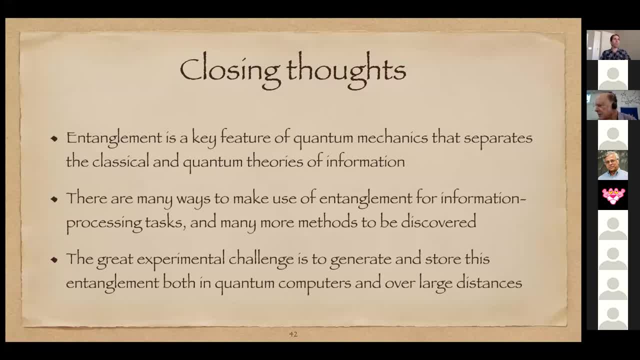 And what did I talk about? I talked about transmitting classical information. I talked about feedback-assisted classical communication. We talked about how entanglement played a role there, a role there. we talked about quantum communication. briefly, i skipped over entanglement assisted. 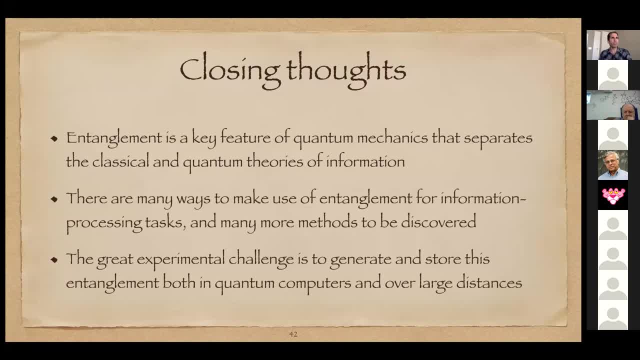 capacity. that's a very interesting capacity that could probably deserve a lecture all on its own. but that's a generalization of super dense coding and in that scenario you really um have the the most beautiful results, i would say, where there's a formula, the quantum mutual information of a 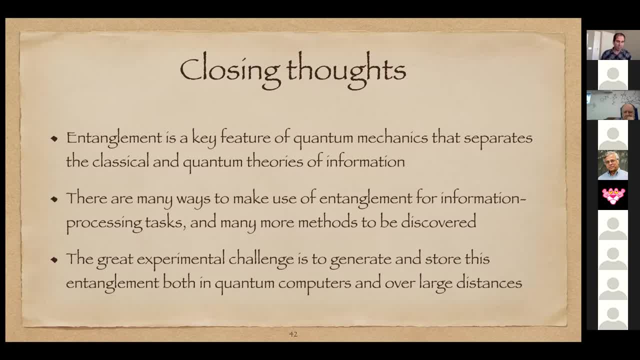 channel is the capacity, and i would say that's the the fully quantum generalization of shannon's results about capacity of classical channels. um, our field is so rich with so many different things that can be done. i suspect that you know, over the next decade at least, there will still be. 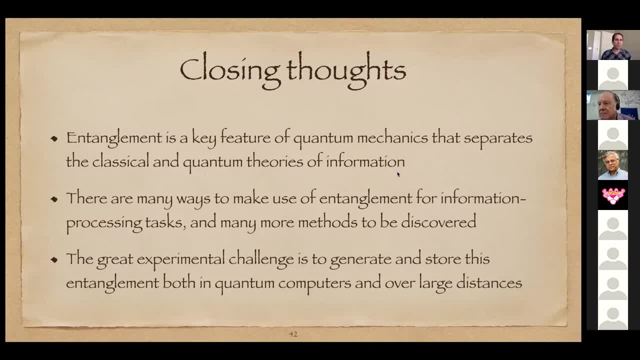 many interesting things to discover and find out about what can be done with entanglement um, and so i look forward to that. and you know, now we're seeing all these implementations. i mean nowadays you can actually log in and program quantum computers and they're all over the world. 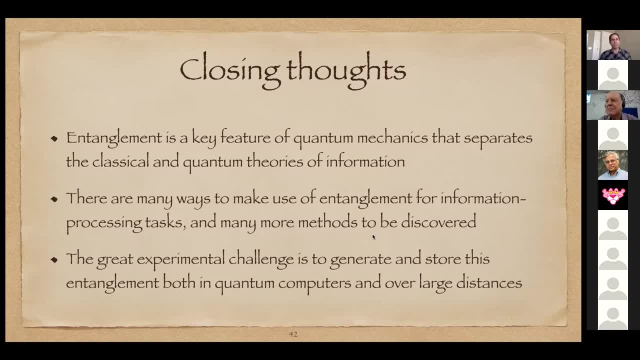 now. it's just really remarkable to think about it, and so the great challenge for experimentalists is to improve these devices where we're generating and storing entanglement, so that we can take advantage of all these great possibilities. and with that i'll stop, thank you. 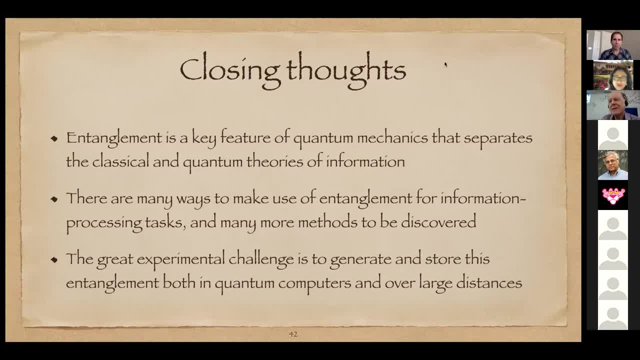 thanks a lot, mark, for that very nice, uh, very detailed overview. uh, so the floor is now open for questions. um, you can just raise hand or type, or, charlie, do you have any questions? because you're muted, just in case. uh, so charlie wrote in the. oh, i know, he wrote the definition. now it's a direct message. 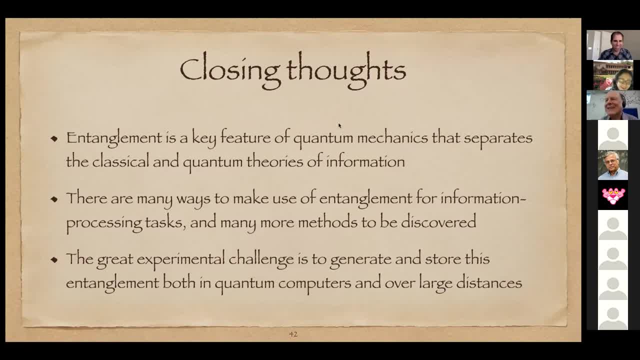 but i think it's very funny, so i'll just read it out. so he said: we'd like to say that shannon discovered an elegant formula for entanglement assisted capacity, which, for classical channels, happens to be equal to the shannon capacity, right? so ringraj has raised hand. ringraj, yeah, do you want to unmute and ask? 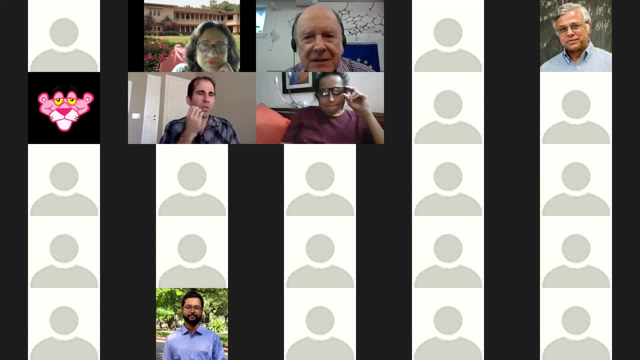 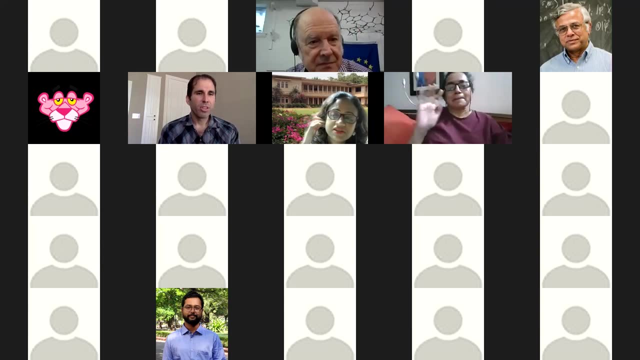 it to me. sorry, where is my sorry ringerage? uh, you have your hand raised. yeah, but i think he's trying to um get his audio to work. okay, so while ringer does that, if anyone else wants to say something, i think there's a question in the chat. what is renee relative? 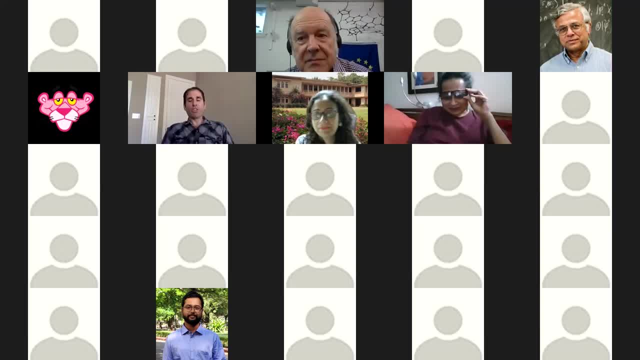 maybe you answer the chat one: what is renee? what is rennie? relative entropy: okay, great question. um, sorry that i was a bit fast with that. i might have been in the chat room, but i'll let you know. might have been a bit presumptuous. um, so we use relative entropy to quantify the distinguishability. 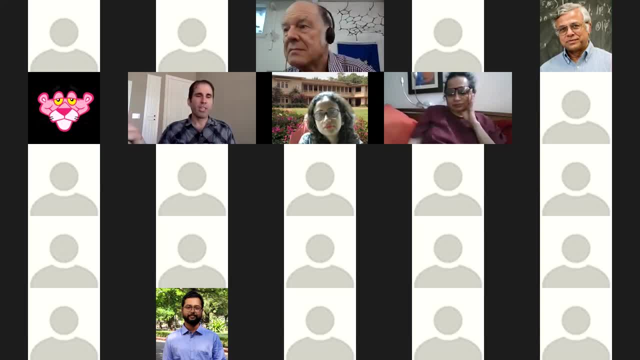 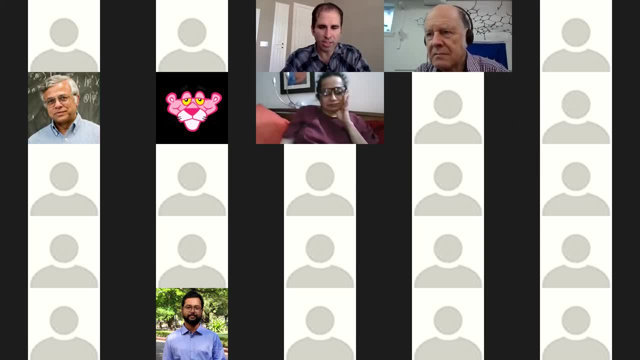 between quantum states. okay, that's. that's a famous formula and, um, you know, often i'll write in the chat like it looks like um minus log sigma. okay, oh, i wrote a direct message to charlotte. let me um, all right, someone's making laws. i'm an audible. okay, one second, give me a second. i'm trying to answer the question, so, uh, relative. 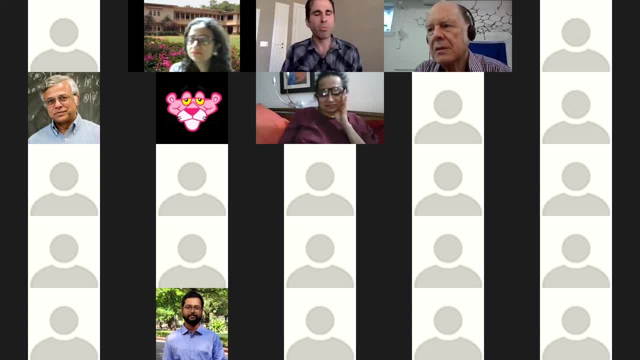 entropy is this? you've probably seen this before if you studied quantum information. this formula a trace of row log, row right and minus log sigma, so that's used as a measure of distinguishability between two quorum states and it has it has a distinct operational meaning. 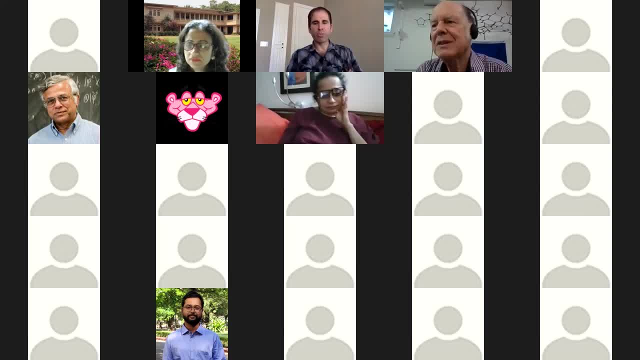 and then you can also think of it as a parent entropy, because, um you, you can, you can derive, uh, von neumann entropy from it as a special case. you can get conditional entropy as entropy as a special case. you can get mutual information as a special case. Okay, Then. 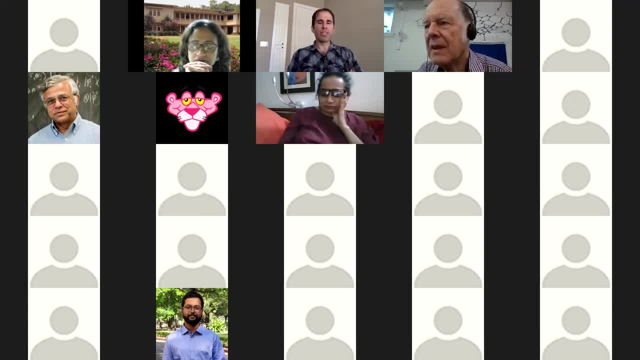 you know, you can formulate certain axioms for what it means for a quantity to be a relative entropy- And I forget who did this in the classical case- but you formulate certain axioms and you get a unique function, which is the relative entropy. If you then drop one of those, 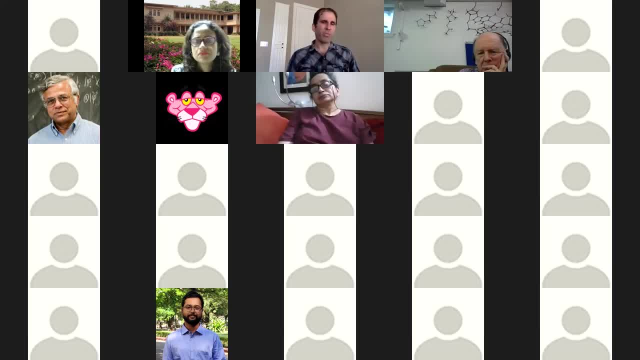 axioms, you get Renyi, relative entropy, And that's what Renyi did from kind of a purely mathematically inquisitive perspective in 1961.. And then subsequently people found operational meaning for Renyi relative entropy in terms of protocols, like refined versions of capacity. 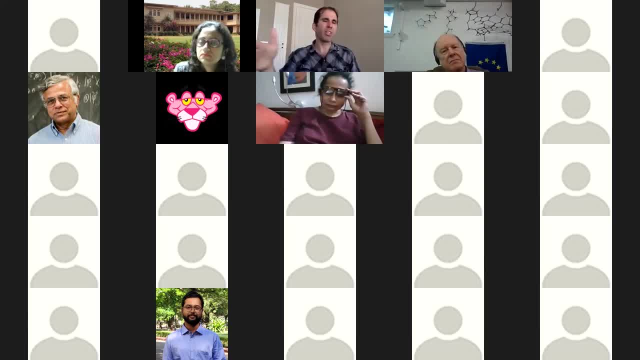 questions. So you're considering like how fast the error decays as a function of the number of channel uses, some question like that Right, And so that that became quite ubiquitous in classical information theory And then of course in quantum. we always looked at classical for guidance. 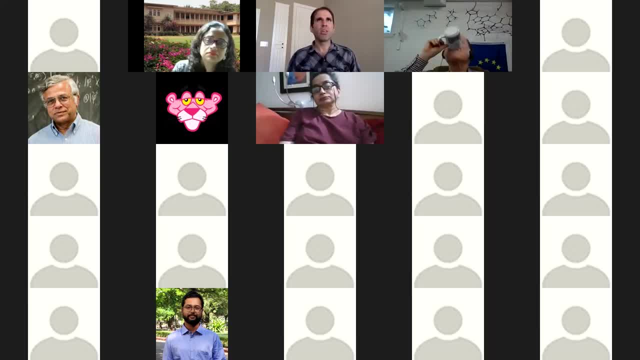 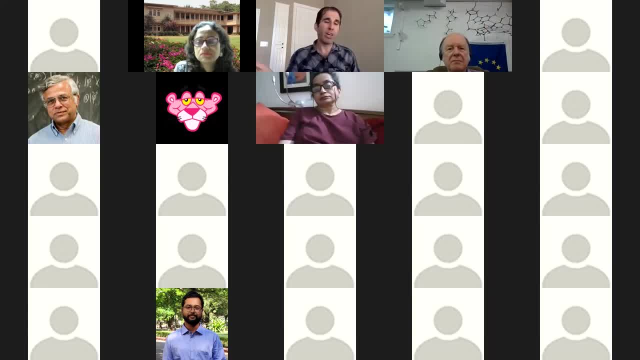 operational meaning in quantum Shannon theory, And you can find a lot of that in our, in our book with Sumit, you know. so you can, you can look in there, All right. So there was a direct question from me, There was a direct message from Khalid Benjamin to me. Why, in the CHSH game, 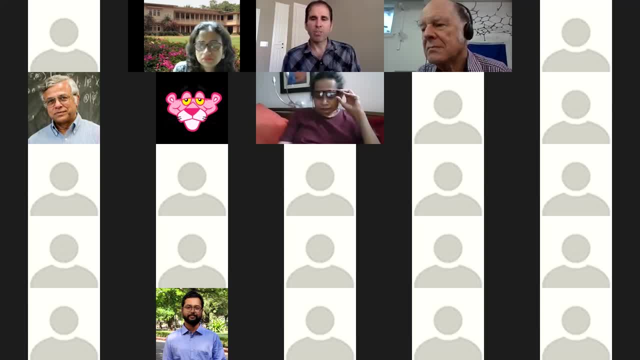 the winning probability is not a hundred percent for quantum. So that's the first question, And it's a great question that was answered by Boris Searleson- I forget what year, but there's something called Searleson bounds, where you can actually through a sequence. 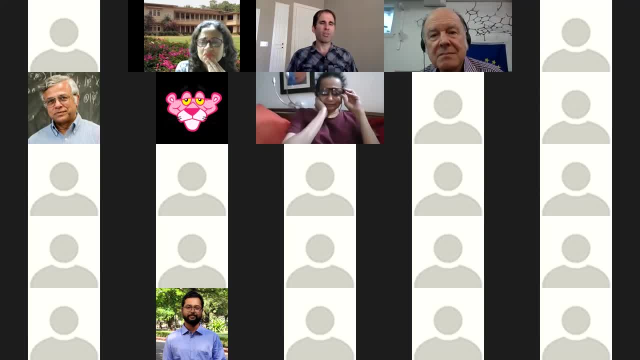 through a sequence of: sorry, there's a scratching noise. I'm going to. I'm suspecting it's in my garage, So I'm going to, maybe if someone could. Yeah, Yeah, If you don't mind. Okay, So there's something called. 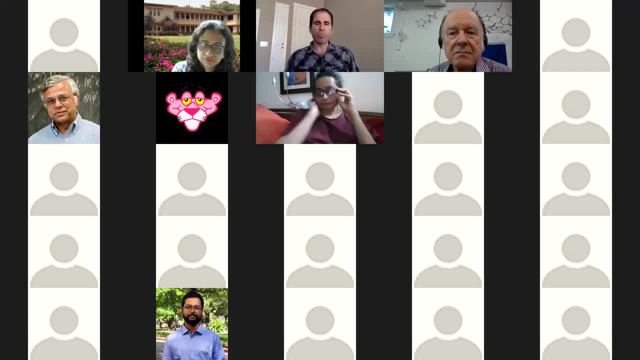 the Searleson bounds. through a sequence of logical steps, you can prove that the winning probability cannot exceed 85%. This, this cosine, squared pi over eight. Okay, And there's a, there's a. the follow-up question is: is there something beyond quantum entanglement? 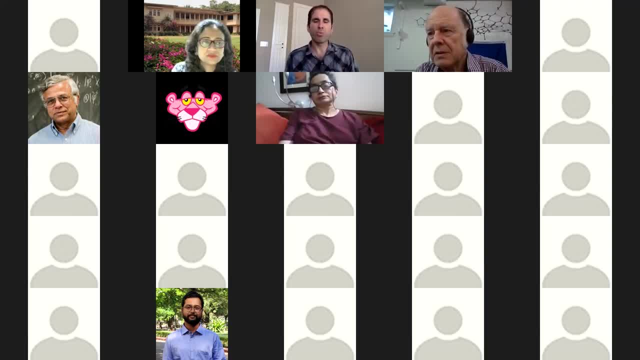 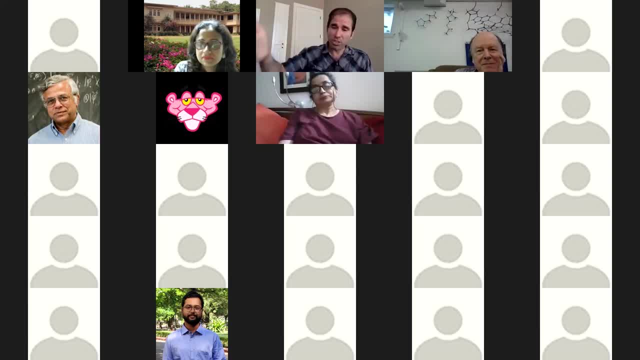 Rolick They came up with. they were, they were interested in this very question. I think it was the early nineties, I forget exactly. but they they came up with something called the PR box, which is kind of a fictitious correlation that two parties could share. that 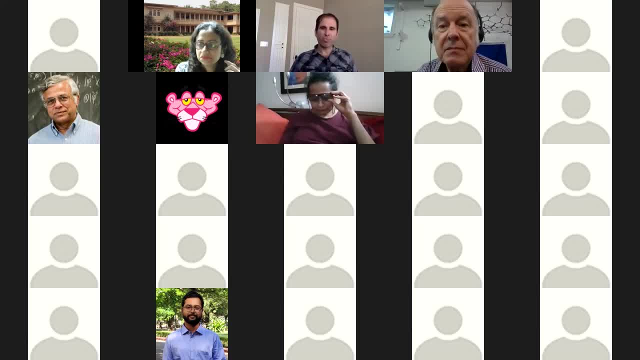 wins the game with a hundred percent. Okay, And it's called non-signaling correlations And those, those go beyond quantum, but it's not clear that we can realize these correlations in practice. So, but there's been a lot of foundation work. There's been a lot of work in foundations of quantum mechanics related. 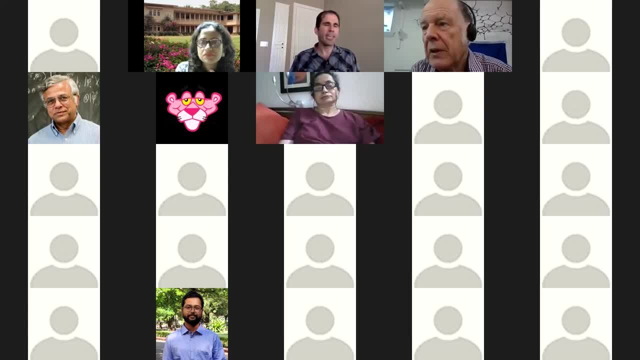 to this PR box. Yeah, And the idea of non-signaling correlations that comes up a lot Like I showed that capacity bounds for feedback assisted capacity to derive that bounds. We use the concept of non-signaling correlations because the constraints corresponding to non-signaling correlations, they can be expressed as semi-definite constraints And 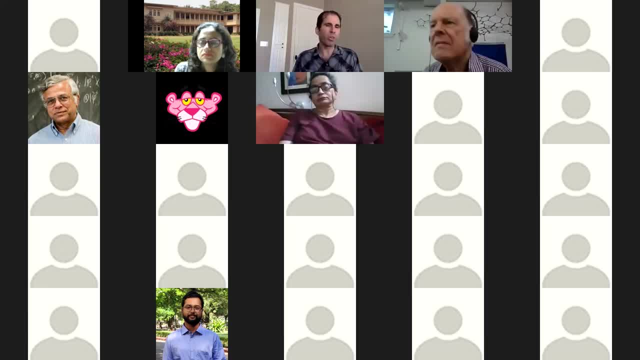 then typically, if things are semi-definite constraints, they can be incorporated into semi-definite programs which can be efficiently evaluated. Okay, So in the chat Charlie said how Renyi entropies are family of quantities, generalizing entropy. 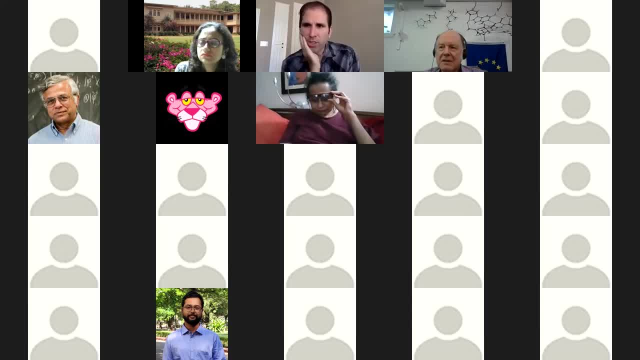 Dia asked a direct question. Should we consider these entropies as a measure of information only? It's also the uncertainty about a system before making measurements of the system. Yes, you can think of it. Indeed, there there measures of uncertainty, and you know entropy. 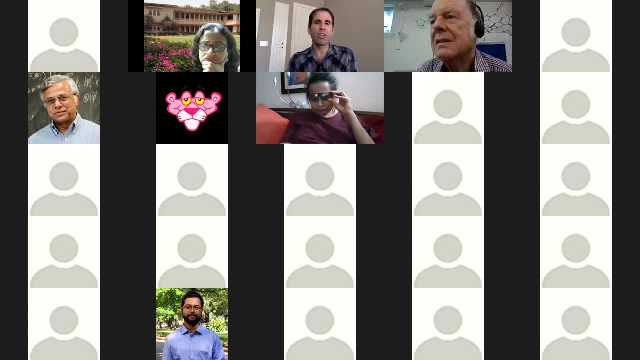 there's a famous story how like you know Shannon was. I think it's just kind of it might be made up, I don't know, but it's very famous and passed along where Shannon was looking for a name for this quantity had come up with and went to von Neumann and asked: 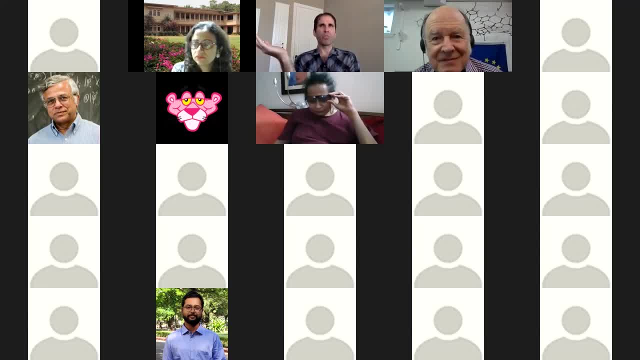 them: what should I call it? And von Neumann said: oh, you should call it entropy, for two reasons: because I invented it 25 years ago And if you use that, you're going to get a lot of information, And so you know, I think that's a really good question And I think 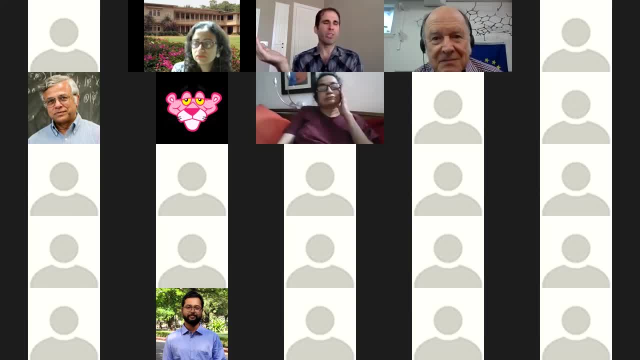 that's a really good question. I think that's a really good question. And I think that's a really good question. I think that's a really good question. I think that's a really good question. I say, if you use that name, entropy, you'll always have an advantage in a debate because 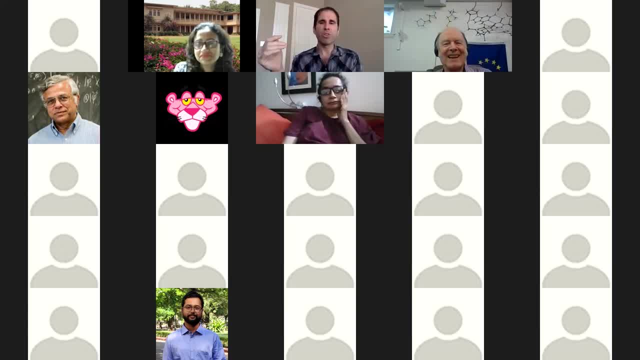 no one knows what it means, And so von Neumann had used entropy in the context of thermodynamics. you know quantum statistical mechanics And you know there it's understood as a measure of uncertainty. Okay, Charlie made the comment. Prophesco showed if you could win the game with a hundred percent. 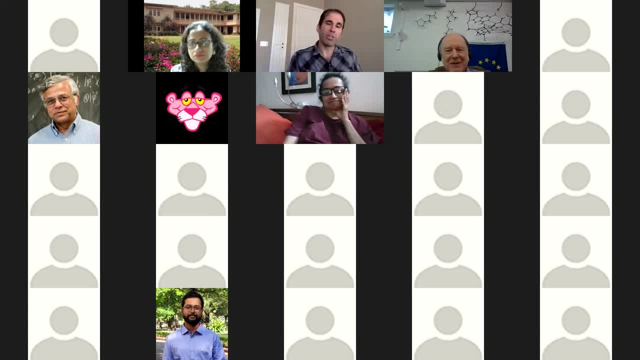 you can communicate fast and the speed of light. Okay, That's very good to know, Thank you. So then these PR boxes should be impossible physically. Runak Chatterjee, I don't know how to say that properly, sorry. How is the CHSH game important to security aspects? 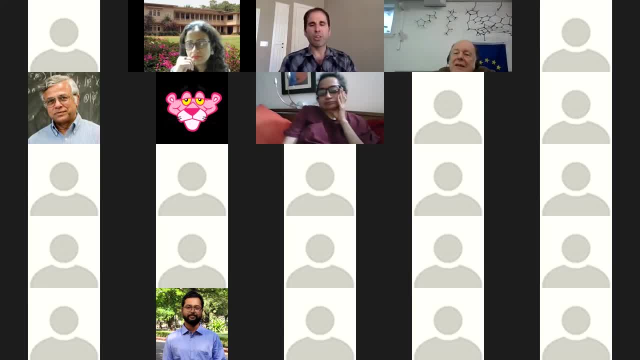 in quantum communications. So that's what I was talking about on that slide: how you use the CHSH game to test whether Alice and Bob truly have entanglement, because there's like a converse statement known that if they're winning the CHSH game with probability close to 85%, 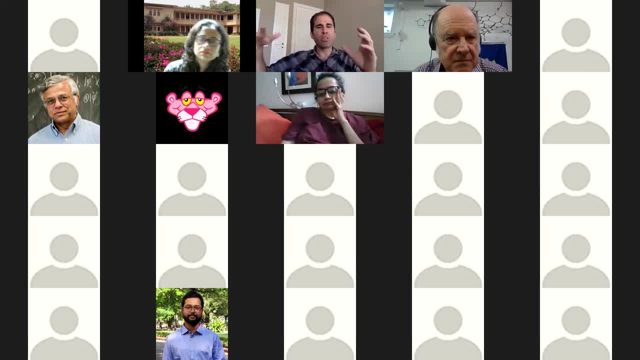 then the only possibility is for them to be using a strategy that wins the CHSH game. It's kind of like a faithfulness statement. So the states that they share will be close to maximum entangled states, And so Then, if they share something close to maximum entangled, 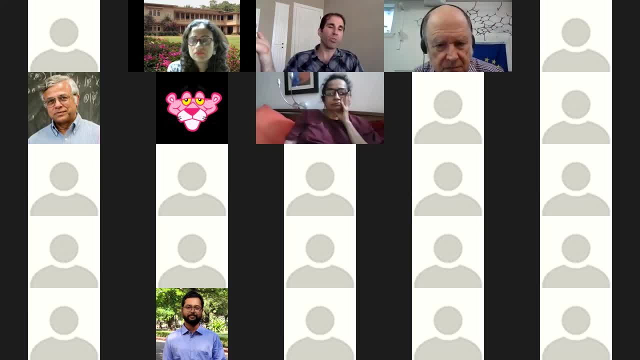 they can distill from that something that's close to a secret key. Does it help to find some bounds that can help us to detect Eve? Yes, that's exactly what it's used for. Okay, You mentioned about. This is from Usha Devi. 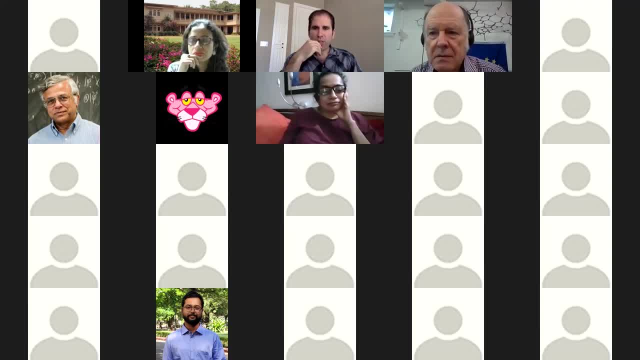 You mentioned about quantum reading, where the figure of merit is the quantum Chernoff bounds. I don't know if I actually mentioned about it, but quantum reading is a Very interesting topic that deserves further study. You can formulate quantum reading as a capacity problem. 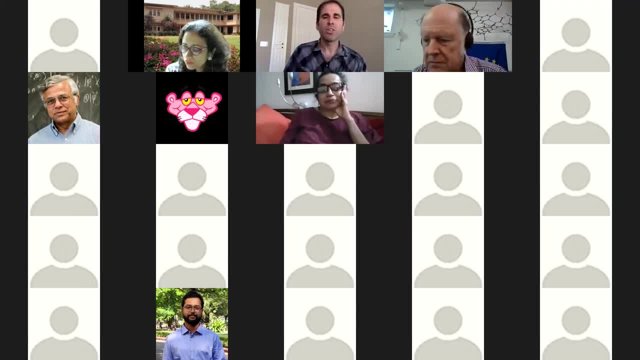 My co-author, former student Siddharth Das, who was here at LSU. we wrote a paper about quantum reading capacity where we defined what I think is the most natural definition of quantum reading capacity. So the question is in this connection. 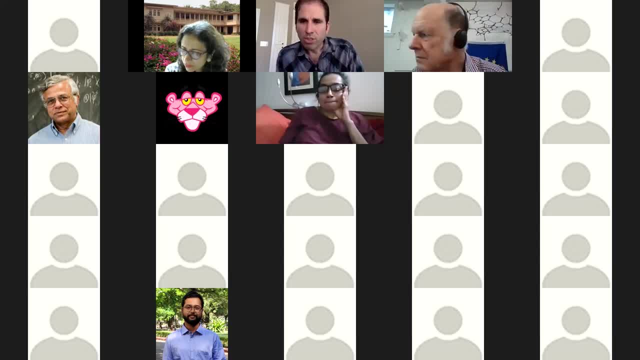 I want to ask the following: Entanglement breaking channels, too, fare well when entangled, when using entangled breaking channels too, entangled states versus unentangled states. But when it comes to classical capacity, entangled breaking channels do not fare well. 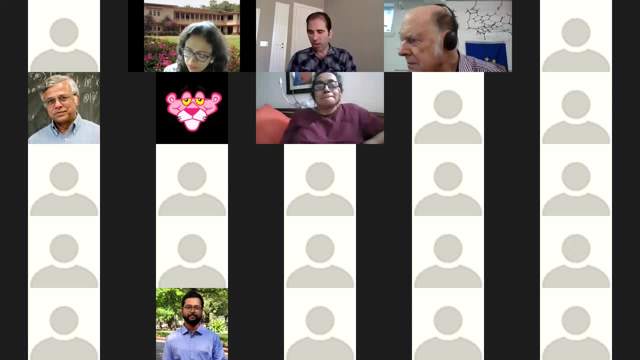 Can you comment on this? Yeah, so this is a great question. Quantum reading is more like entanglement assisted capacity. okay, So entanglement assisted capacity. you're allowed to use this pre-shared entanglement to communicate between Alice and Bob. 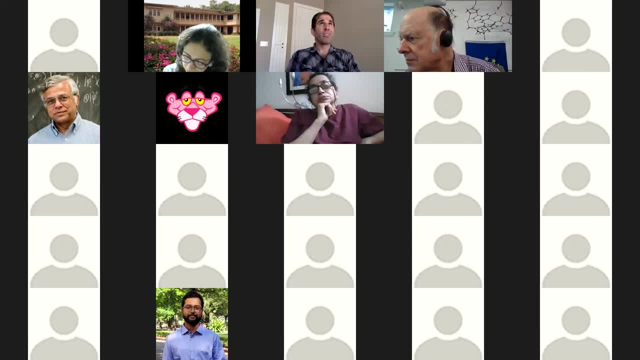 The way you can think about quantum reading and the relation to entanglement assisted capacity is this: So in entanglement assisted capacity, Alice and Bob are in different locations and they share entanglement beforehand And then Alice can encode, like in superdense coding. 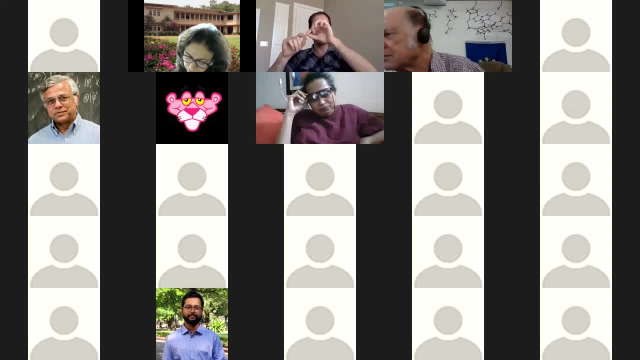 Alice can encode a message into her share and transmit it to Bob. Quantum reading is more like what's called quantum illumination, So that's something that Seth Lloyd invented. So there, Alice prepares an entangled state locally, sends one share over a channel to Bob. 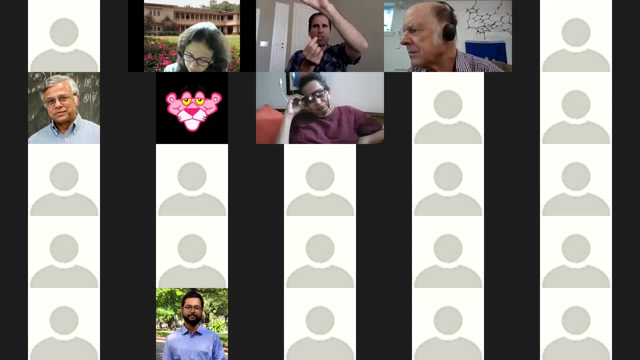 who then encodes something onto that share of the entanglement and sends it back to Alice, And then Alice does a joint measurement right. And so that's the connection between these concepts, And it's known that the entanglement assisted capacity. 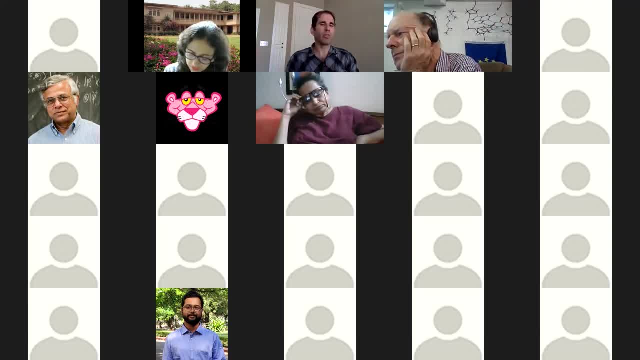 of an entanglement breaking channel can be larger than its unassisted capacity, right? So like there's all kinds of channels for which that's known and entanglement breaking ones like thermal channels, et cetera. So that's the reason. 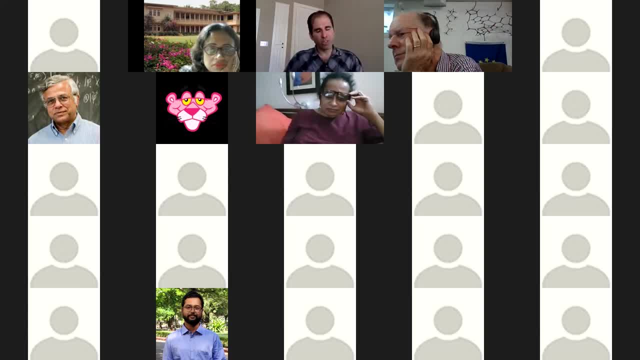 And the way that this is explained in the context of quantum illumination is that, indeed, there's a lot of things that can be done. One of them is that, indeed, with an entanglement, breaking channel, the state that comes back is separable. 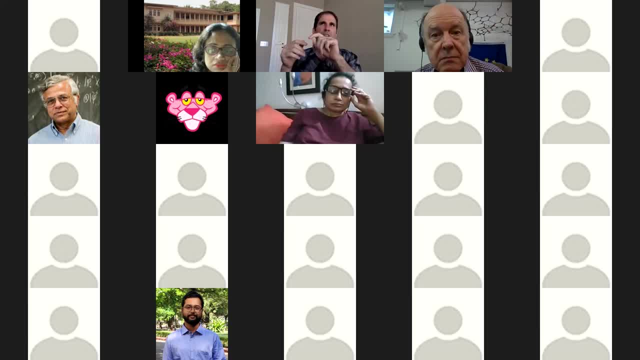 but the correlations in the state are larger than those that you could have had if you would have used the separable state to begin with. Okay, So that's a way to think about it. That's a very interesting question, And I think quantum reading capacity deserves further study. 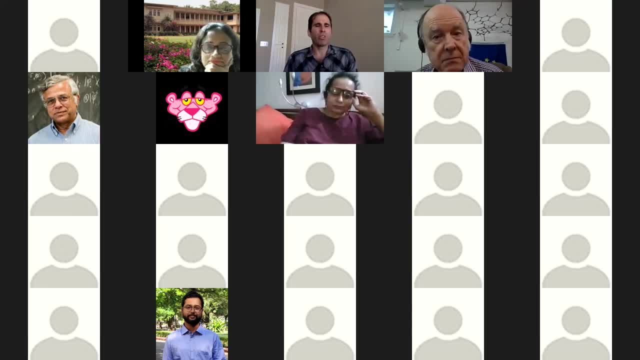 Like it's not known, various bounds and we have projects going on. It's hard to figure out upper bounds for quantum reading capacity. Okay, There's a question from Rengaraj LMU. So when designing a polar decoder for classical error correction? 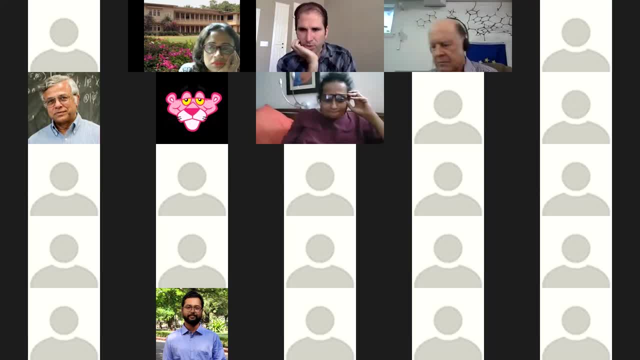 the frame error rate is slightly higher than LDPC codes. Please comment on this. I don't know What exactly is meant by frame error rate, Like for the whole block. So okay, It could be that for okay. I think the question is this. 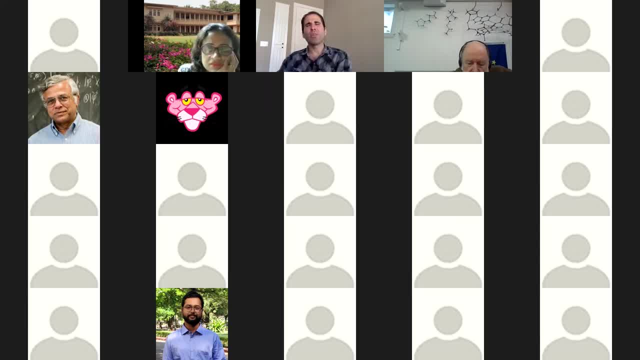 like it could be for a given block size. the frame error rate for LDPC codes is in practice found to be lower than that for polar codes. But you know, the key insight of our icon was that as the block size gets larger and larger, 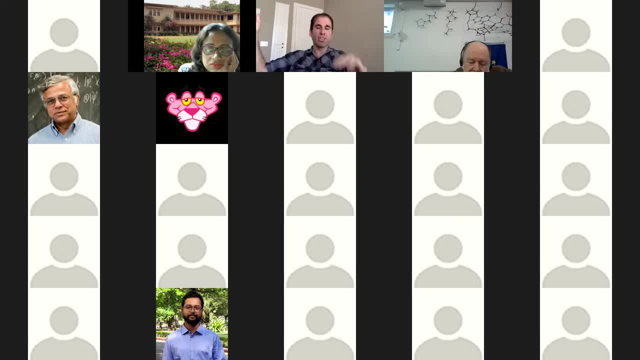 the frame error rate can be much higher. The frame error rate can be made to go to zero while achieving capacity. So Archon's achievement was monumental. You know, like Shannon in 1948 set out this question of designing error correction codes that achieve the capacity. 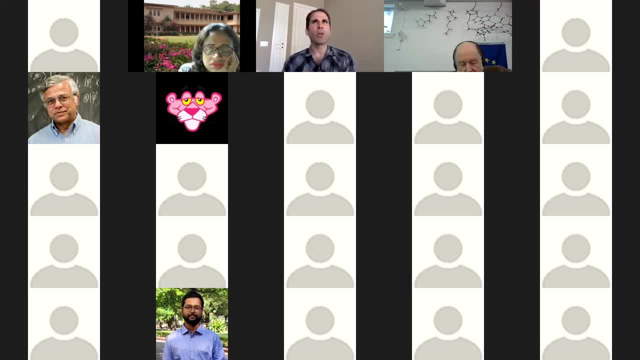 And for years and years and years, people tried all kinds of things. And then there were breakthroughs in the 90s where they could show that, like turbo codes appear to be achieving capacity. right, But there was no proof of it. And then there was LDPC codes. 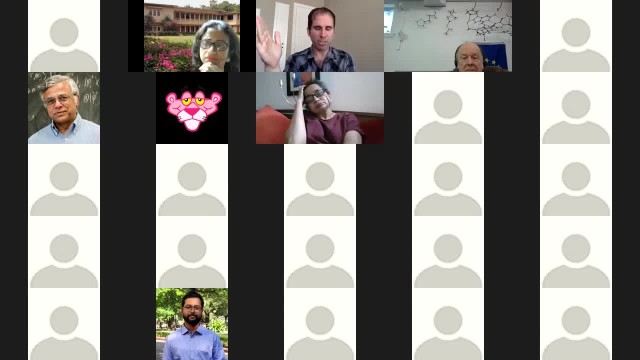 and then people showed numerically: oh, they appear to be achieving capacity. Archon in his paper- I believe it was 2007,. proved it, You know. he had a mathematical proof that, oh, there are these fossil codes and they achieve capacity. 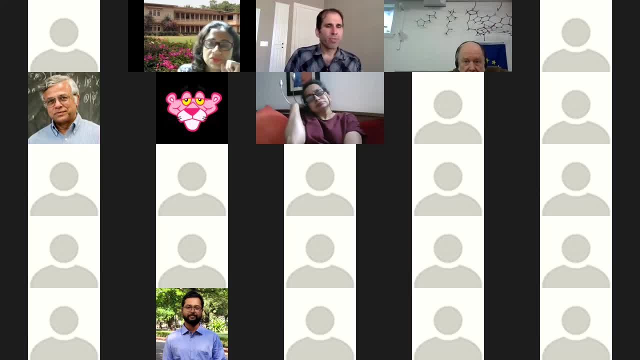 So sorry, Mark, how are you doing with time? I mean, you have- I'm fine over here. I have to leave in about 15 minutes if y'all are pressed for time. So we have one more question in the chat. 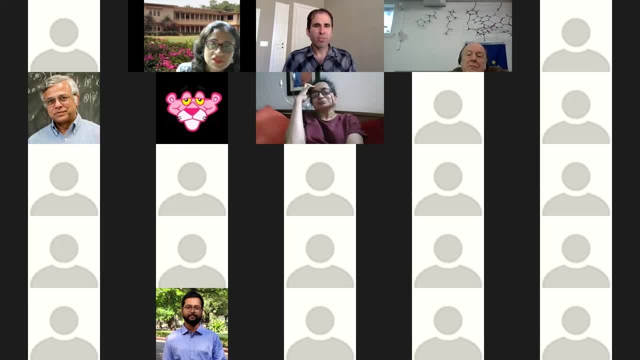 And I think we should also see if Professor Holm actually wanted to ask something, because he had raised his hand, which is now not raised anymore. So we- I'm happy to have all these questions frankly when I get to talk. Okay, he has actually written in the chat. 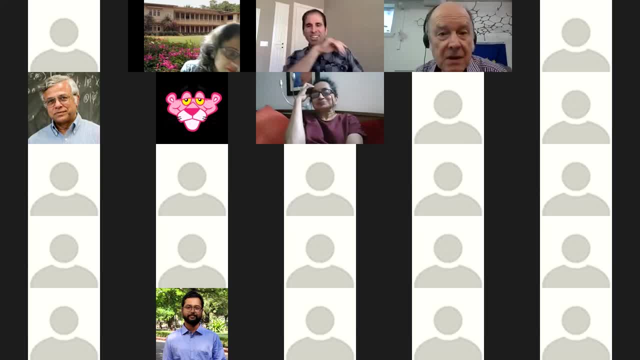 So then, yeah, you can just keep reading the chat. then I think both of you, yeah, please. So I wanted to continue a bit with polar codes. Polar codes are now used in present times in technology, So I believe that we're on 4G. 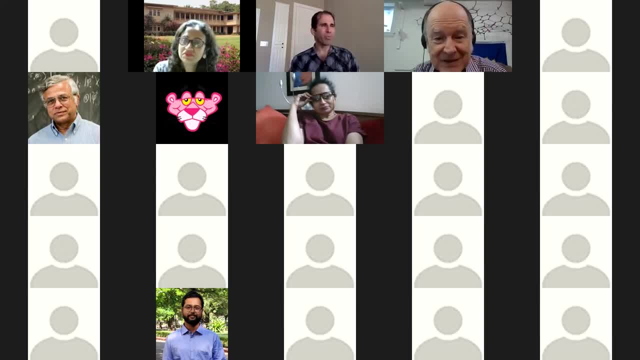 Am I correct or is it 5G? Anyway, they're used in present day technology And this issue of frame error rates. there's all kinds of ways that you can modify the original proposal of Archon to improve the practical performance. 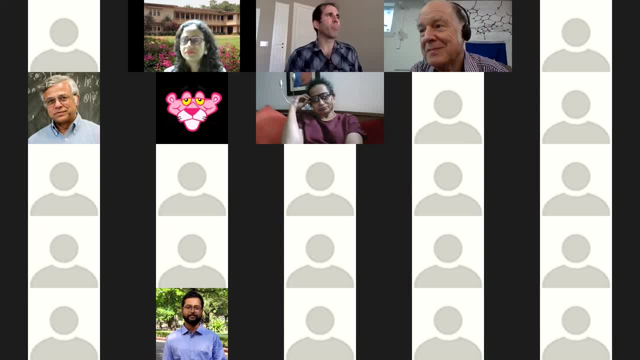 And so there's been all kinds of research about that, And then now those things are incorporated into the present-day technology. So you know, I think it'd be wonderful to study polar codes further. There has been a lot of work, but you know just this basic setting of communicating. 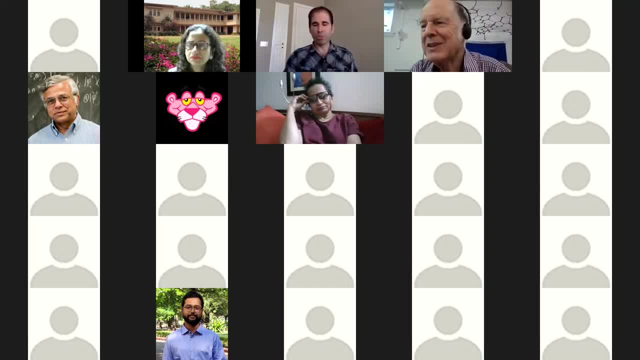 classical data over QAM channels. there's been only so much work. A former student, Kaushik Sethadrishan, and he's now a postdoc with Saikot and he'll be starting in Pittsburgh as a professor. So they used an ion trap quantum computer to try to test out the performance of 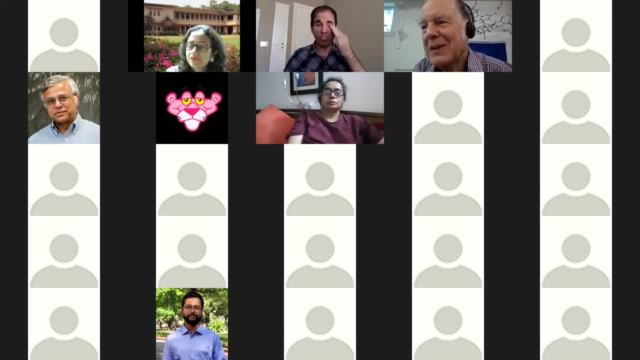 classical polar codes to try to show some quantum advantage, And so that was the latest thing on that topic. that I think was pretty interesting. Okay, PR box maximally violates information causality. Question from Indranil Can you kindly comment on? 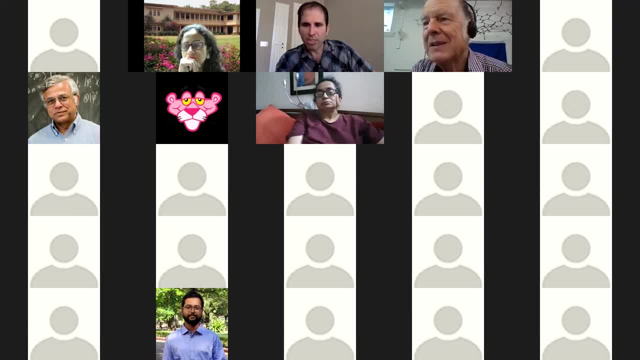 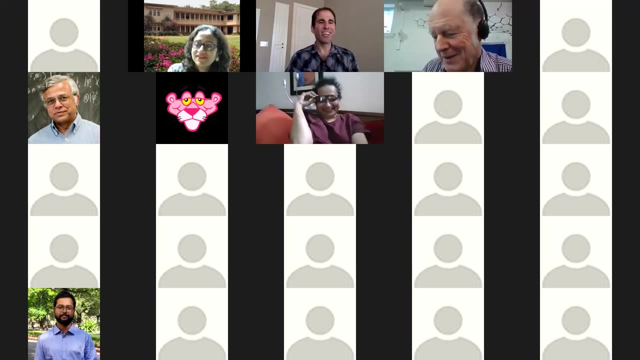 how indefinite causal order affects channel capacity. Recent updates in this context. Okay, Am I being recorded? Yes, Mark, So I guess I'll say on the record: I'm pretty skeptical about this whole topic of indefinite causal orders and channel capacity. Like you'll see, things like 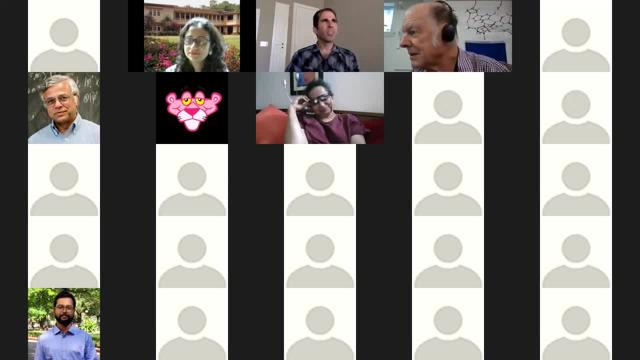 oh, you can send information at a non-trivial rate over a completely depolarizing channel right, which is like totally useless if somehow you have access to indefinite causal order. And so my main skepticism is like: yeah, it's certainly interesting mathematically. 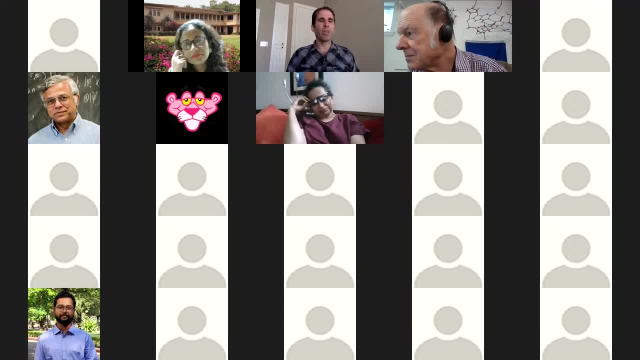 Can we see this in the wild, like in an experiment, right, Or not even in the wild, like experiment, Can we expect to see these effects come to fruition? And I'm very skeptical about the whole thing. It has made an impact on quantum gravity because, you know, in quantum gravity 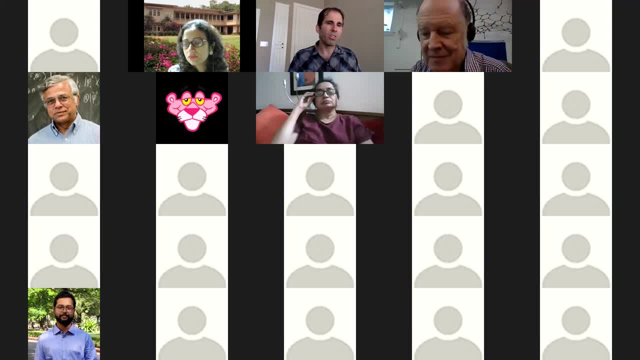 we could possibly expect to see superpositions of causal orders come into play. So I guess I don't have much to comment because I'm not immersed in the topic. The person to come to converse with about this and possibly invite, if you're interested to hear about it. 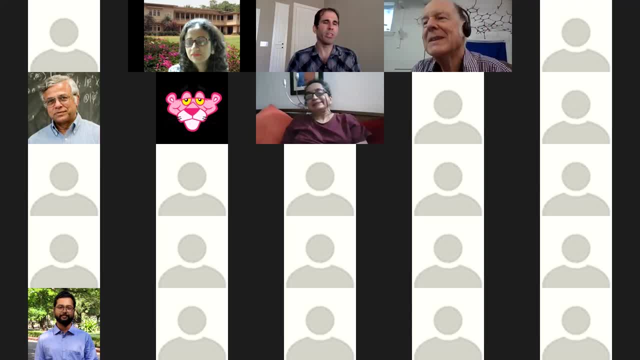 for a seminar is Giulio Chiarabella. I don't know if you've invited him already, but he's been really pushing this topic quite a bit and has quite a bit of research about it. I think it's very interesting from a theoretical perspective And you know all kinds of things. 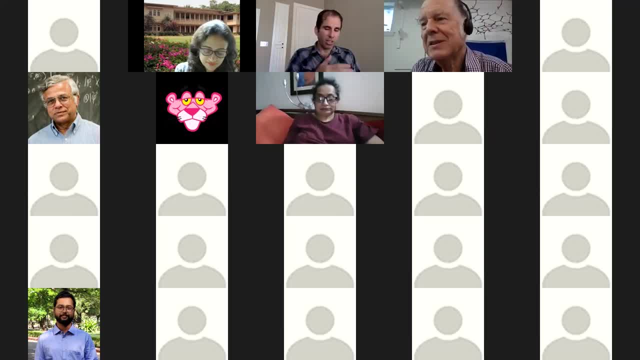 have been discussed and considered theoretically, like distinguishability of channels, you know, transmitting information over channels, classical quantum et cetera. And you know, I think Giulio has a grand plan of considering like a second quantized quantum Shannon theory where you could. 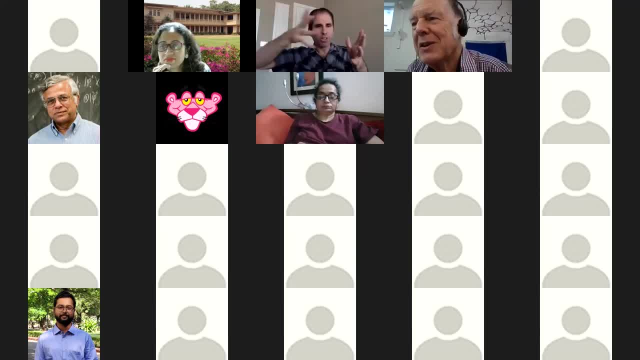 have like the timelines, like in all the diagrams I was showing you. these timelines are classical, right, But he wants to consider when the timelines can be quantum, you know superpositions of causal dynamics. Okay, So there was a comment of Dipankar: role of noisy channels in the 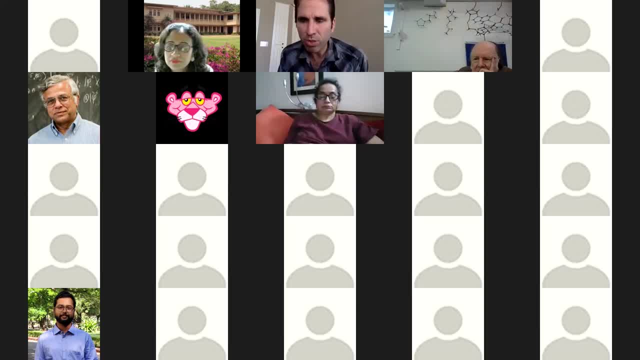 context of higher dimensional entanglement, say for bipartite qubits. What are the future interesting questions to study using the studies on noisy channels you mentioned? Okay, So for higher dimensional entanglement, bipartite qubits, there has been a lot of work. 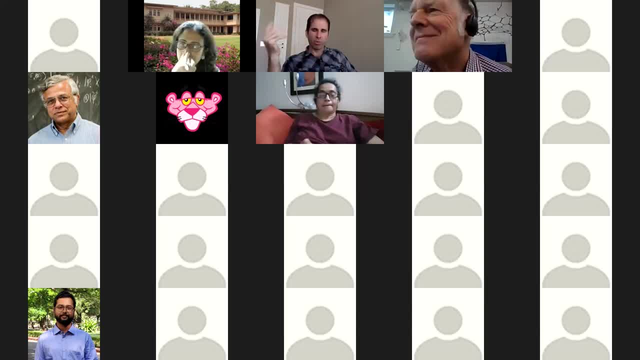 on computing entanglement measures. There's been a lot of work, and especially from scientists in India. You know, there's one measure that I think is very fascinating, and this is squashed entanglement. Okay, And so there's very few states on which we know how to evaluate squash. 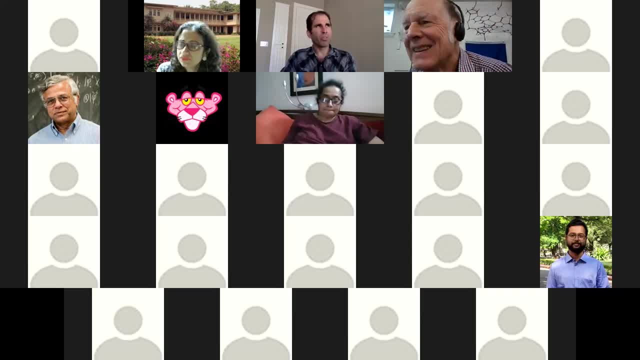 entanglement, And so if there were simply more developments on that topic, I would find that that an interesting. I think it's a useful entanglement measure Why It's an upper bounds on distillable entanglement. It's an upper bound on distalble secret key. 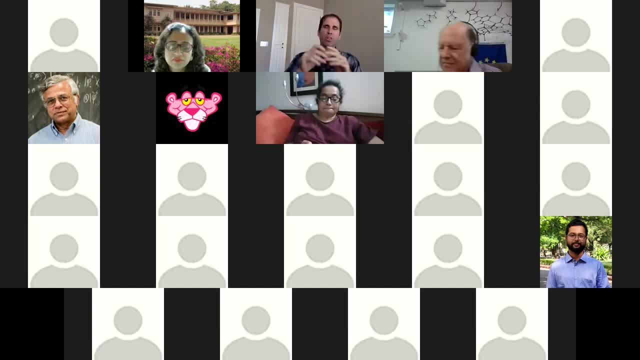 There's also squash entanglement of a channel. that's an upper bound on qkd rates you can achieve over a channel. You know we use that to get bounds to limitations on quantum chain distribution, So I think that could be an interesting topic. Okay so, Charlie —. 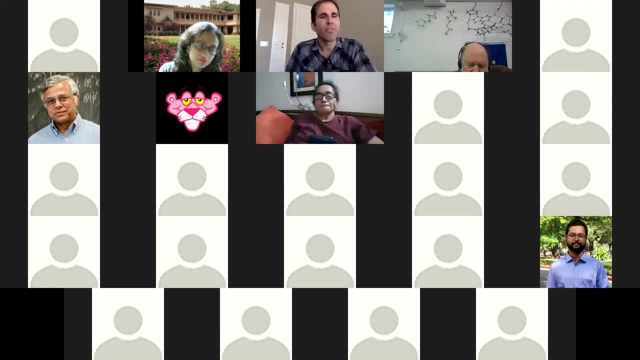 So can I just ask you: so that's squash entanglement. do you mean that work that Andre Winter and his collaborators introduced in 1900? That's right, And that satisfies the additivity condition and those conditions which the additivity. 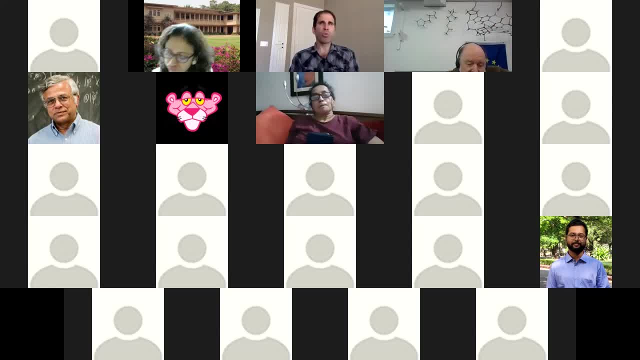 Well, it's actually evaluated for bipartite states. The thing about squash entanglement is it has all these wonderful properties which make it a great. Yes, you mean those additivity properties and the properties like additivity? Yeah, yeah. 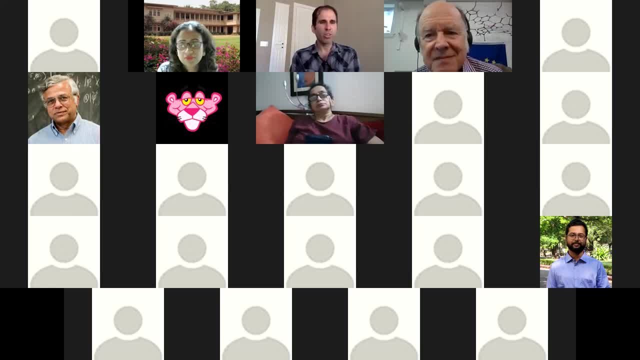 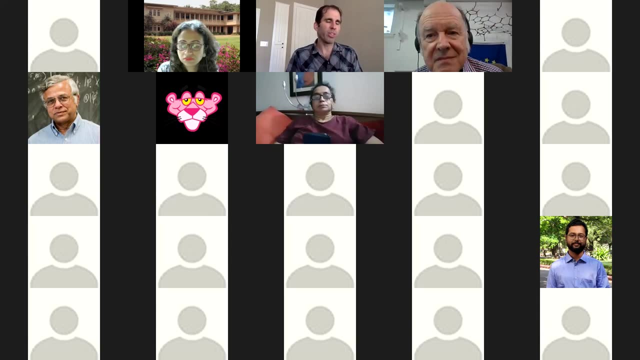 However, to actually compute it for states is a big challenge, And so what you typically do is you, because squash entanglement is an upper bound on distillable key, you just try to figure out a clever upper bound on squash entanglement to bound distillable key. 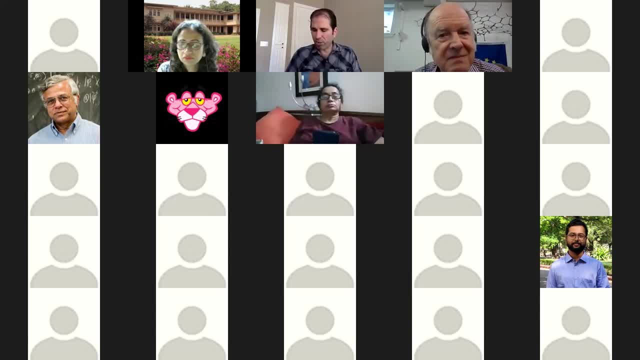 And so that's what's typically done To precisely evaluate. it would be Very interesting. Okay, And another point, you didn't talk about any in the content: the effect of noisy possible channel in another newly emerging application of entanglement, say for random number generation or genuine random number, because entanglement has been applied there. 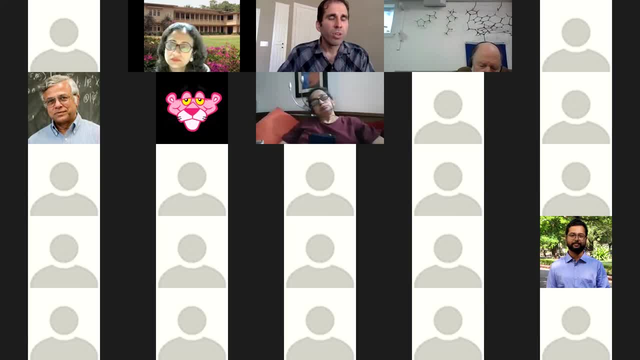 So those kinds of applications, this noisy channel kind of analysis, That's right. So we have. We've worked on that topic. there was a former student- her name is a neat car, I think- she worked with her bossy and her masters. so we wrote a paper where we defined a device independent capacity of a channel that was relevant for device independent. 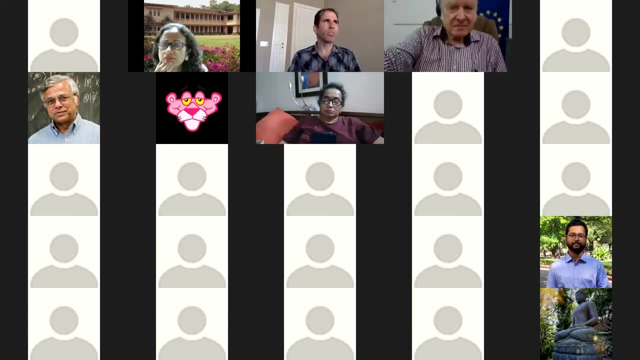 QKB. And then we we use notions related to squash, entanglement, to, to get to, to invent a quantity That is an upper bounds on device independent capacity, with the idea that we want to understand, okay, what are the limits of device independent to get the you know, what are the rates that we can hope to never exceed? and you know, to motivate work on building repeaters for quantity distribution. 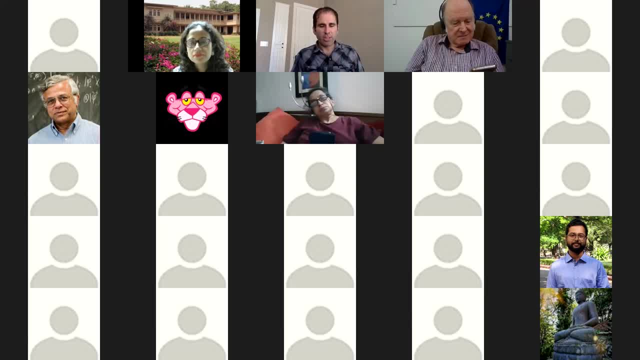 So you know. and then you're asking about random number generation. I believe that these bands can be used Also For to bound the rate at which random numbers can be generated. Okay, Oh, okay. So Charlie made the comments. since Mark has come all the way from the USA to India, it would be a waste of time for him to hurry back home after having stayed only 60 minutes. 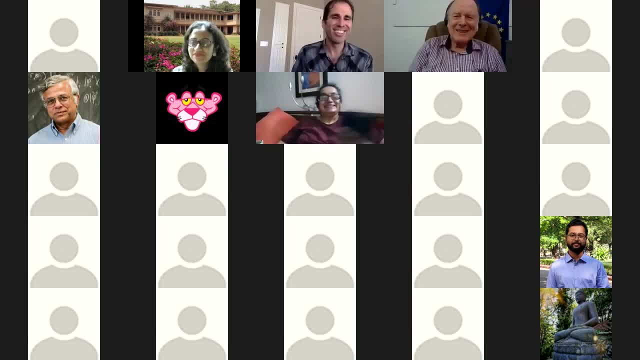 Okay, All right, Charles, and they have an appointment south of the next. All right, Visit. Okay, The conversation is going on. You may have noted from his recital of names that he has important number of Indian students. the US. 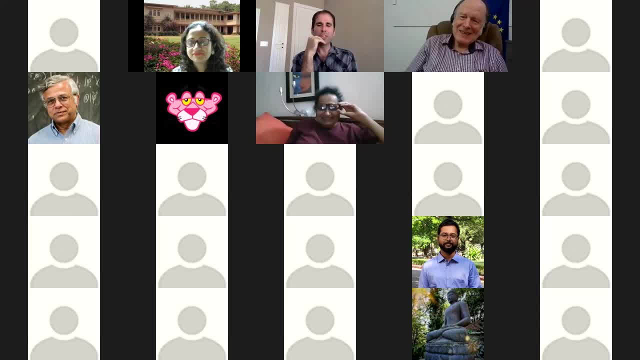 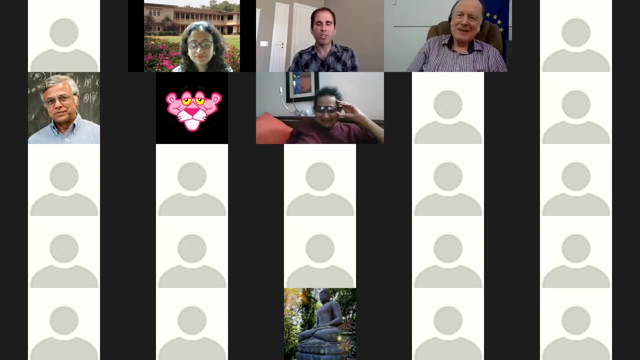 Indeed, that's true. I have been very happy Over- I guess it's now been a decade- to have so many great students come from India to the US and we all get along very well And we're very happy group here, Okay. 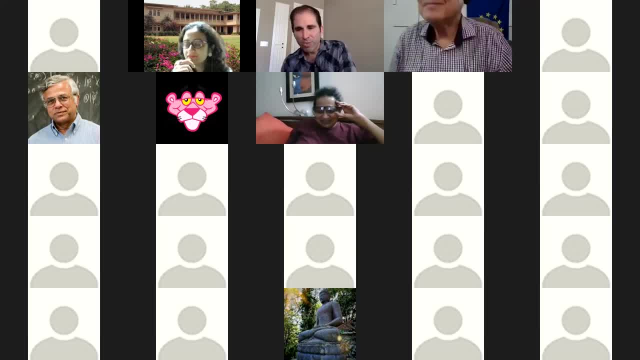 So I hope that you know that continues. So let's go to the next question. So what is squash entanglement? So, in short, you use conditional mutual information, So that's a generalization of mutual information where you take a bipartisan state and find an extension of it where it's a tribe. 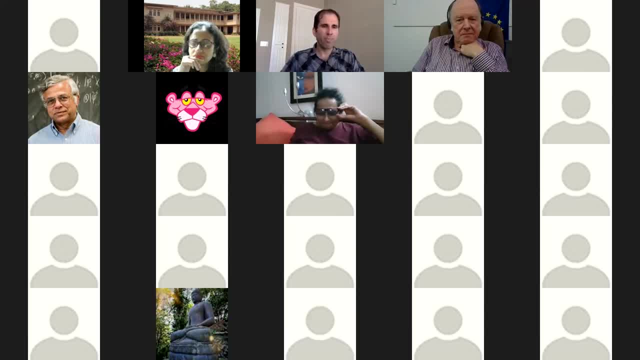 Try parts I extension, you get the extended system to the eavesdropper And then you evaluate the conditional reach information of A and B given E. So it's like the correlations that Alice and Bob have from the perspective of E, And then what you do is an optimization. 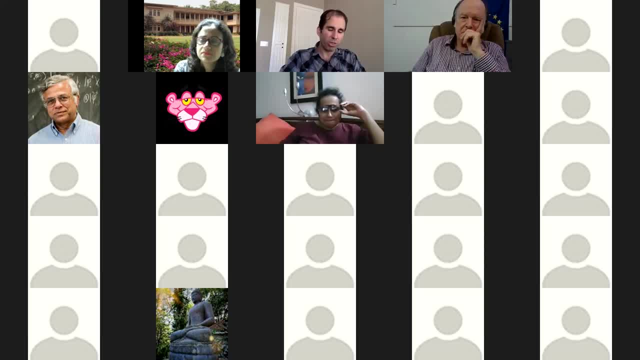 You minimize over all. you minimize the conditional reach information over all these extension systems And that minimization is, as far as we know, unbounded And that's why it's hard to compute in general And it could possibly be an uncomputable measure. 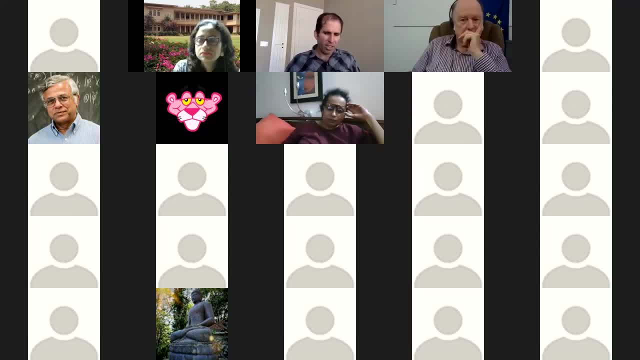 You know- that's what people have thought for at least a decade- that when you see this regularized quantity, that regularized quantity taken in optimization over an unbounded extension system, it's possible that the quantity could be uncomputable. you know. 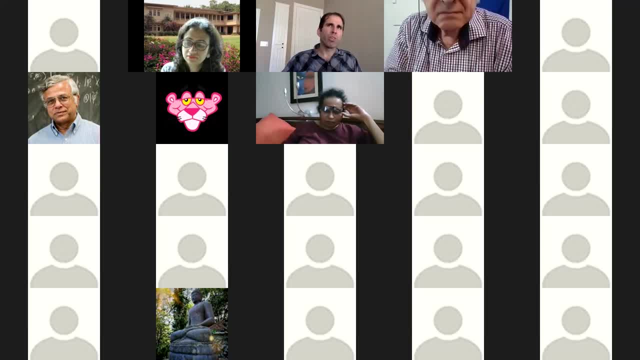 So even though theoretically we can prove that squash entanglement has all these nice properties, like it's kind of an ideal entanglement measure, in that sense it's unideal in that we can actually compute it. So that's why I think there could be. 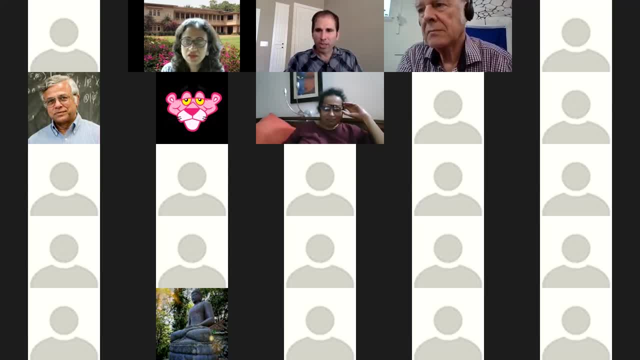 more interesting work there. Okay, so I like Charlie's comment. Mark's skepticism about causal order is like mine about closed time, like curves as a cryptanalytic or computational aid. um, yeah, indeed, uh, that's. that's a, you know, interesting research line that has been done about closed. 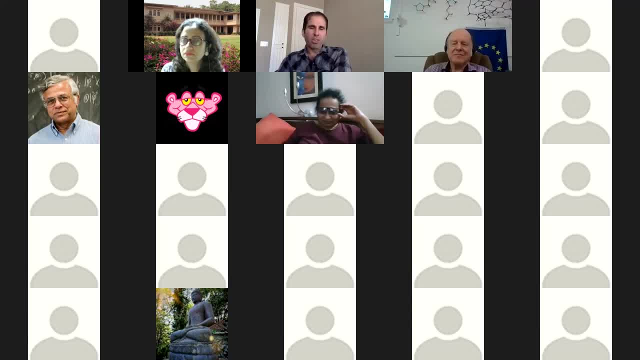 time, like curves. there are different models that have appeared and, uh, they're very intriguing, but, um, they all involve non-linear modifications of quantum mechanics and so, um, you know, they- they kind of everything's just much more challenging to deal with. and then there are kind of different. 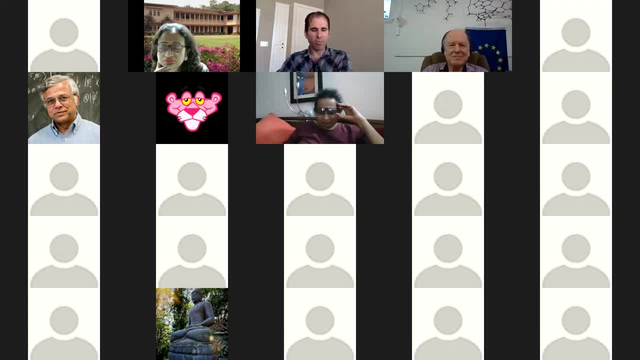 interpretations of what goes on. you know, there was a, um, i believe, in scott aronson's book quantum computing, since democratus. he has a chapter called the ctc wars or something like that, and it's about uh, different interpretations on, uh, what, what is possible with close, like time, like curves. so 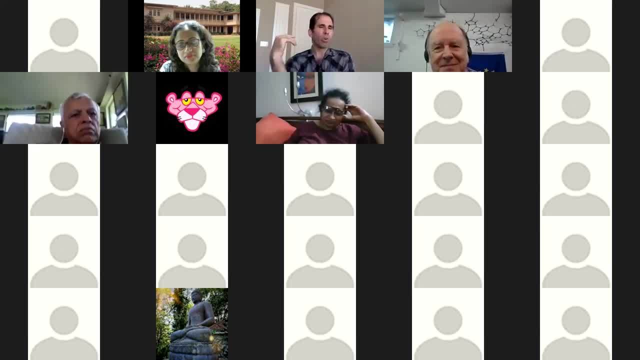 scott aronson and john watrous wrote a paper that quantum computers supplemented with closed time, like curves, could achieve, uh, piece-based computations, you know so, like computations where there's um, you're allowed a polynomial amount of memory, and it's a very powerful computational class. however, uh, charlie and collaborators, 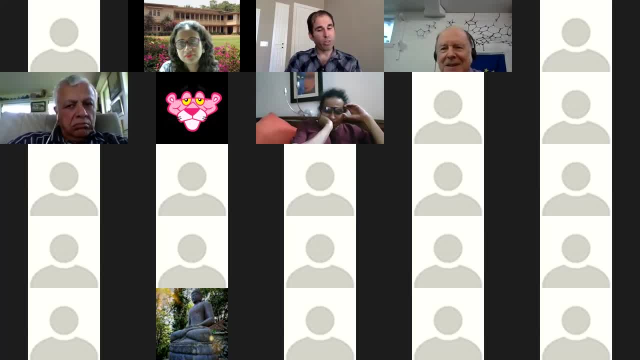 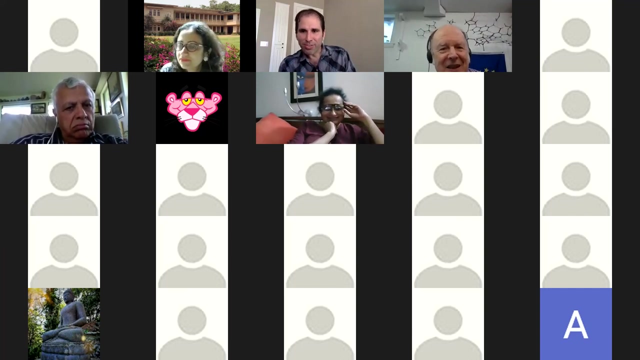 wrote a paper where they they wrote that there's actually no advantage at all offered by these. uh, closed time occurred. they behave according to the model of deutsch and um. i don't think this is resolved. it's like that's why it's a war, um, so okay, yeah, so i don't think we have any more. 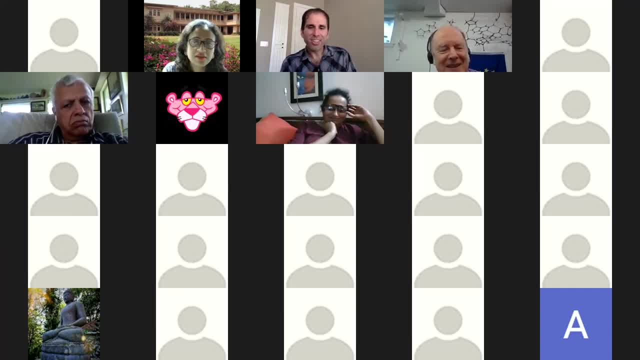 questions mark. so, um, if anyone wants to say anything at this point, then please unmute. yeah, i think mark said he has to leave in a minute. yeah, i'm going to need the. the dowlings are here, okay, yes, of course. yeah, i, i didn't catch that on.